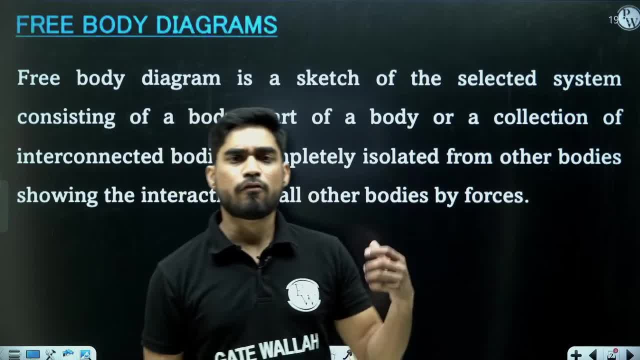 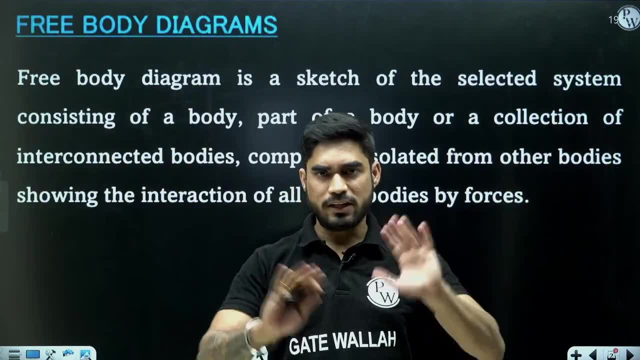 through the free body diagram. So what are free body diagrams? Free body diagrams are through forces. So basically, if you want to analyze the forces of a body, then you isolate that body from all the other bodies. whatever connection they have, you disconnect them. 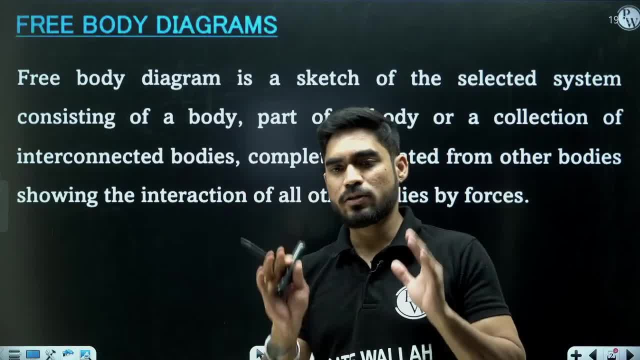 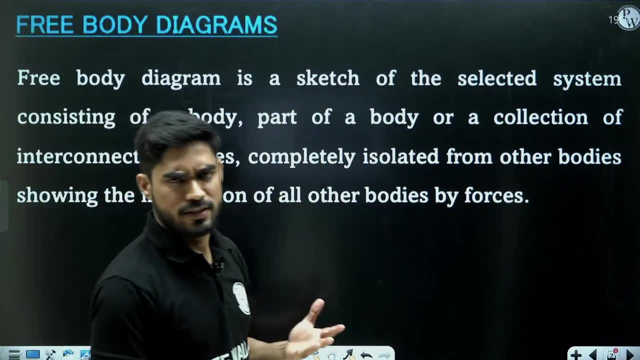 you isolate the body And when you disconnect the body from other bodies, you need to show the connection between them, the interaction between them through forces. We saw some good examples of free body diagrams yesterday And I told you about the reactions due to. 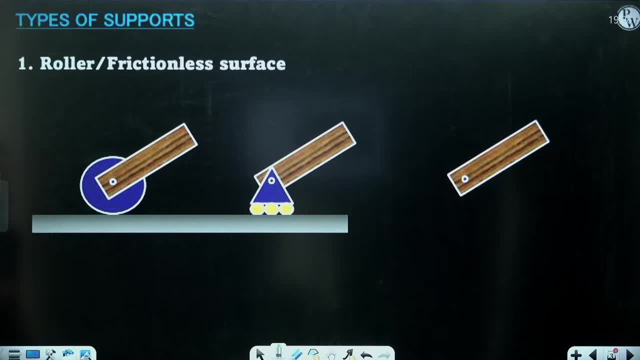 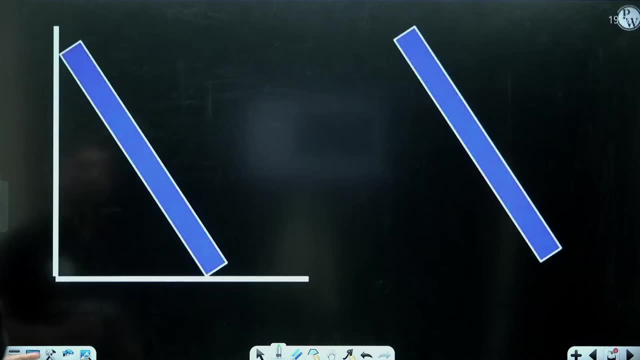 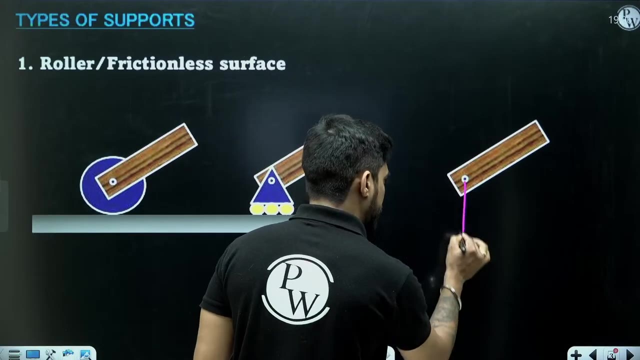 each type of support. There are three categories of support: roller or frictionless surface, hinge support or friction surface and fixed support. In case of the first category means roller support. you get one reaction which is normal to the surface of the roller. Yes, 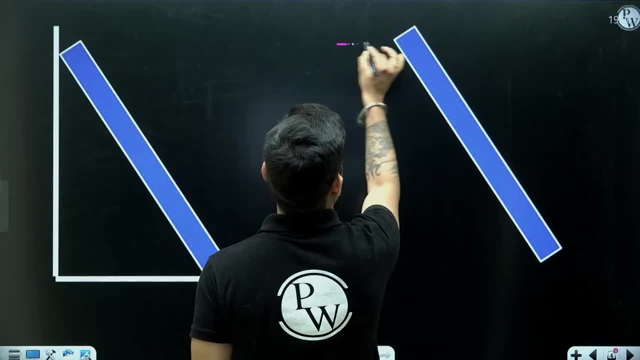 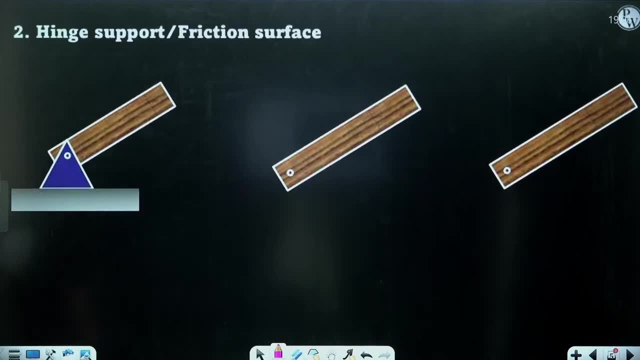 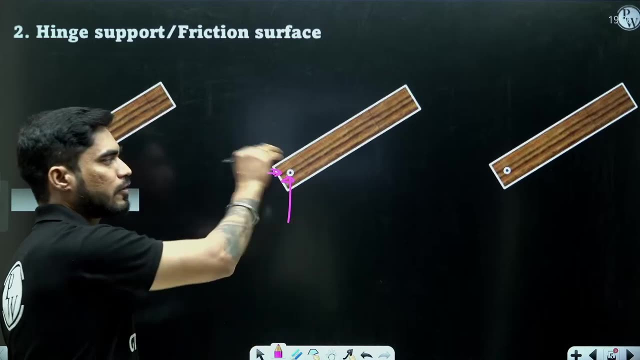 same goes with the friction surface- also frictionless surface also- you get one normal force perpendicular to the surface. In case of hinge support, also known as spin support, you get two reactions. But in some cases, instead of drawing these two reactions, we show the resultant of both and we only 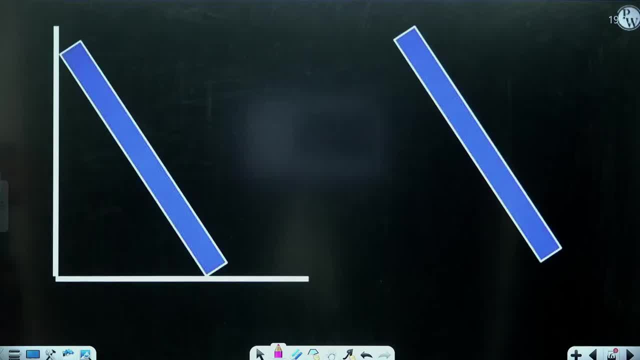 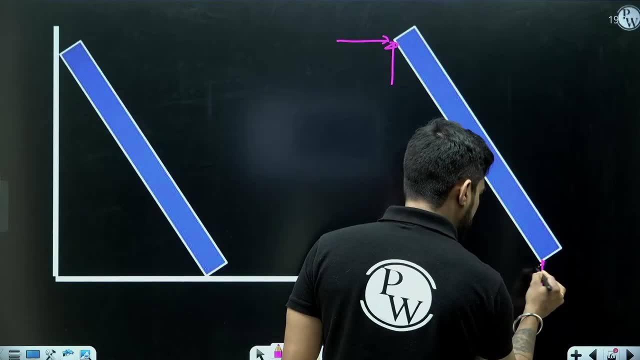 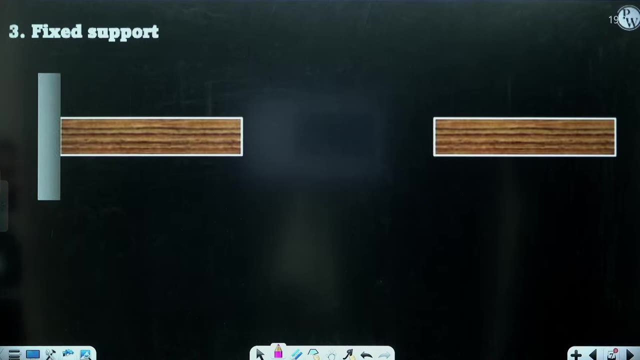 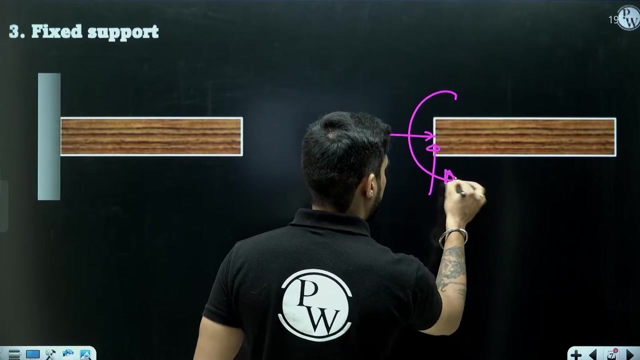 get a single reaction. Same goes with friction surface, also At the point of contact. you get two forces right like this, And the last one was the fixed support. In this case you get three reactions: one in X, one in Y, and you also get a couple. Why are you getting a couple here? Why not couple? 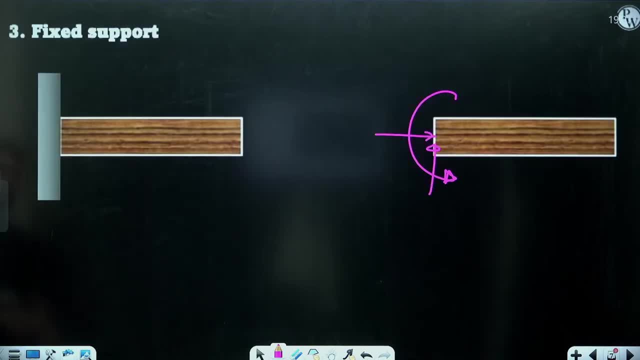 in other cases, Because you get a couple if the constraint is if the rotation of the body is also constrained. And here, as the body is fixed, the rotation of the body is constrained, So you are getting a couple. In other cases the rotation is not constrained. 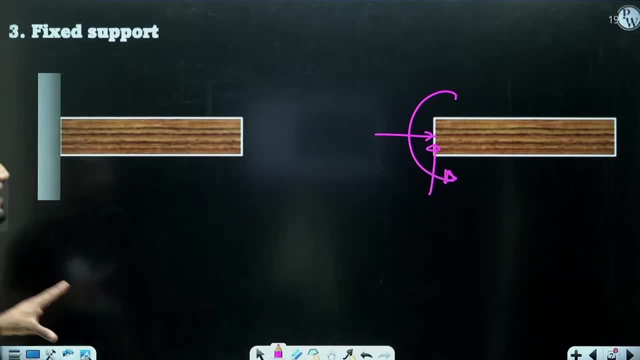 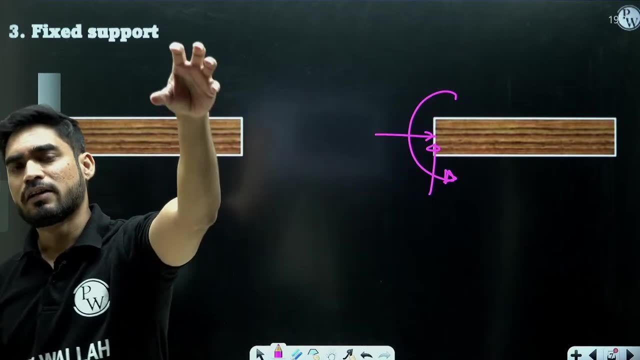 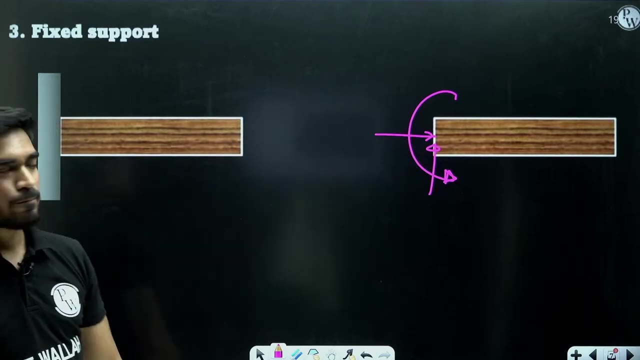 So you were not getting a couple. So these were the three categories of supports. So whatever subtype of support the body has in real life when we solve the problem in engineering mechanics, we will consider either one of these three supports. And now, in today's 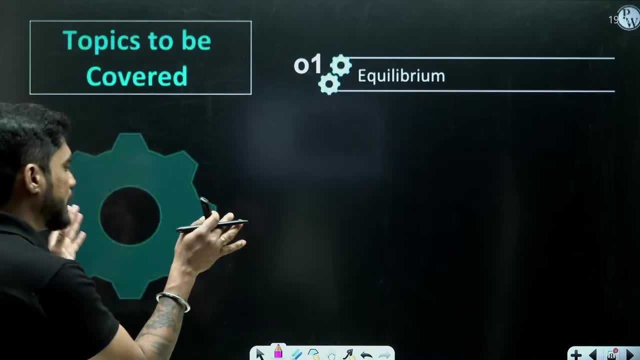 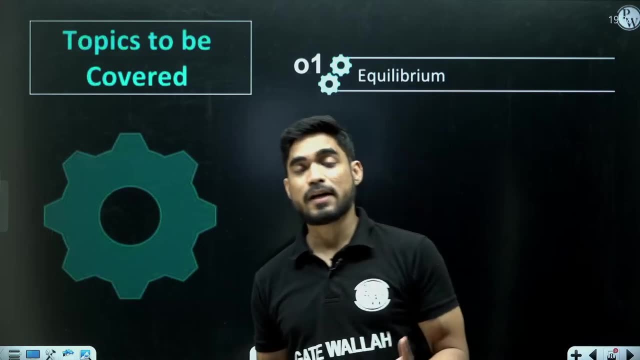 class. we are going to start with equilibrium. See the entire structure. in this situation you are getting a couple, But in this case you are getting a couple Because you are getting entire statics part is based on the concept of equilibrium, okay, So we need to first. 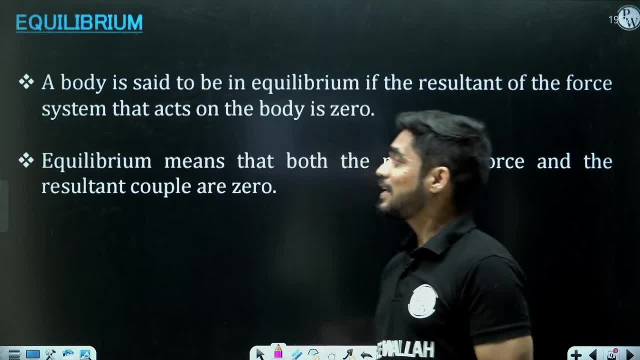 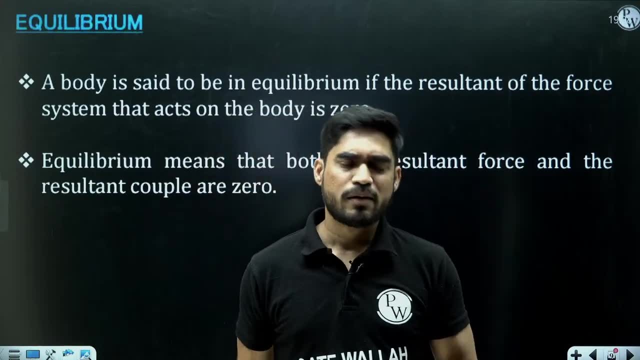 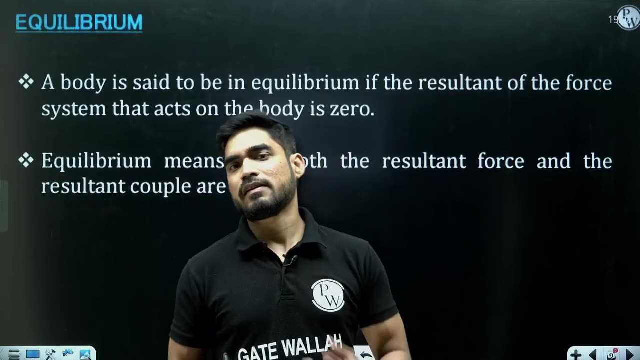 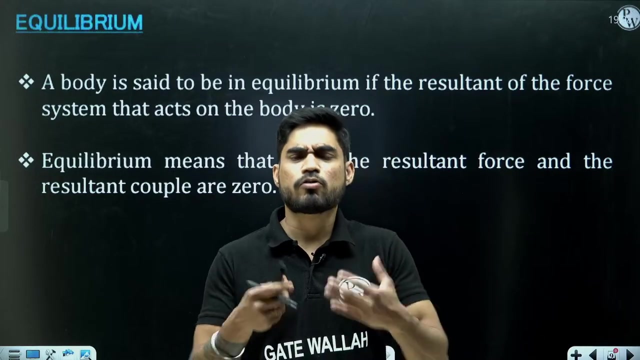 understand what do we mean by equilibrium. So let us understand about equilibrium. See, you might have heard this term in different subjects, because equilibrium in different context has different meaning. For example, when you study thermodynamics, then there is a term called thermal equilibrium, right? What do we mean by thermal equilibrium? If the temperature 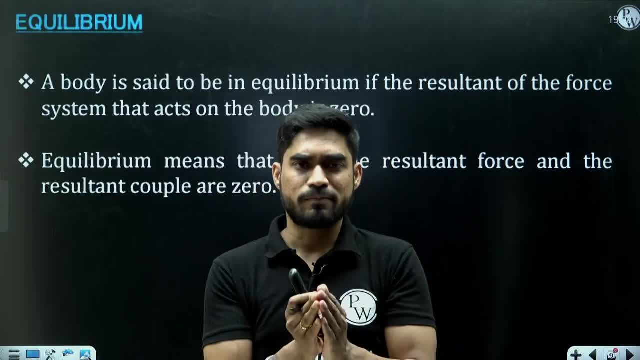 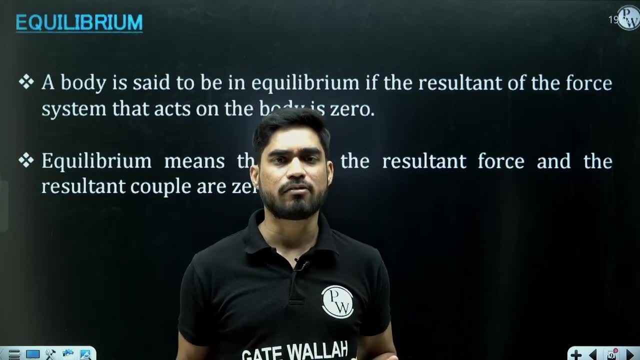 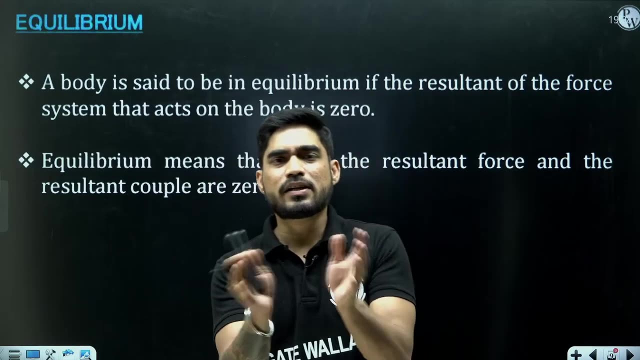 of the two bodies is exactly same. there is no heat interaction between the two bodies. we call that. we call them to be in thermal equilibrium. right Then in chemistry you might have heard about chemical equilibrium. When there is no reaction happening, you call the bodies to. 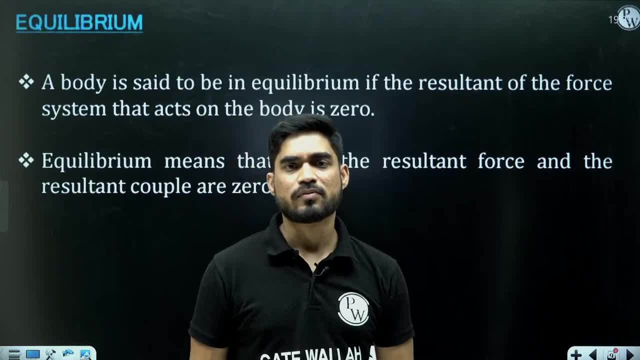 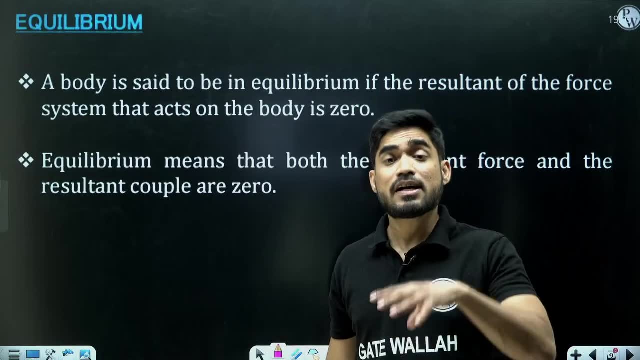 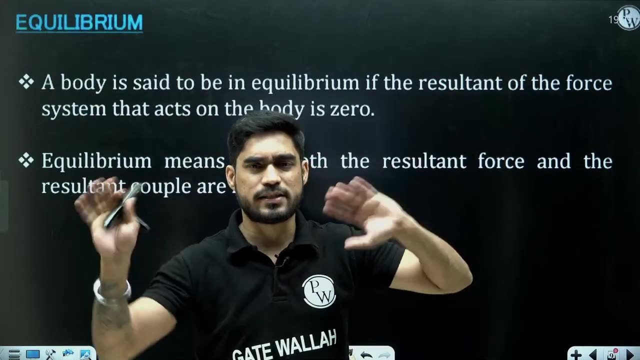 be. you call the chemicals to be In chemical equilibrium. So there are different types of equilibrium, But here we are going to talk about mechanical equilibrium. Here we are going to talk about the equilibrium in the context of forces. So when a body is subjected to different forces moments, then what will be? 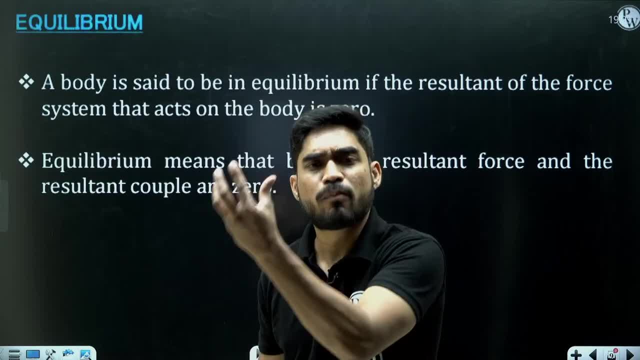 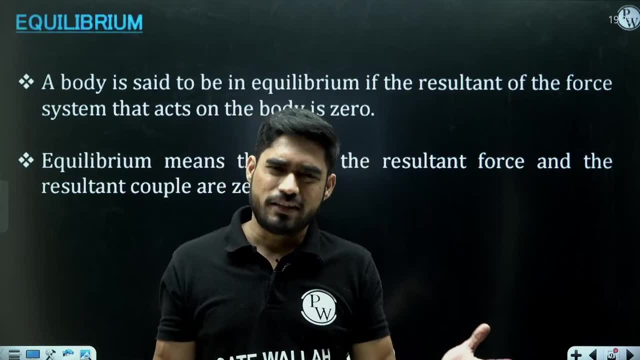 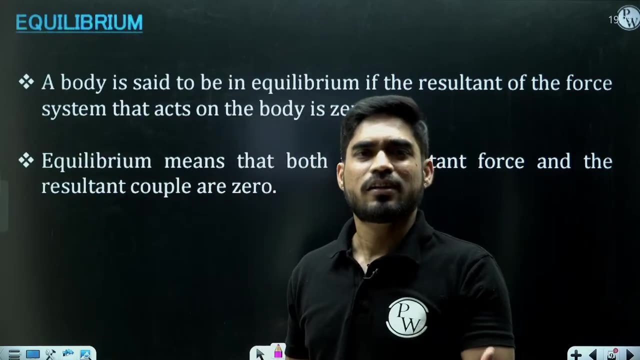 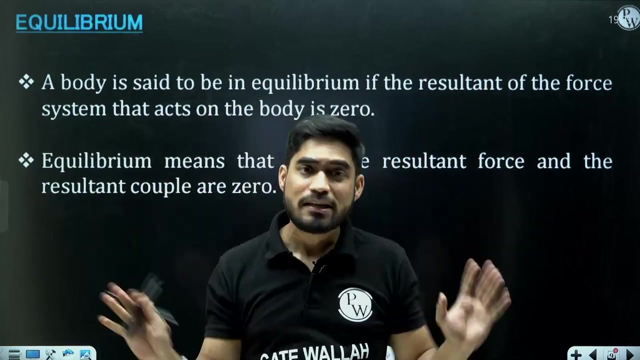 the condition of equilibrium. When do we say that the body is in equilibrium? In general, you can say: equilibrium means equality, Because the term itself is derived from this word. only right, Equality, Equal. So what does this mean? When all the forces acting on the body becomes equal, they are going to cancel each. 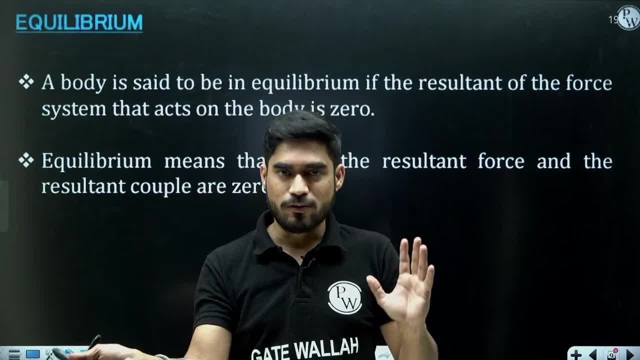 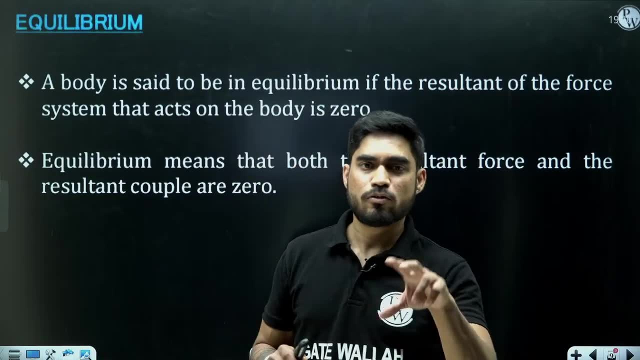 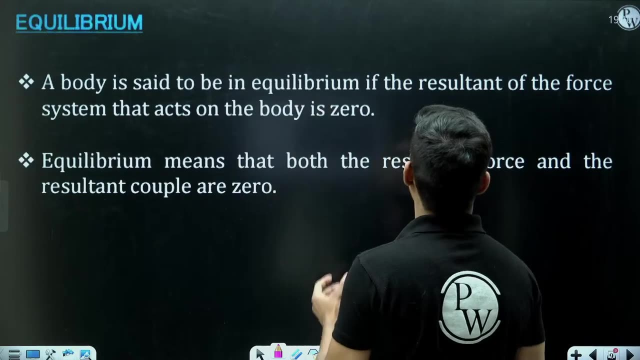 other And the net force will become zero. This is a very generalized statement, Exactly in technical statement. if I have to tell you what is equilibrium- mechanical equilibrium, equilibrium related to forces- then a body is said to be in equilibrium if the resultant of the 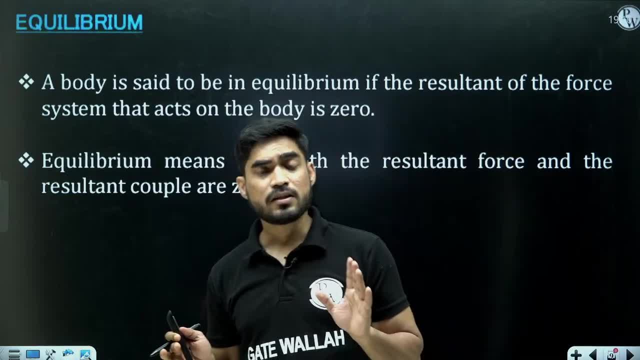 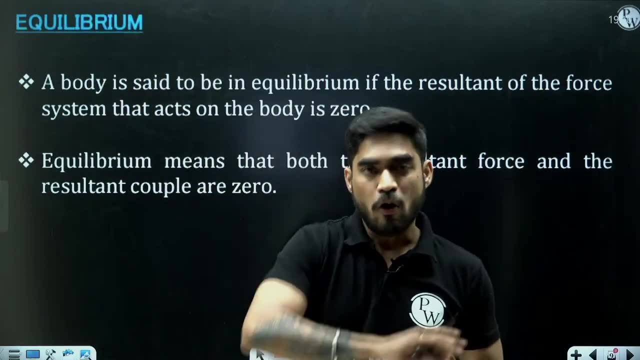 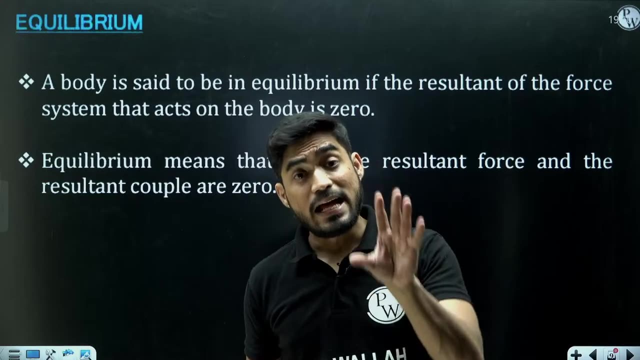 force system is zero. See, the body is subjected to multiple forces: Three, four, five, maybe ten forces. All these forces collectively are known as force system, And this force system will have a resultant. We have already seen how to find resultant of different force systems, So we are going to. 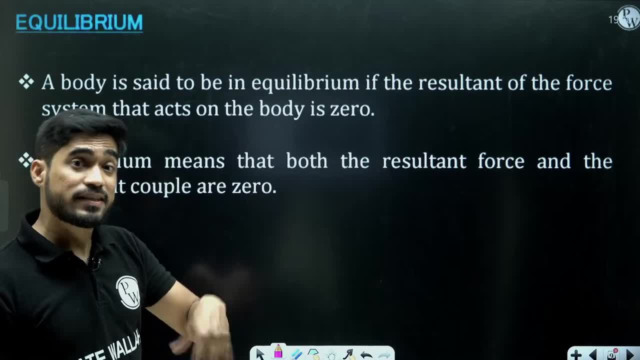 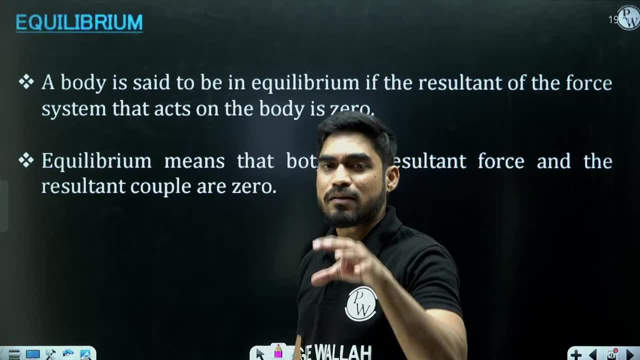 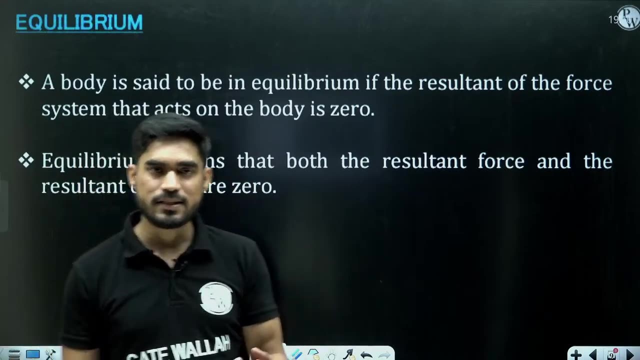 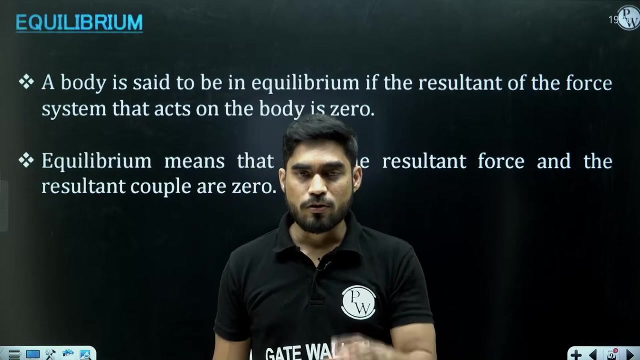 explain these functions. Now, if this resultant is zero, it means the body is in equilibrium. Now the resultant can be a single force or a force and a couple. We have seen in some cases we get a couple also. Apart from the force, we also get a couple. So if the resultant is: 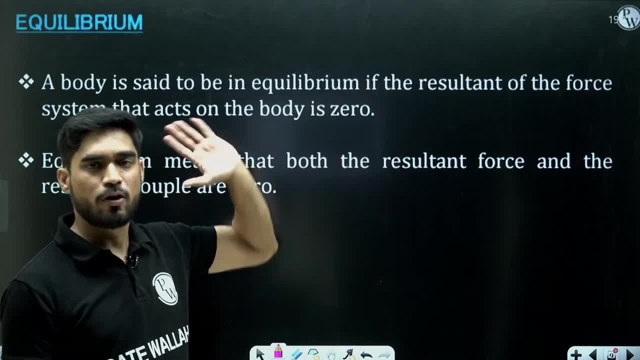 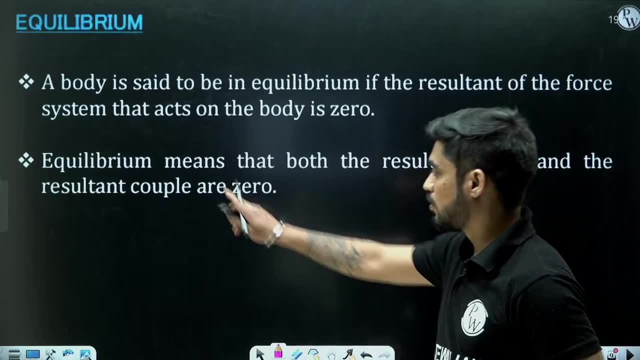 only a force, then that force will be zero. If the body is in equilibrium, the body will be in, and if the resultant consists of the force as well as the couple, then both will be 0.. Look at this: Equilibrium means both the resultant force and the. 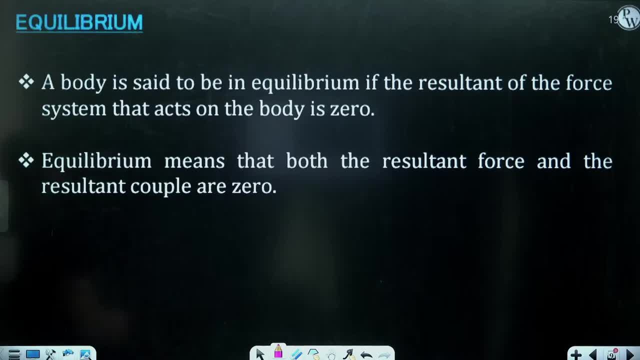 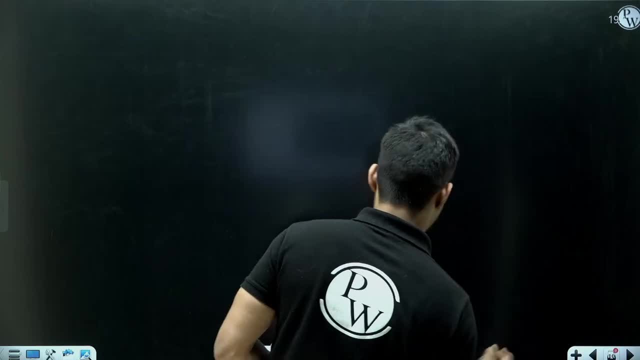 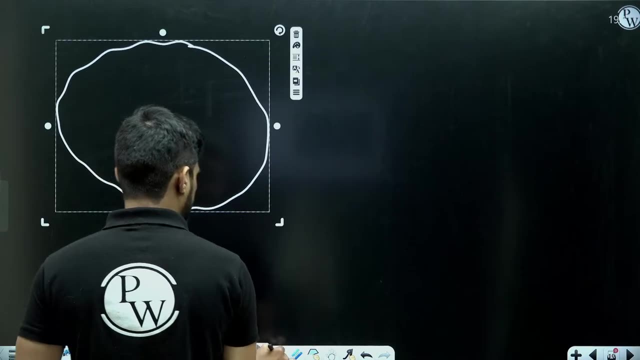 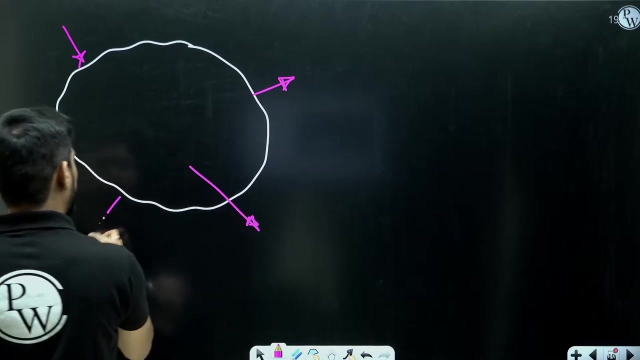 resultant couple are 0.. So let's say we have a body which is subjected to three-dimensional forces. Ok, This body is subjected to what Three-dimensional forces? Right now I can't show you the third dimension. Just assume that this body is subjected to. 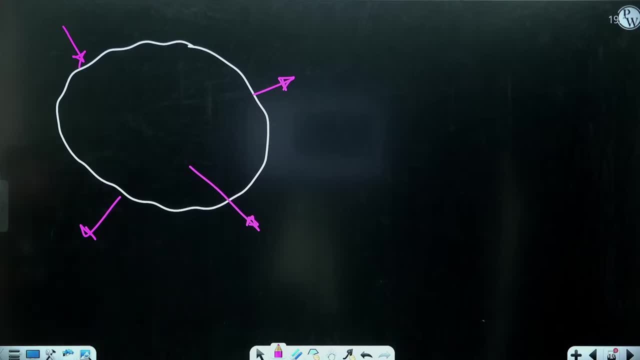 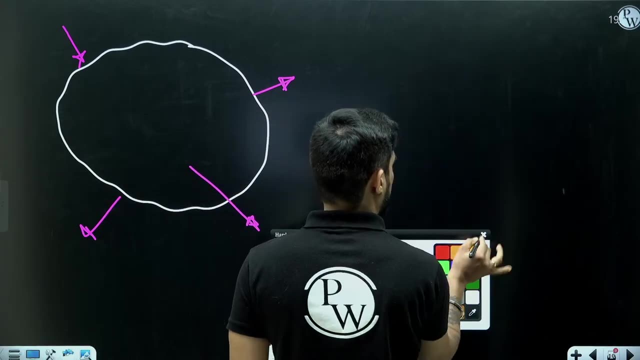 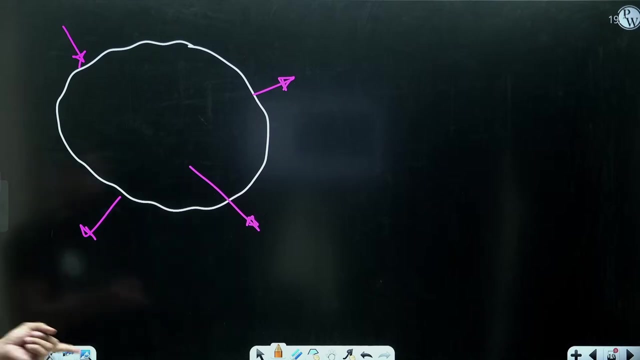 three-dimensional forces as well as couples. Now the resultant is 0.. Right, The resultant force and the couple are 0. So if the resultant force is 0, it means the component of the forces. the component of the resultants will also. 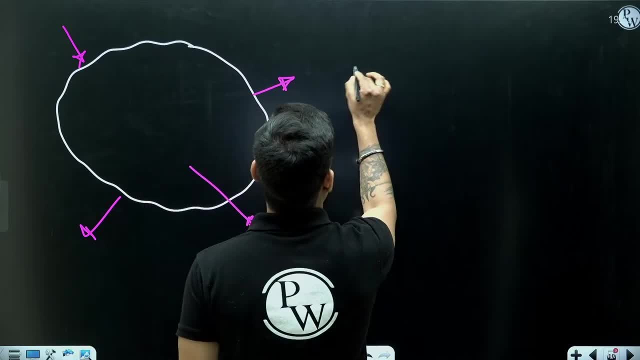 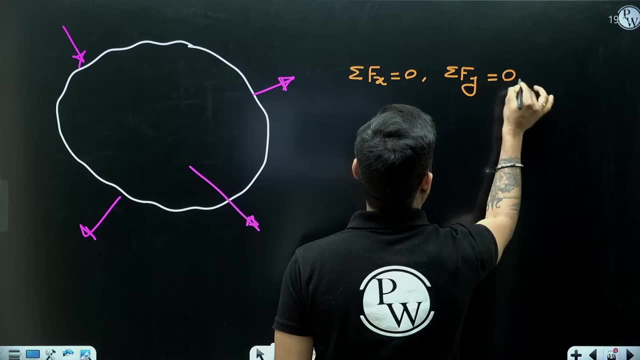 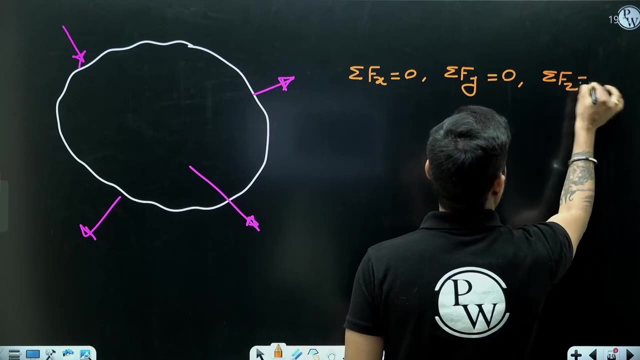 be 0. So it means summation of Fx will be 0, summation of Fy will be 0, as well as summation of Fz will be 0. See, the resultant force is also three-dimensional, I am assuming, right. 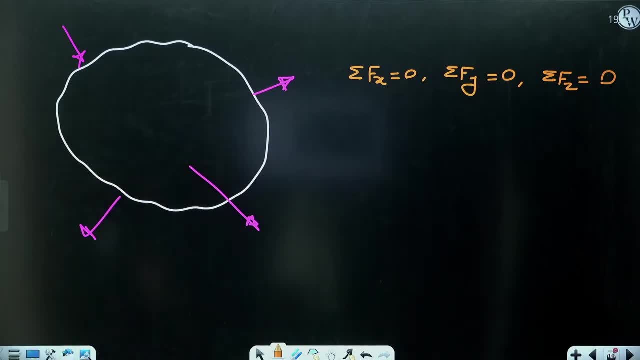 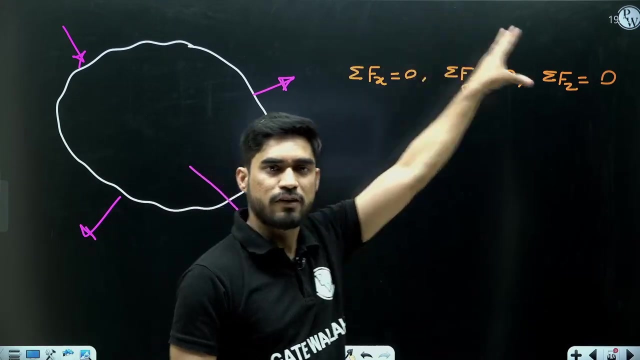 now that the body is subjected to three-dimensional forces, So the resultant will also be three-dimensional. Yes, Right, So it will have three different components. So if I resolve the resultant, I will get three components. summation of Fx. summation of Fy. 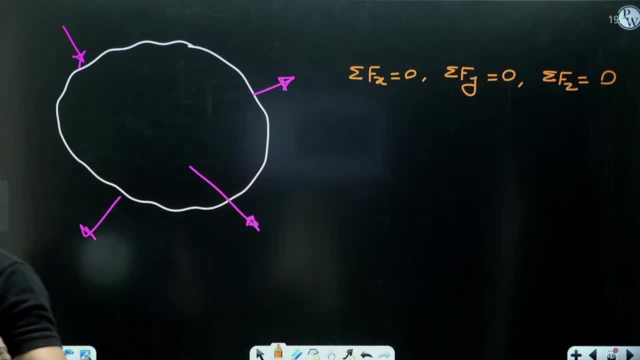 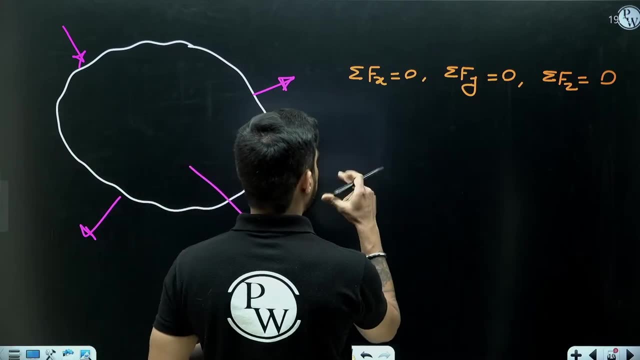 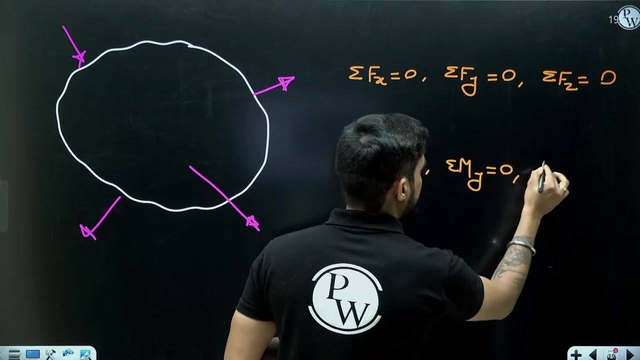 summation of Fz, and if the resultant itself is 0, the components will also be 0. Similarly, if I resolve the couple also, I will get three components of couple: summation of MX, summation of MY summation of Mz. So these are also北. 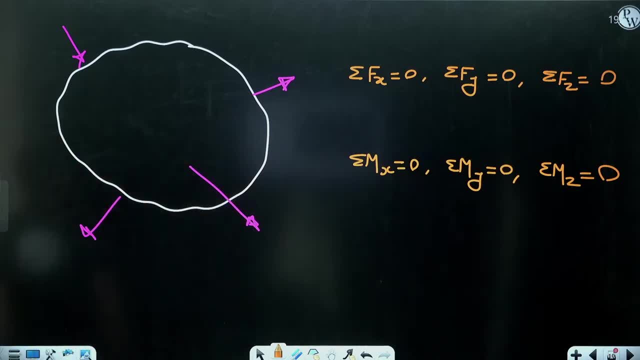 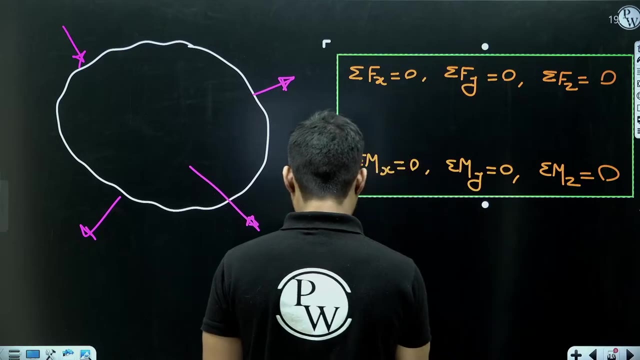 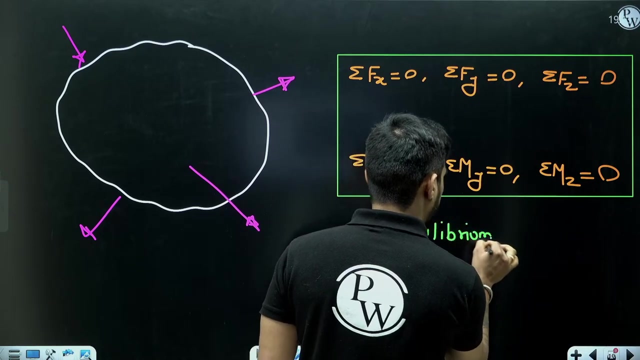 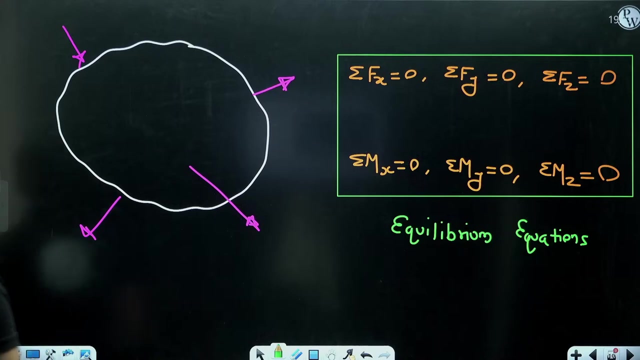 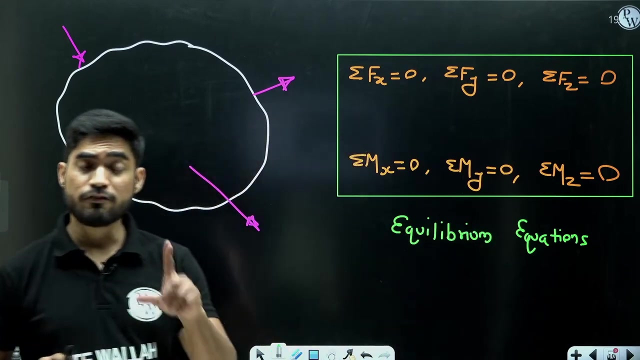 equal to 0.. So we have these six mathematical relations. These mathematical relations collectively are known as equilibrium equations. What do we mean by equilibrium equations? Understand very important Equilibrium equations are the necessary conditions to be fulfilled if the body is in equilibrium. If the body is in equilibrium, it means these: 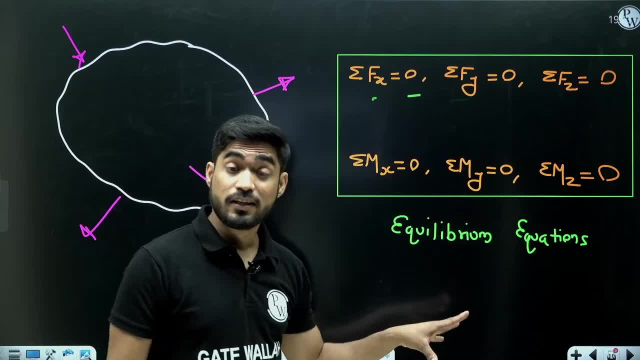 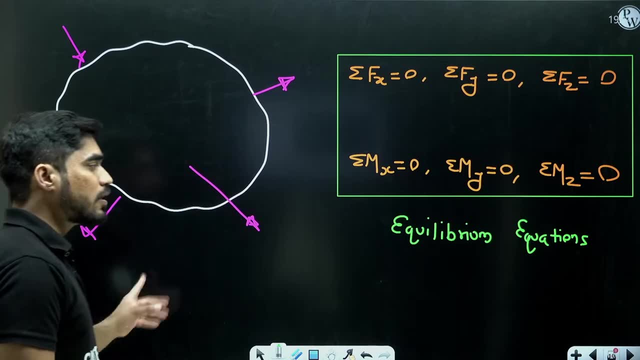 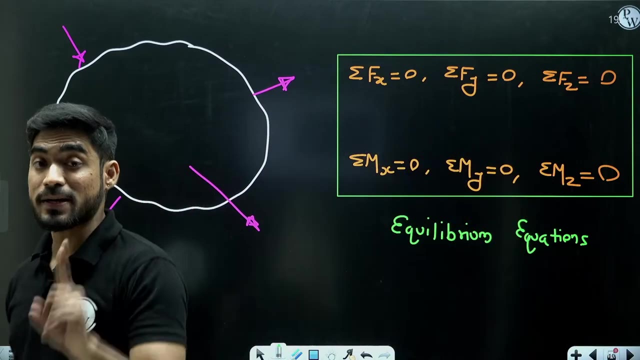 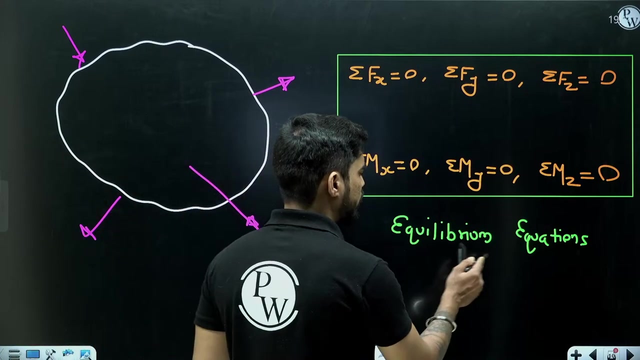 six equations must be satisfied. If any one of these equations are not satisfied, the body will not be in equilibrium. So these are the necessary conditions which must be satisfied. Now why are we studying about equilibrium? A关 These equations must be satisfied, but what we will get A關 By satisfying them? 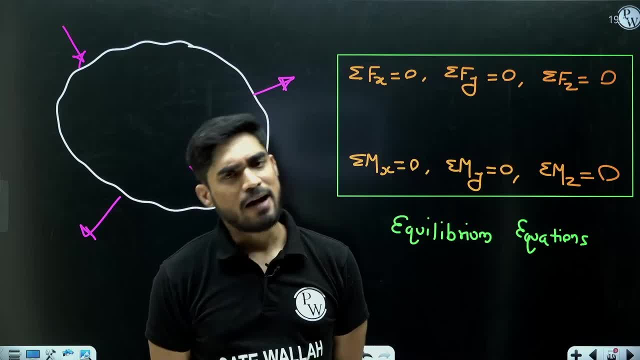 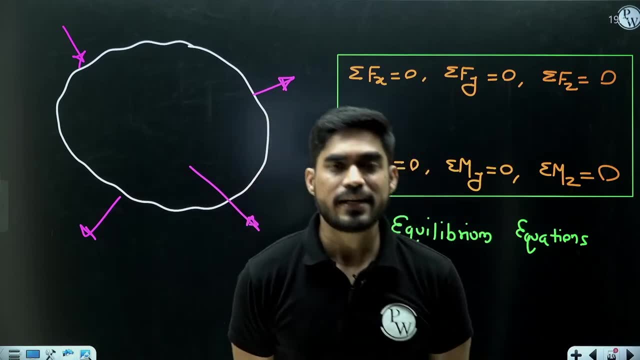 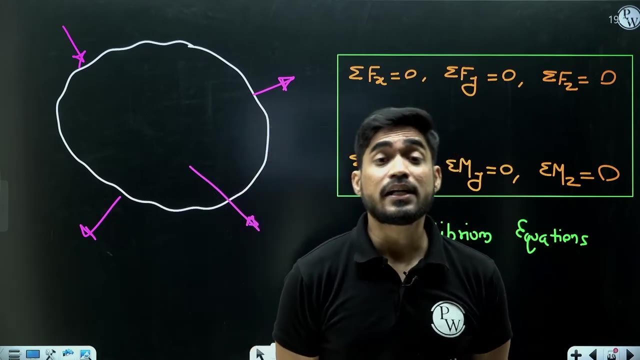 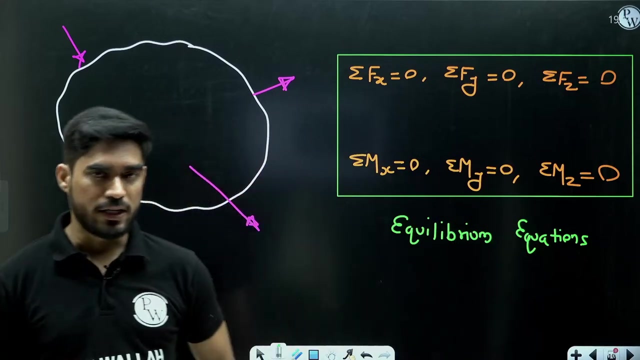 If we already know that a body is in equilibrium, why will we write these equations? A关 Understand this Experience. 10 дело 단 t. These equations, these mathematical equations, are used to calculate the unknown forces acting on a body. When you draw the free body diagram of a body, there are some forces that are known to you. 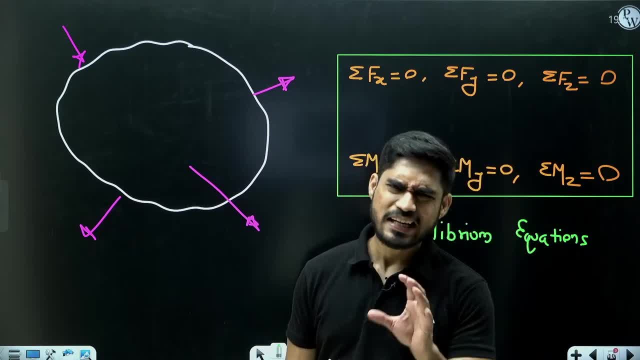 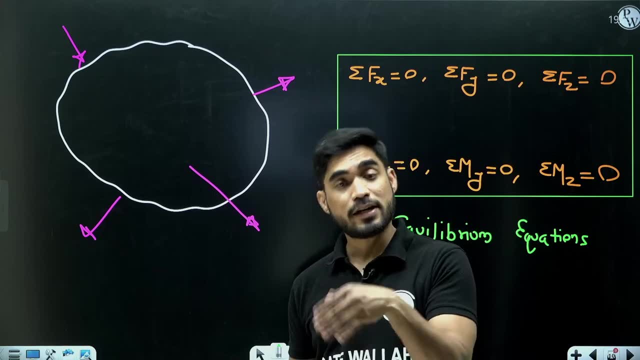 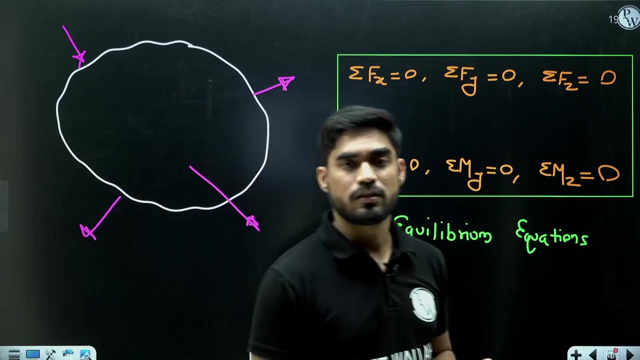 For example, weight of the body. that is known to you, But there are some forces which are unknown to you, For example, reaction forces due to supports. This is not known to you. This is an unknown force. So whenever you draw free body diagram of a body, there are some forces that 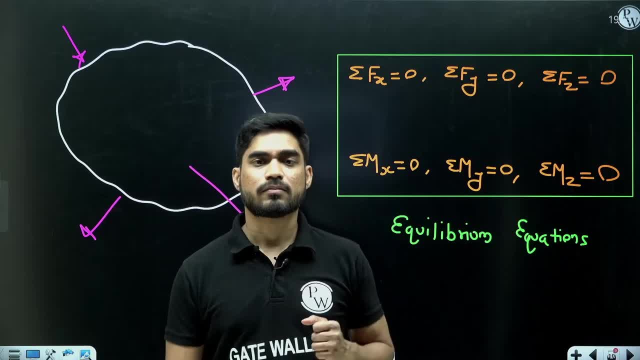 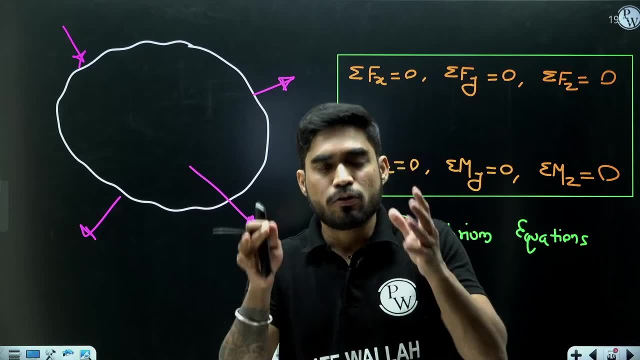 are known and there are some forces that are unknown. These unknown forces have to be calculated. Then only you will be able to design the body. In order to calculate these unknown forces and to calculate the free body diagram of body, you need to know the force acting on the body. 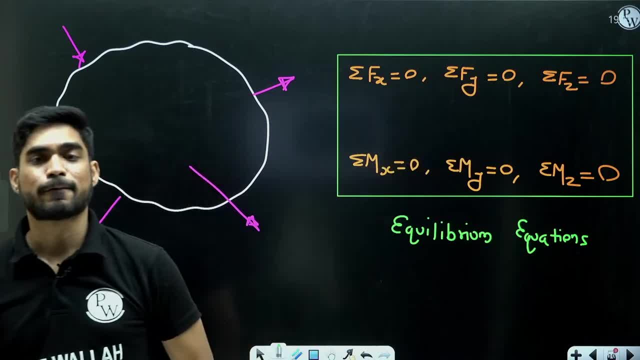 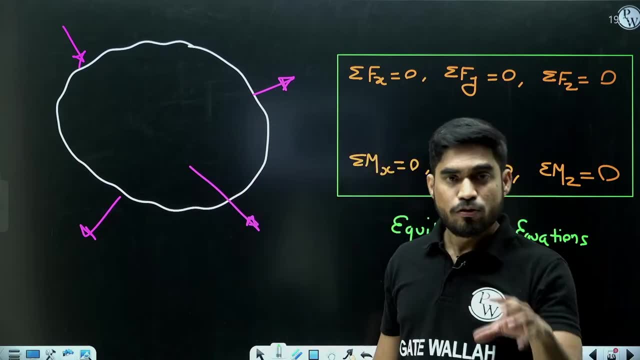 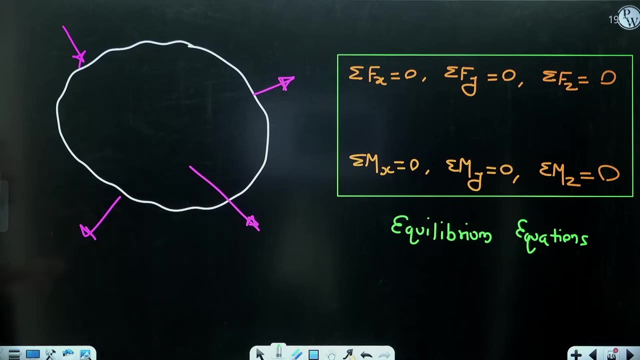 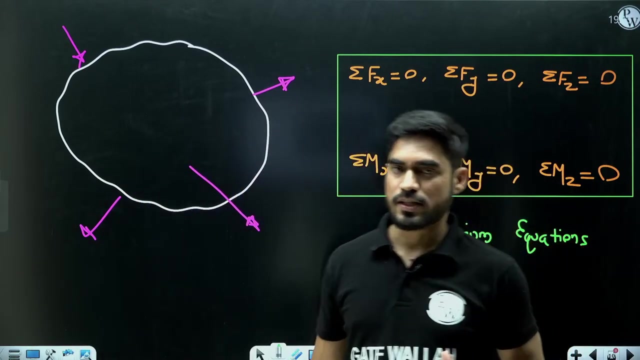 forces, we will use these mathematical equations. So these mathematical equations are used to calculate the unknown forces acting on a body. So what we are going to do is, whenever you have a question where the body is in equilibrium and you have to calculate some unknown forces, 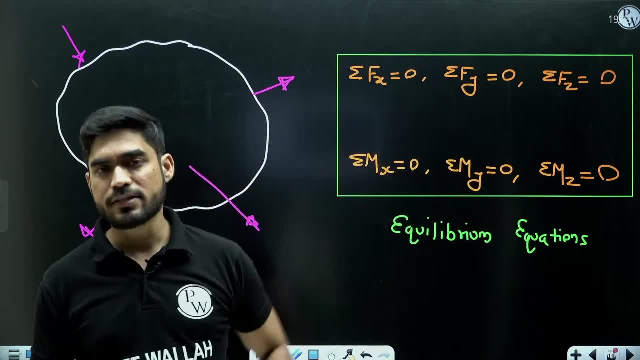 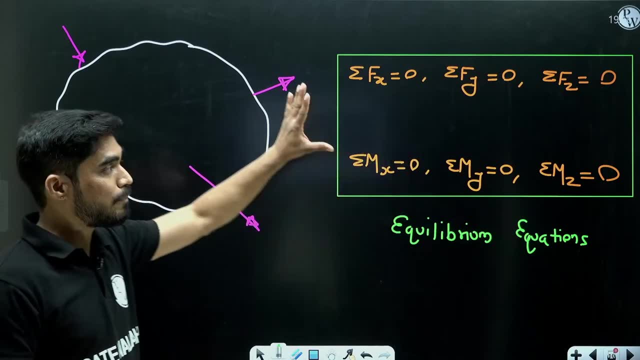 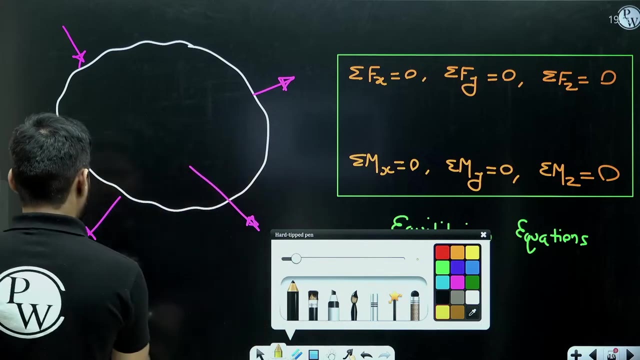 you will draw the free body diagram of the body first, because without drawing the free body diagram, we will not be able to apply these equations. In order to apply these equations, you have to have the free body diagram. What is this? This is free body diagram, So we can only 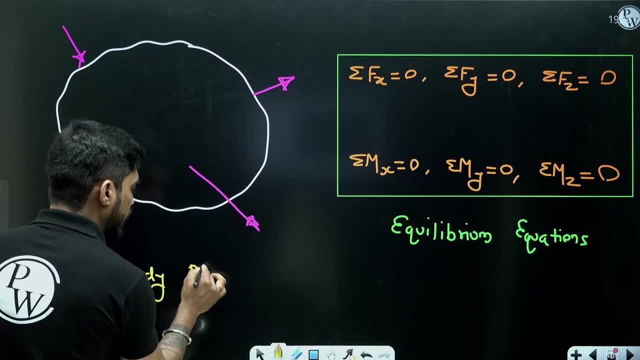 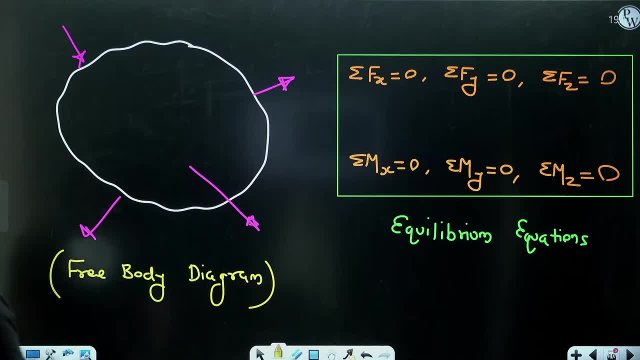 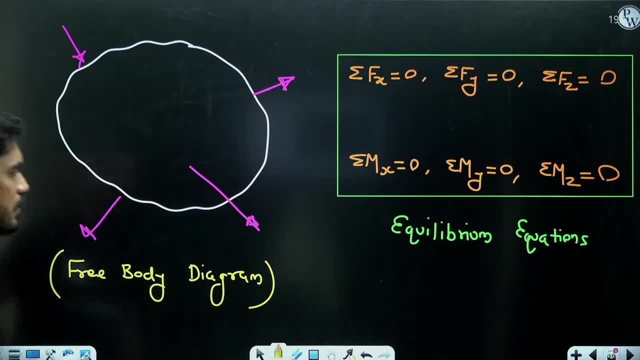 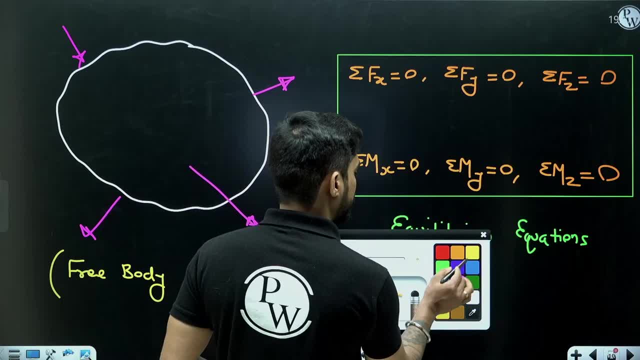 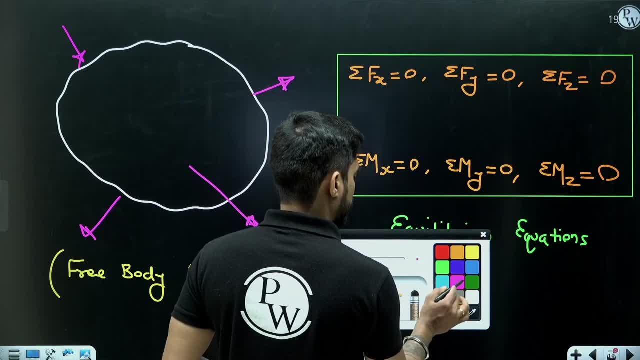 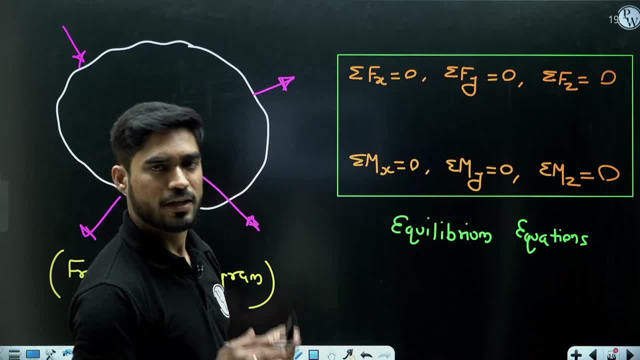 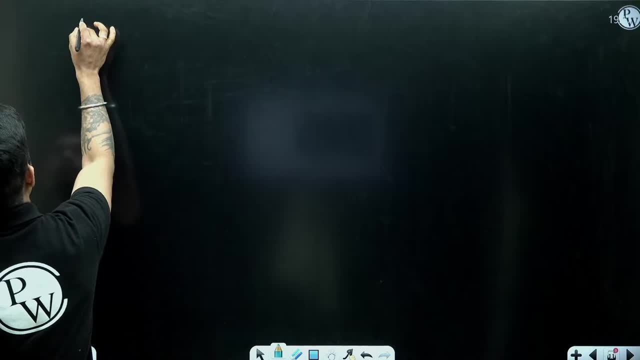 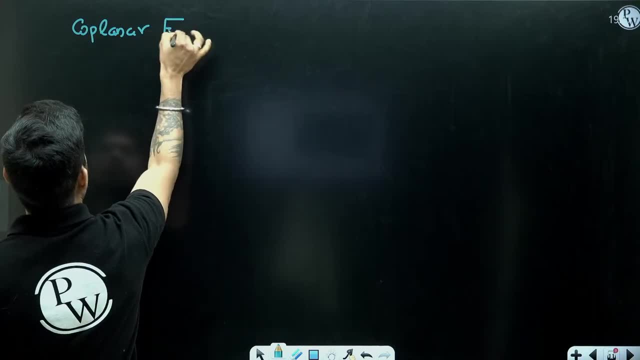 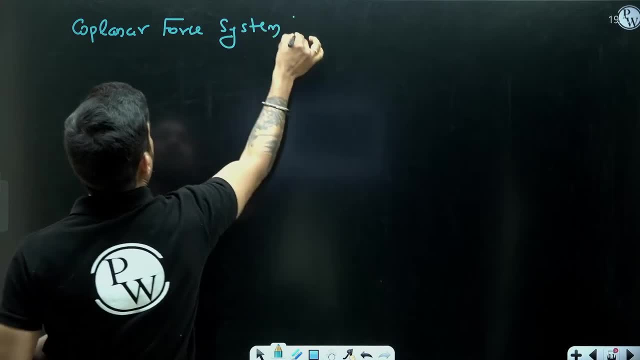 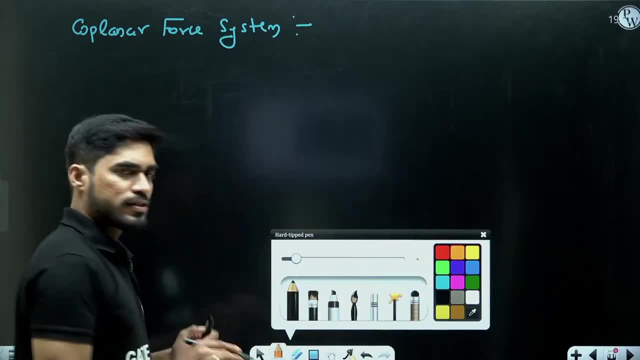 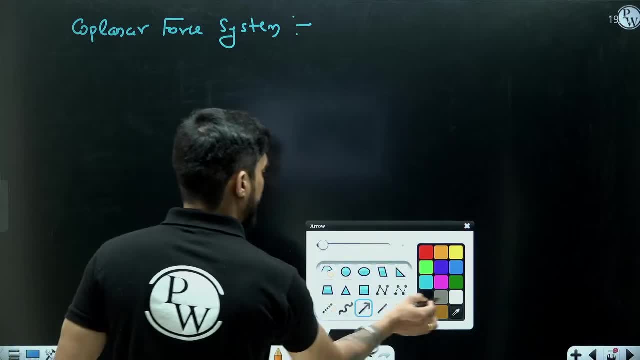 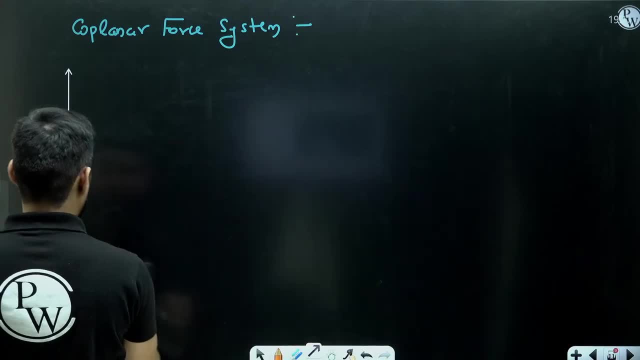 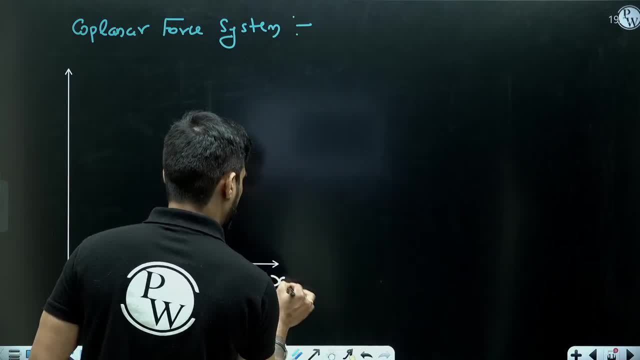 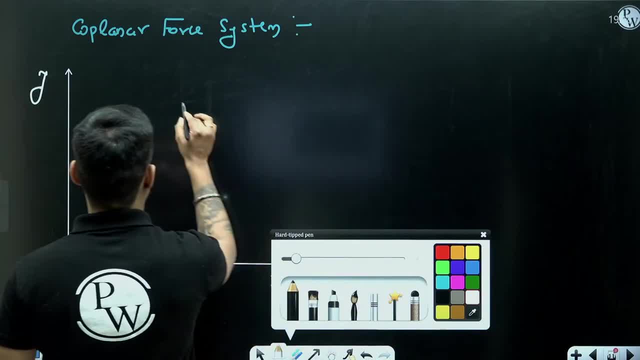 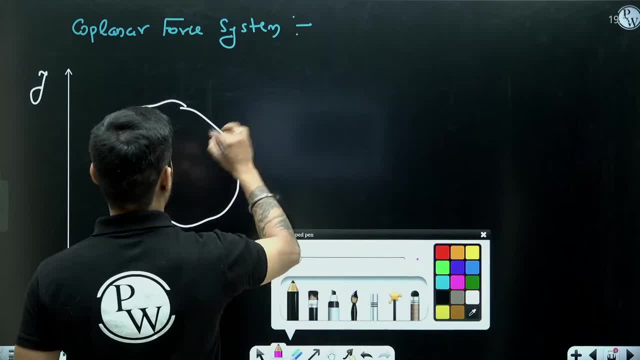 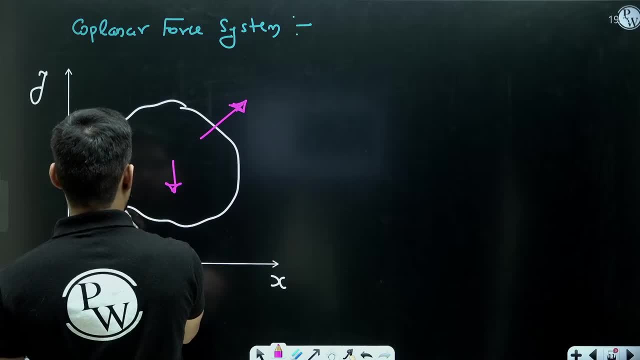 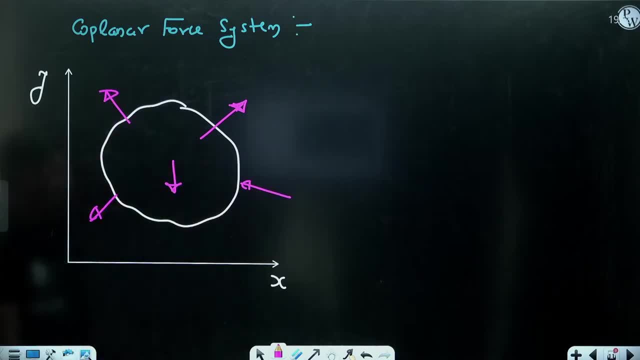 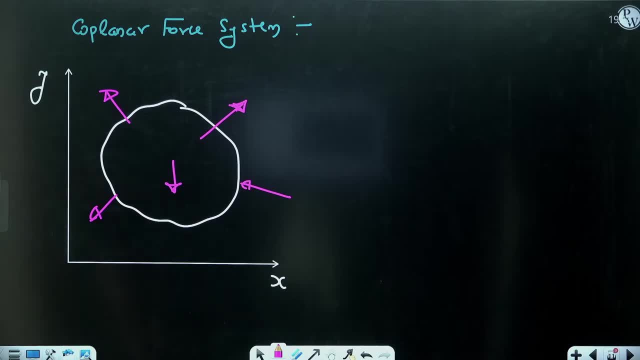 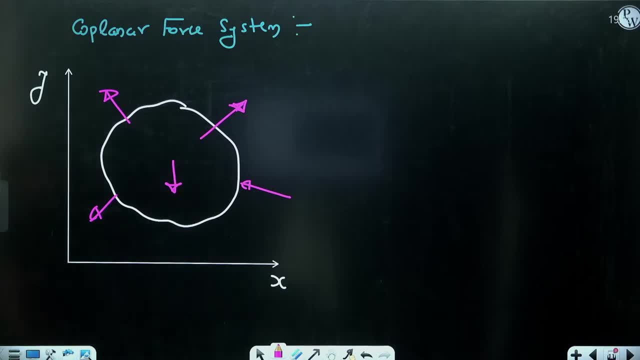 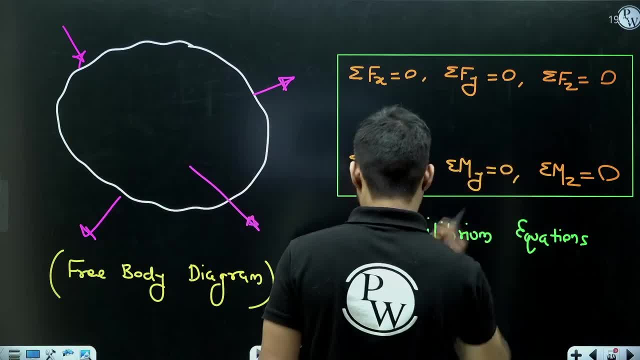 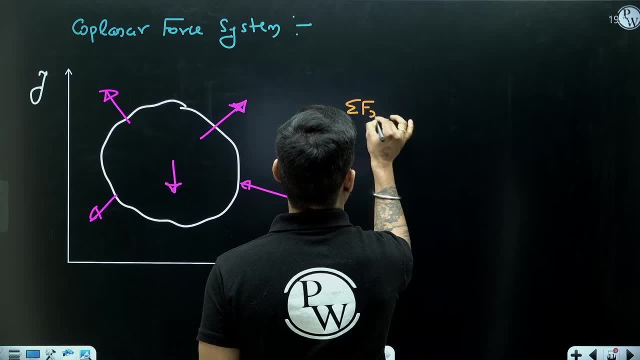 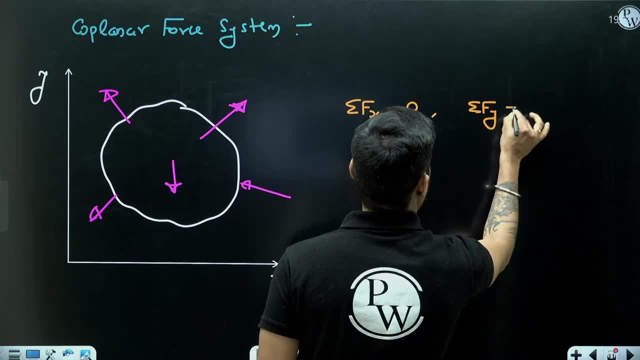 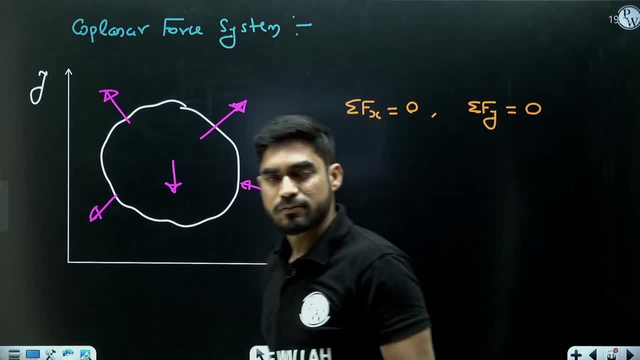 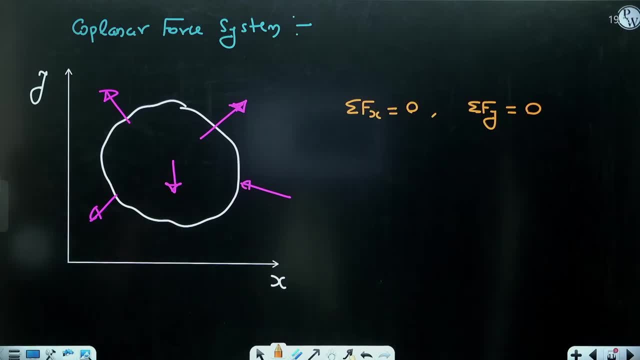 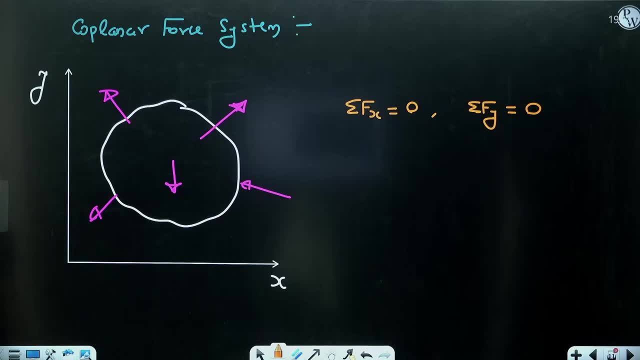 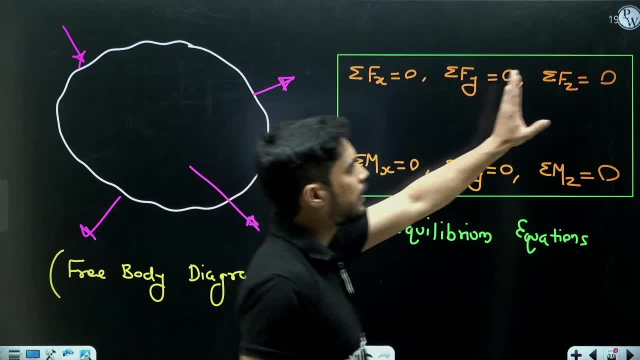 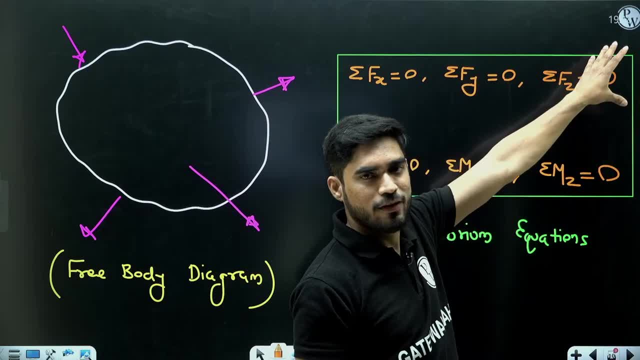 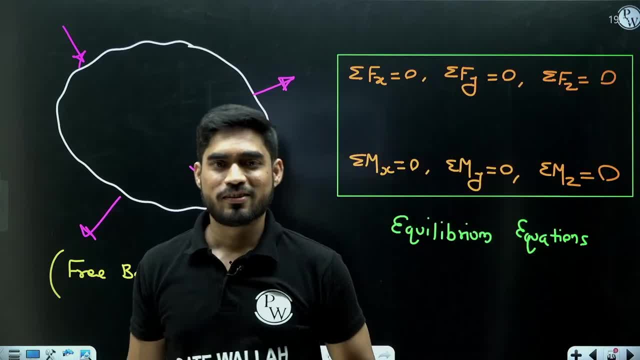 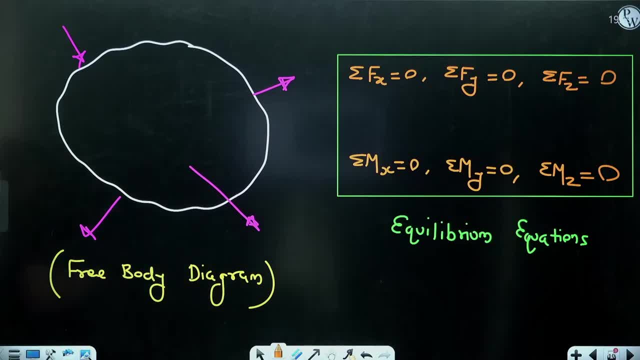 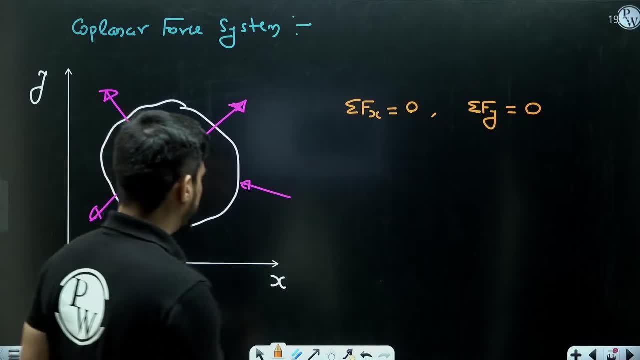 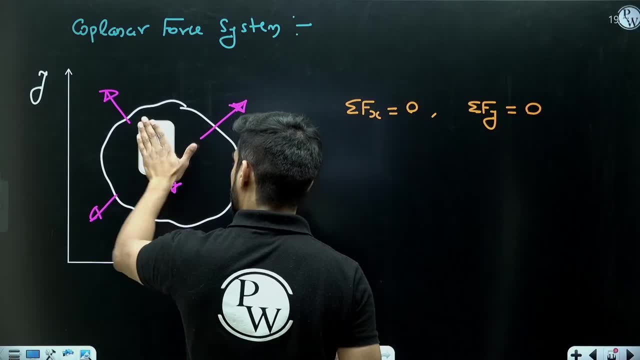 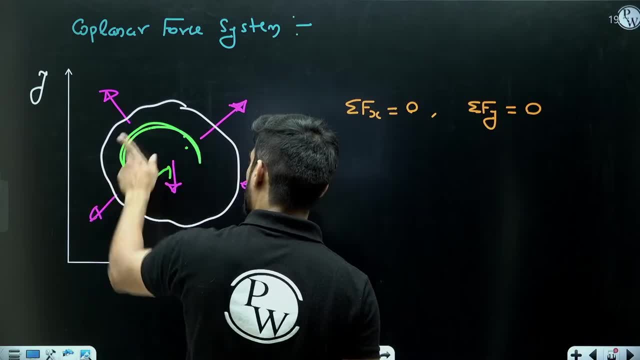 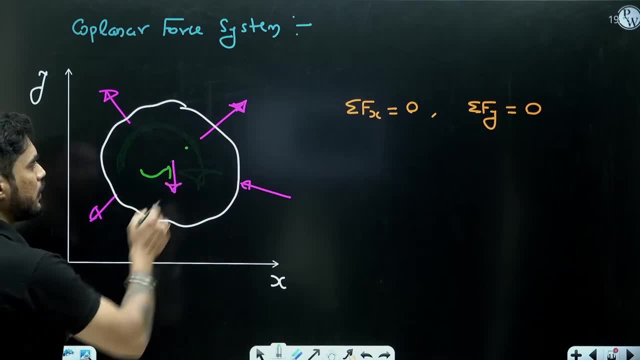 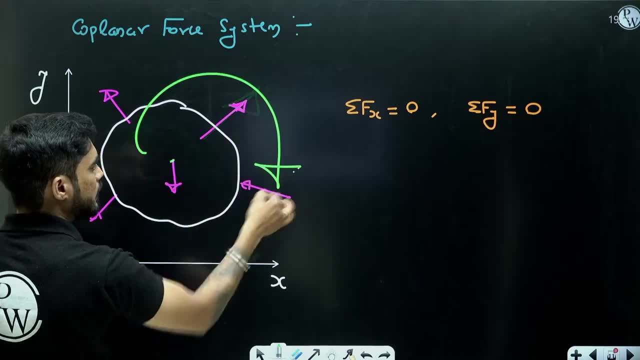 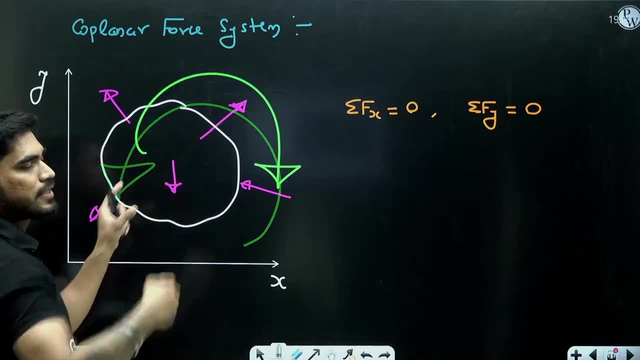 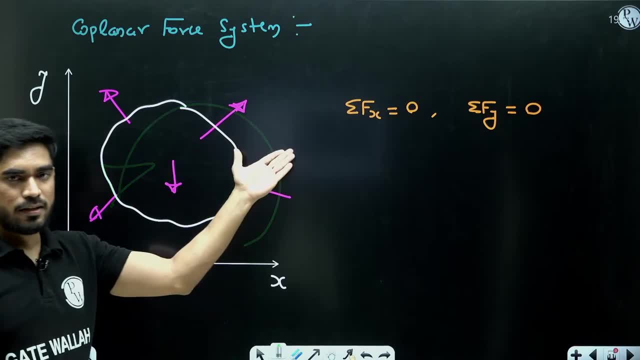 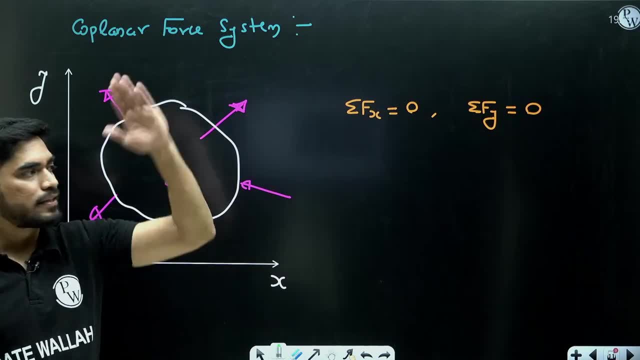 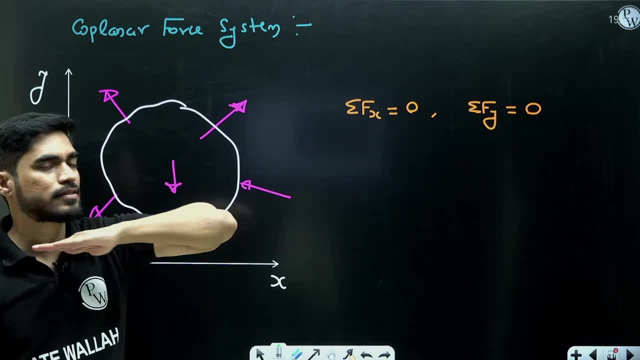 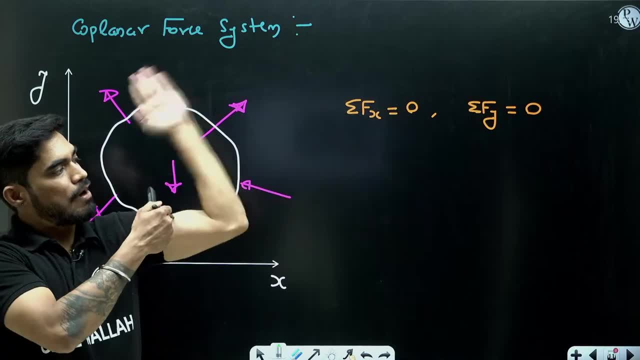 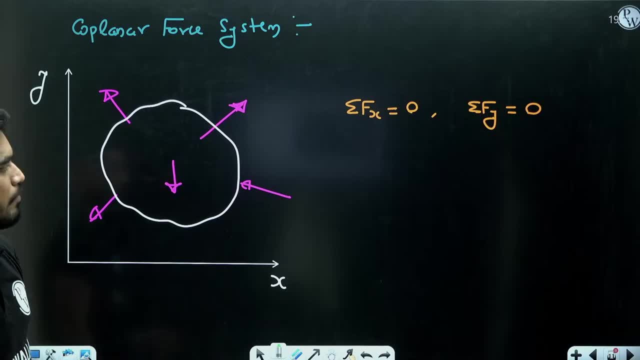 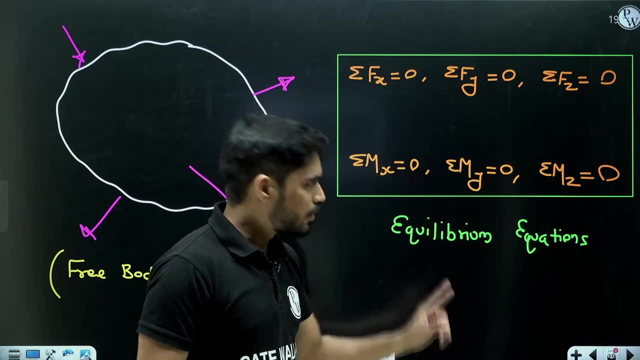 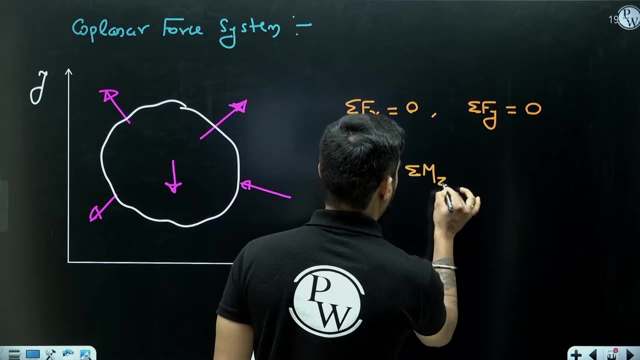 apply equilibrium equations on free body diagram. So we can only apply equilibrium equations on free body diagram. So we can only So net moment about x and y are already 0, because they cannot apply the moment about x or y. They can only apply moment about z. So you will only have this equation. summation of nz equal to. 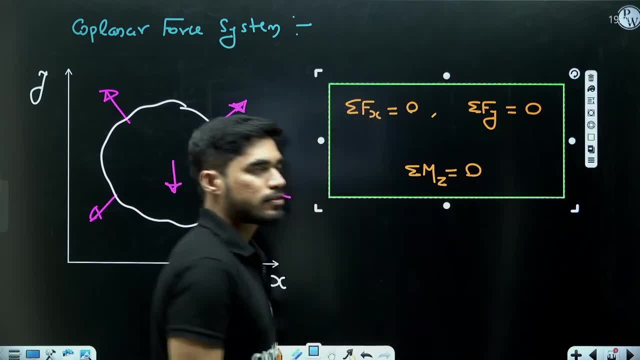 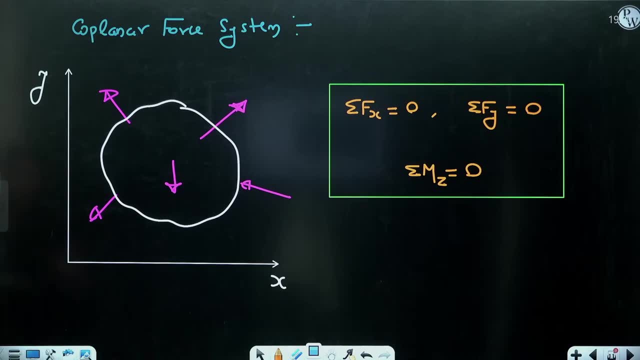 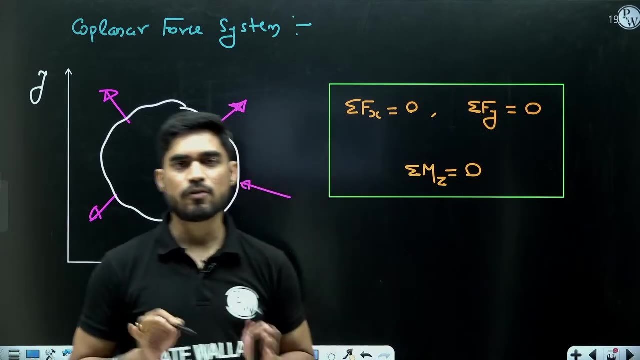 0.. So now, how many equations do we have? We have three equilibrium equations for a co-planar force system. This is the only force system that we are going to deal with in our syllabus. We are not going to deal with three-dimensional force system. So whenever we 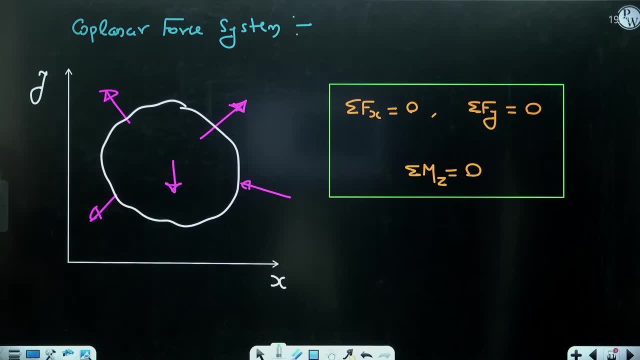 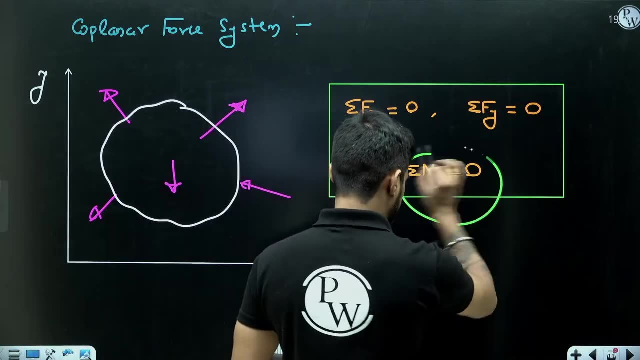 will solve problems. we will only use these equations: Summation of fx equals to 0, summation of fy equal to 0 and summation of mz equal to 0.. So what will be the steps to solve the problem? 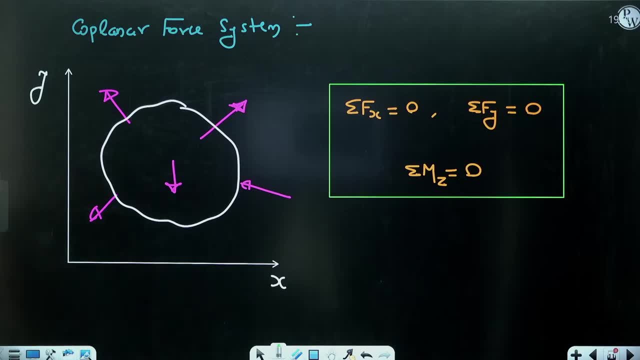 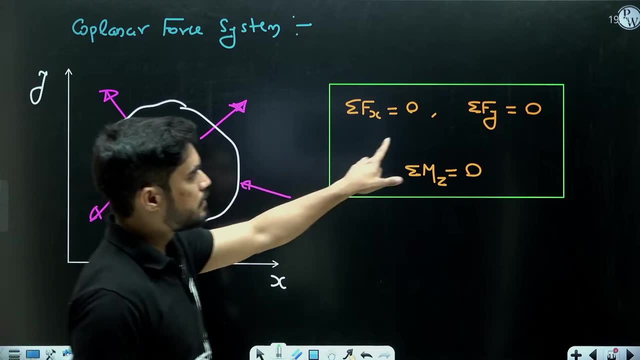 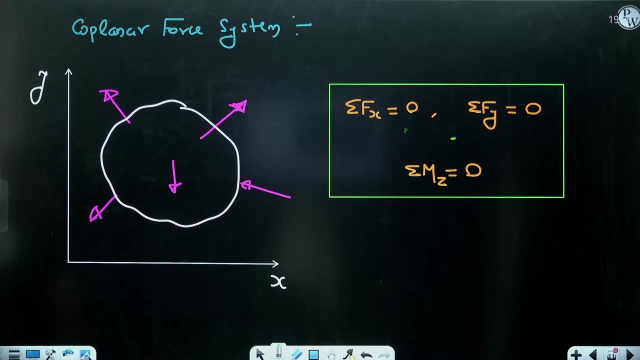 You will go to the diagram of the body. Whatever the body is in the question, you will draw the free body diagram of that body. Then you will apply these equations, You will solve the equations and you will find the unknown force. What are the unknown forces? Reaction forces, Whatever the reactions, the body? 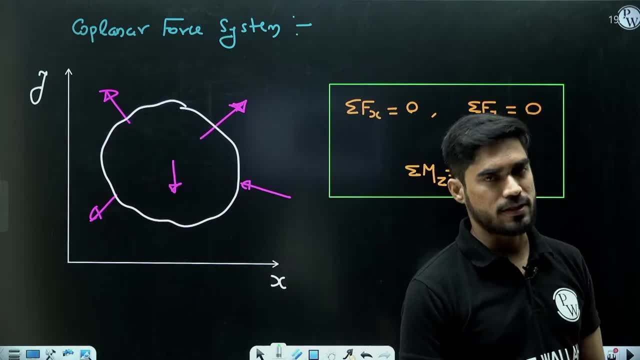 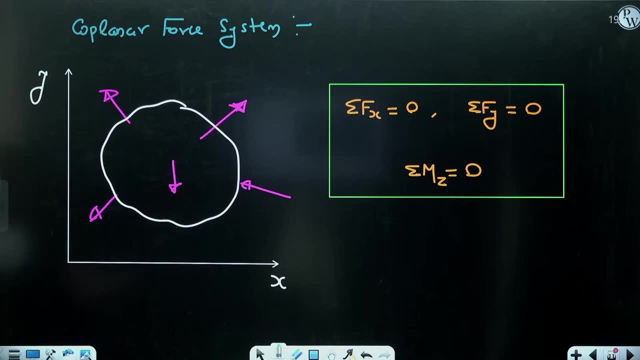 is getting from supports. Those are the unknown forces. So you will draw the FBD. You will find the unknown forces. You will try to find and apply the equilibrium equations, solve the equilibrium equation and find the reactions. Now, whenever you will draw the free body diagram, you will have to 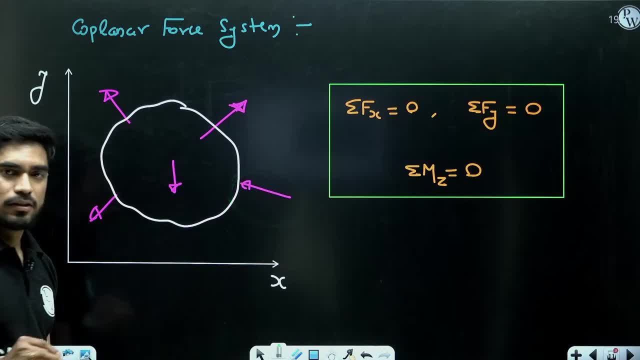 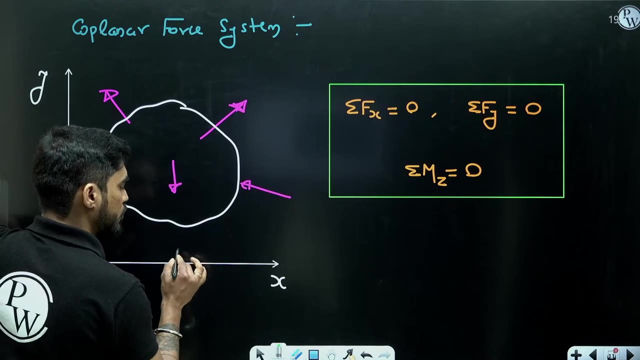 see what type of reactions you are going to get. So we have already seen what type of reactions do we have, right, In case of roller support, hinge support, fix support. Now, whenever you are confused about the direction, see, you have to know whether the force will be in x or y. But let's say 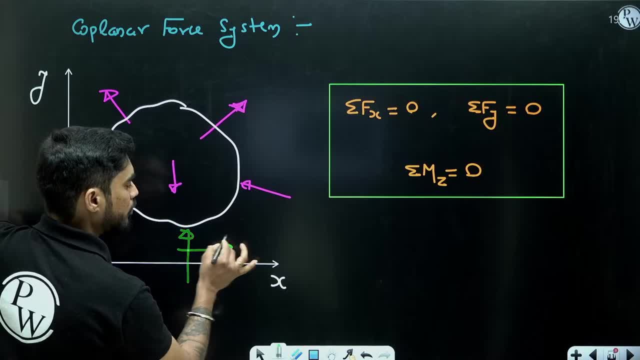 you know that the force will be in x or y, So you will have to know whether the force will be in x or y. So you force is in x, But you don't know whether it will be towards right or towards left. 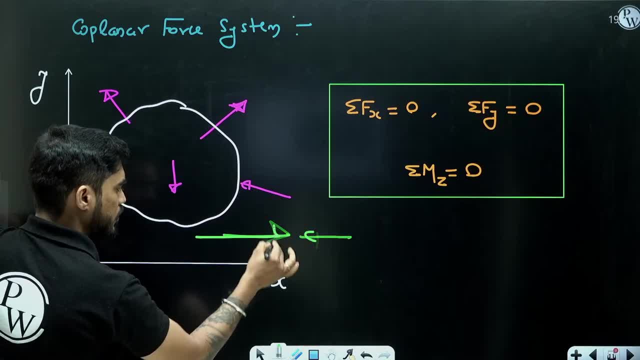 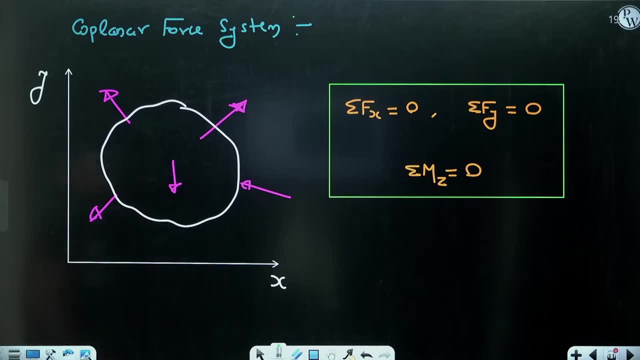 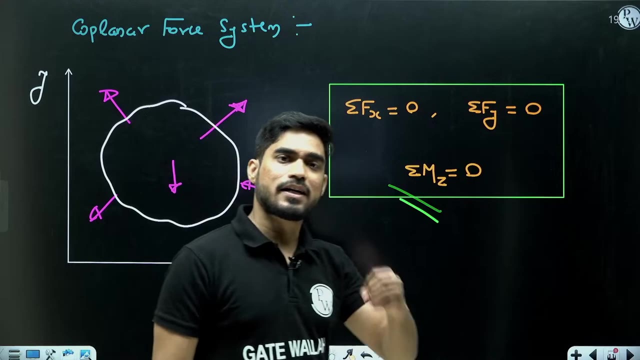 You assume any one direction. Let's say I have assumed the force to be towards right, to be in the positive x. If I am getting a positive answer by solving these equations, my assumption is correct, And if I am getting a negative answer, my assumption is wrong. 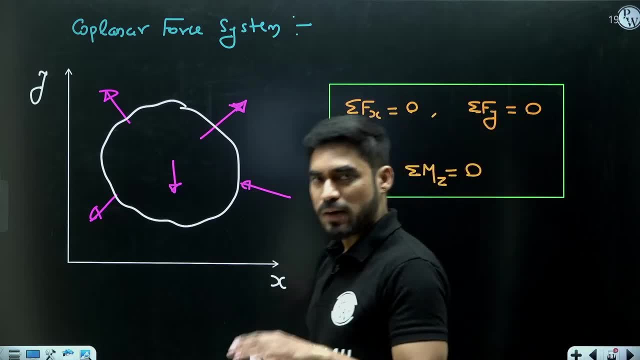 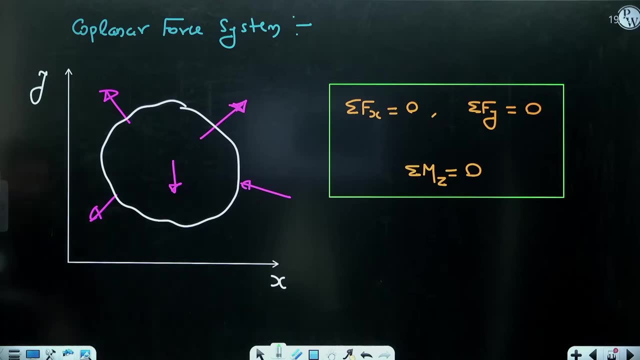 I hope this point is clear to you Whenever you are applying the reaction forces or reaction couple. you don't need to worry about the plus or minus direction, Plus x or minus x, plus y or minus y, clockwise couple or anti-clockwise couple. you don't need to worry about this. 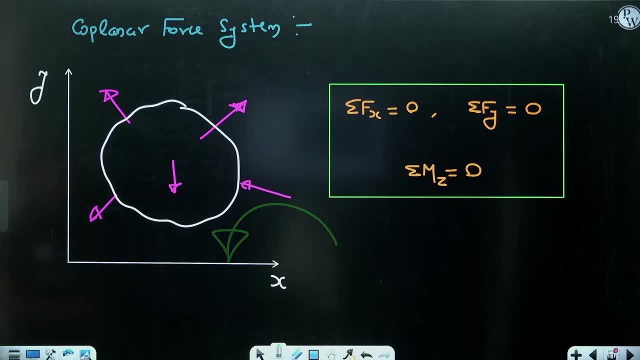 Assume any one direction. If you are getting positive answers by solving these equations, your directions are correct. If you are getting negative answers, your directions are wrong. But you can't do this If a force is in x direction and you are assuming y direction. 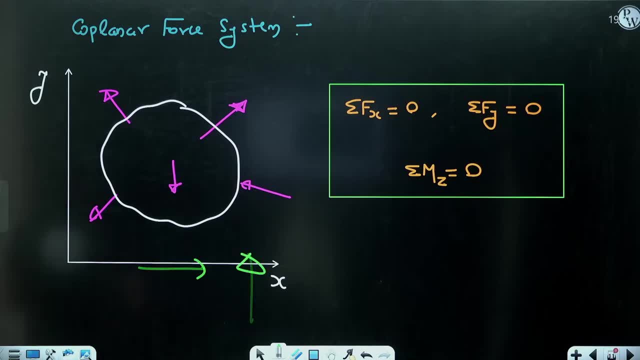 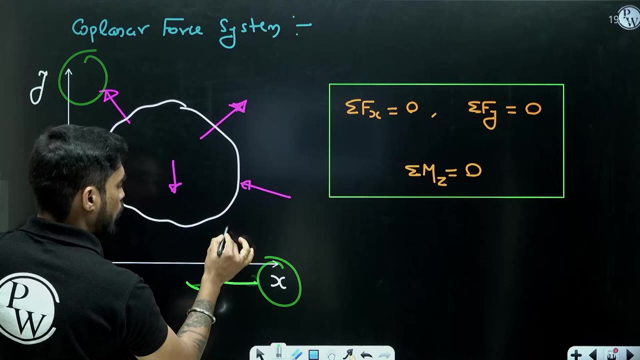 then you will have wrong answer. So you can't do this, You can't do that. I don't know whether the force is in x or y. I will just imagine You can't do that. You have to know whether the force is in x or y or in both directions, But positive x, negative x or positive y. 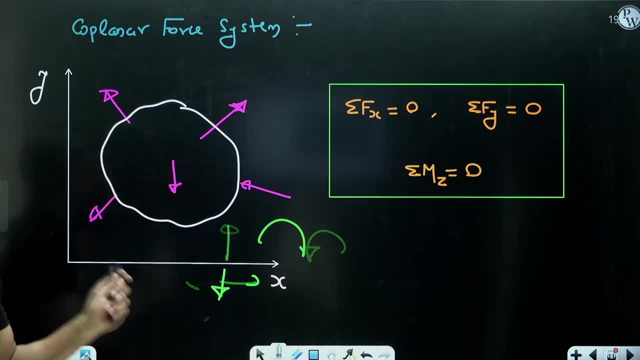 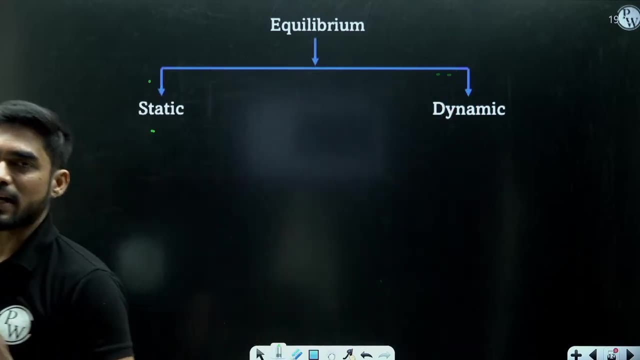 negative y or clockwise couple, anti-clockwise couple, that you don't need to worry about. I hope this point is clear. Now. equilibriums are of two types: static equilibrium and dynamic equilibrium. Understand the meaning of both types of equilibrium, Because it makes 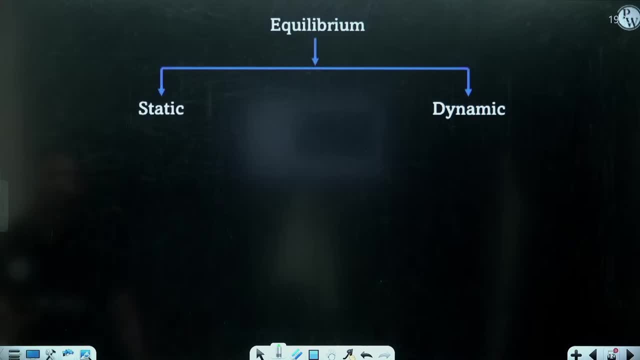 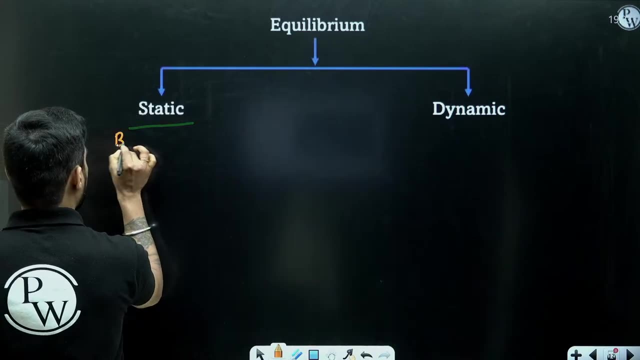 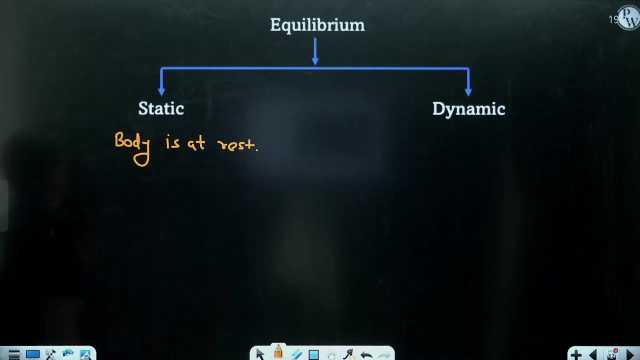 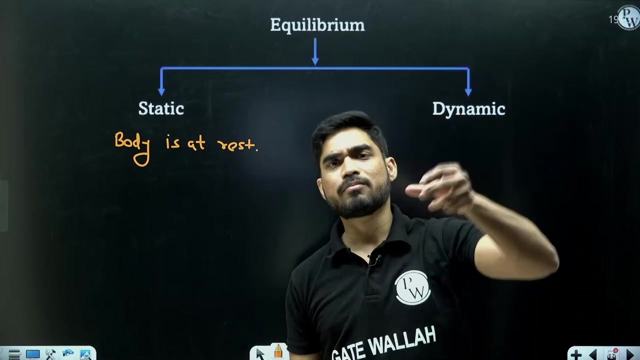 confusion. It creates confusion. Static equilibrium means the body is at rest. For example, let's consider any one member of the structure. you are living in the house. you are living in beam or column or bar, whatever structural member you consider. 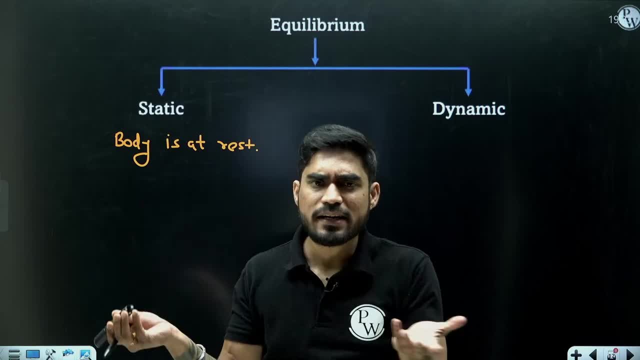 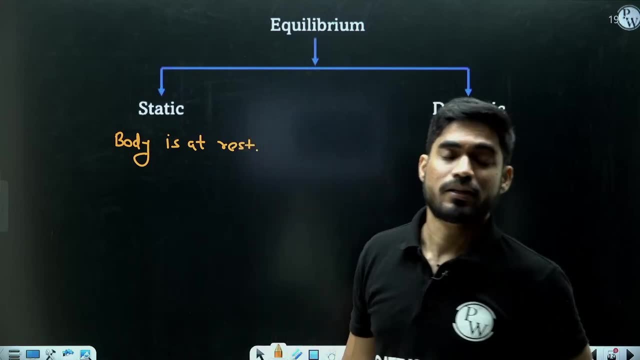 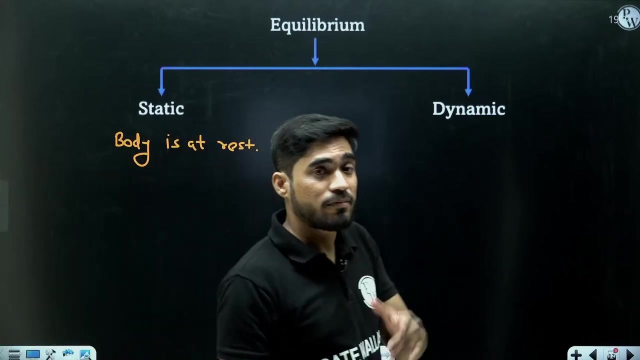 That member is in static equilibrium because it is at rest. It is not moving. Yes, What is dynamic equilibrium? Dynamic means moving, So the body is moving. If the body is moving, how come it is in equilibrium? Equilibrium doesn't only mean that the body has to be at rest, Even if the body is. 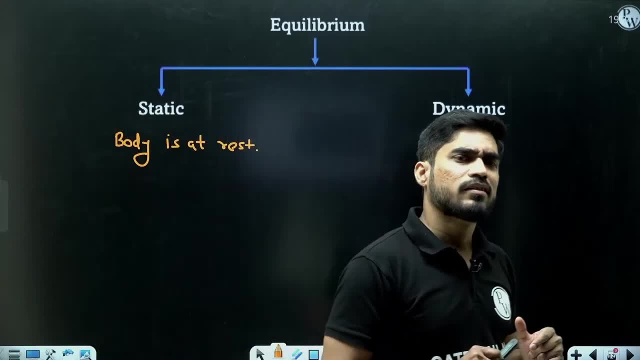 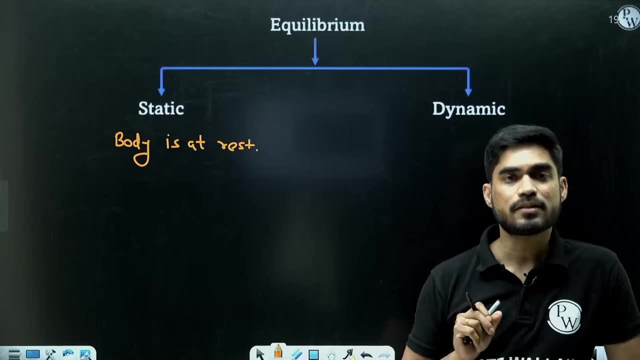 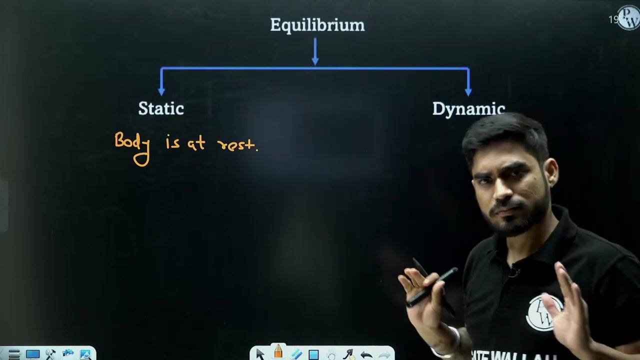 moving it can be in equilibrium. How Equilibrium means the net force and moment must be zero. Yes, Let's say you have pushed a body and then you have left it. You have given a body a push And then you have left it. 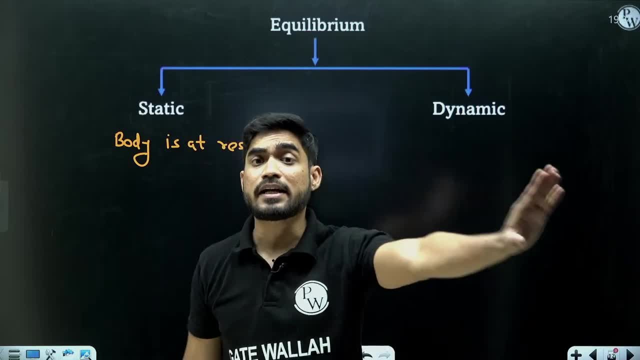 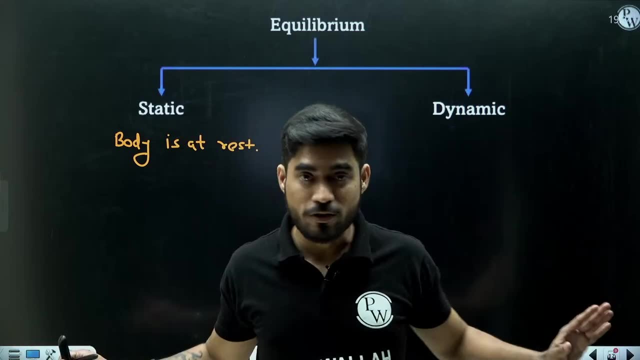 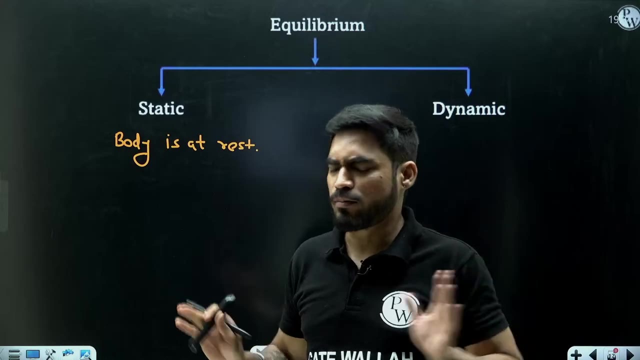 And now the body is moving and there is no force acting on the body. Assume the condition Even friction forces are also zero. Imagine friction force is also not there. You have pushed a body, The body is moving And now there is no force acting on the body. 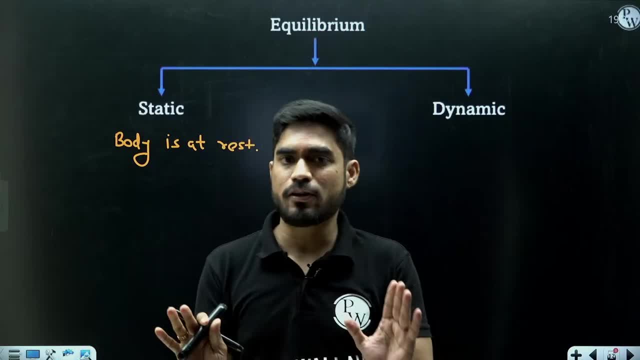 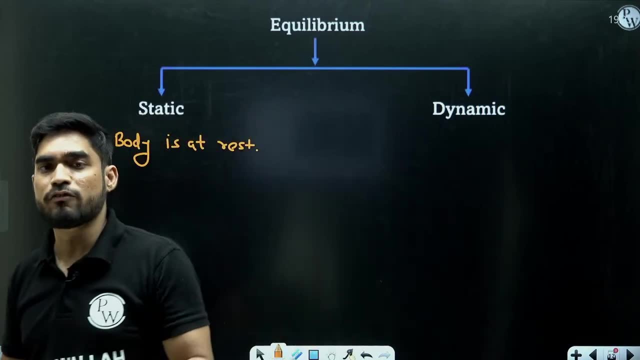 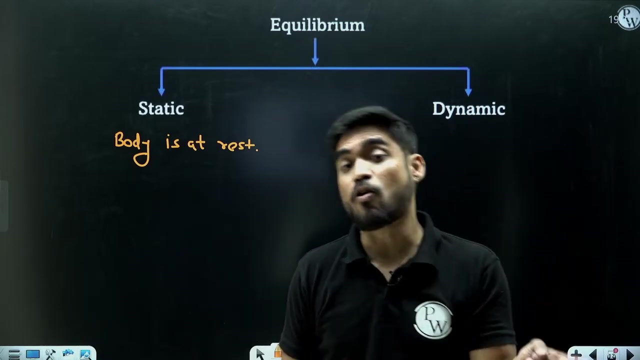 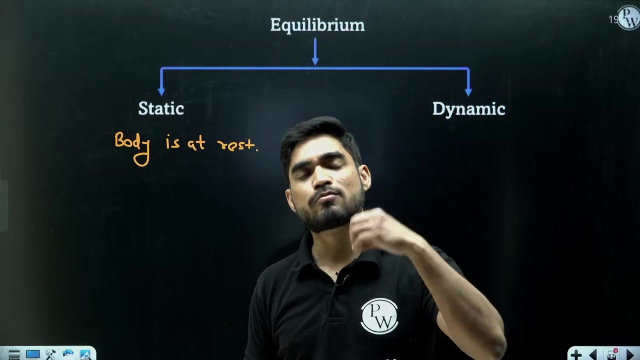 Even the friction force is also zero. So net force is zero. Now the body is moving. So if the net force on the body is moving, it will not accelerate. It means it will move with constant velocity in the same direction. If, let's say, the body is moving at 10 km per hour in x direction, 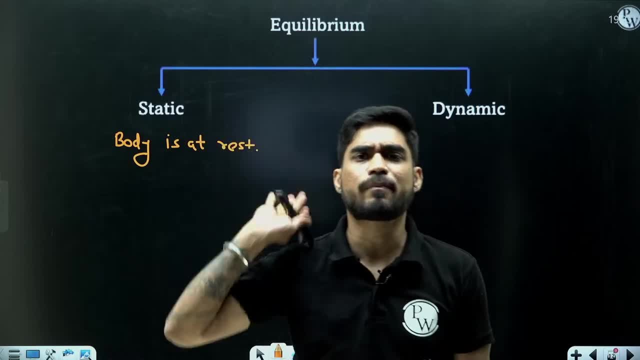 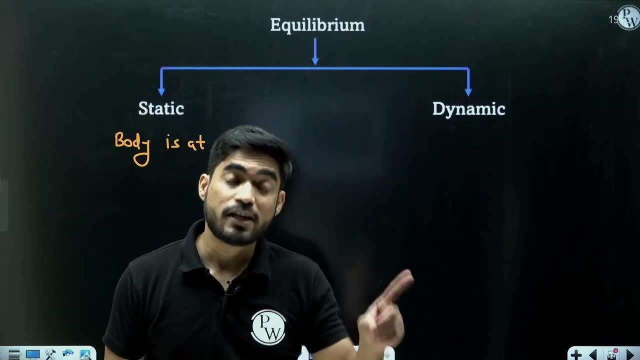 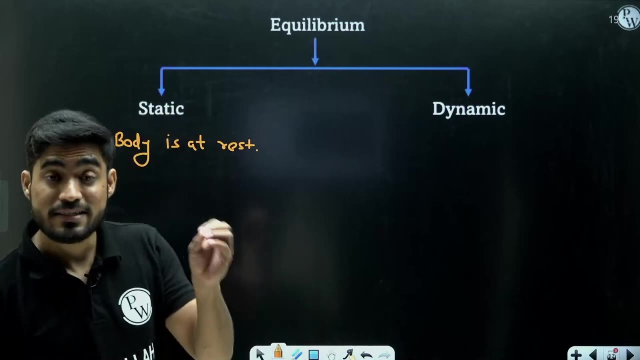 It will keep on moving in x direction with 10 km per hour. It will not accelerate. So net force is zero. So there will be no acceleration, There will be no change in velocity, But the body can move with constant velocity in the same direction. 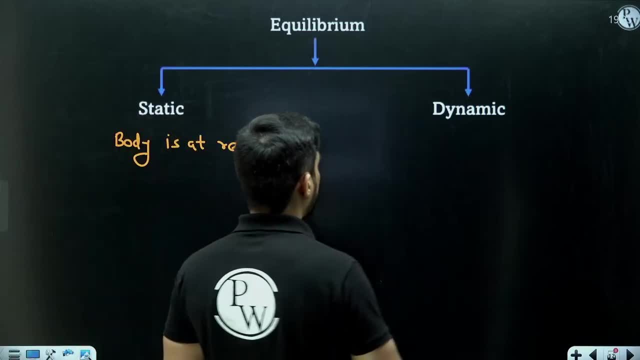 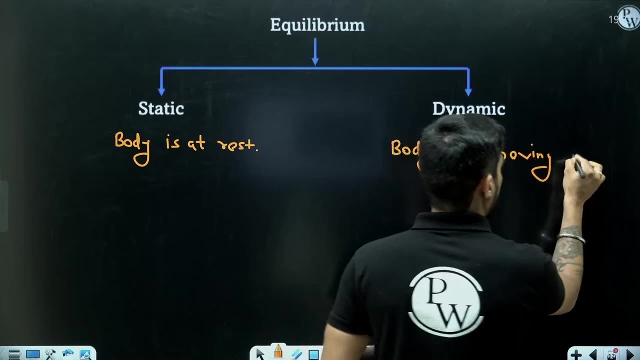 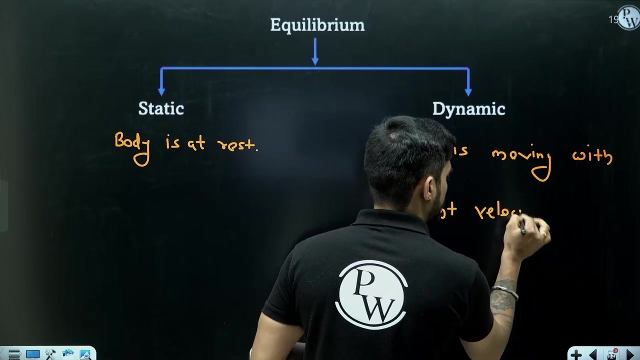 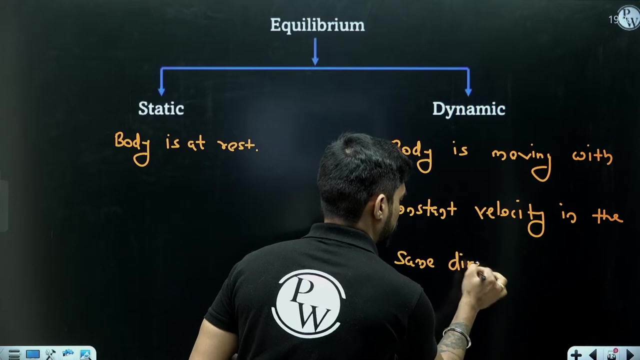 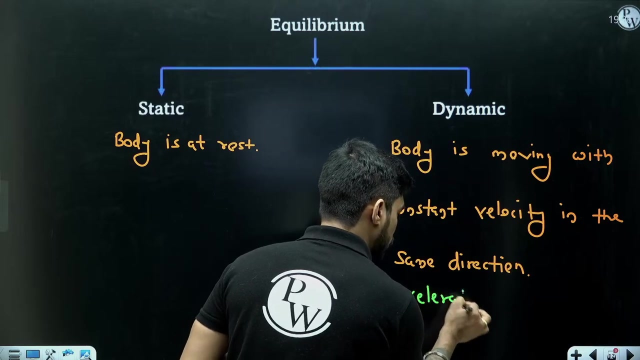 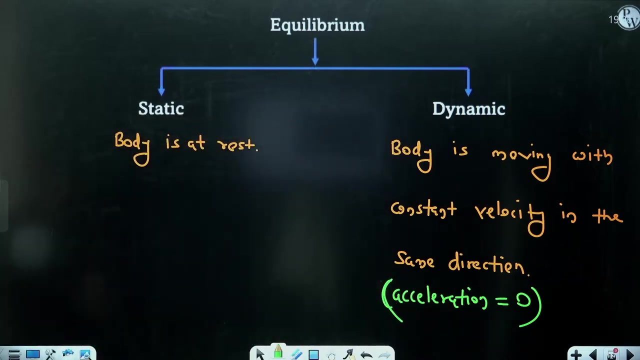 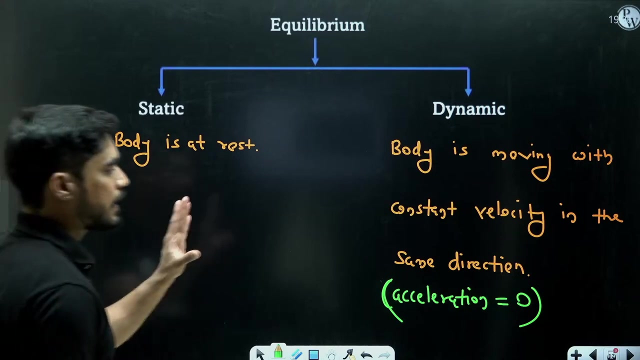 So dynamic equilibrium means body is moving with constant velocity In the same direction. Acceleration is zero. So understand about dynamic equilibrium: Even if the body is moving, but it is moving with constant velocity in same direction, It means it is in dynamic equilibrium. 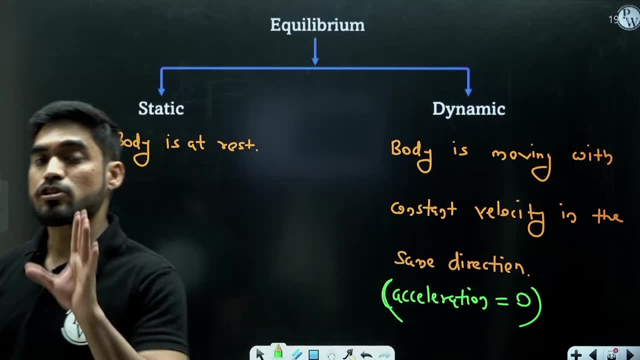 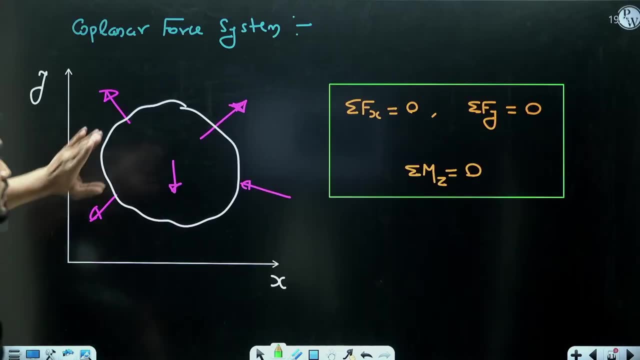 The acceleration of the body is zero. So you can have a dynamic equilibrium, You can have static equilibrium, You can also have dynamic equilibrium. In both cases these equations are applicable. Equilibrium means equilibrium. Net force and moment must be zero. 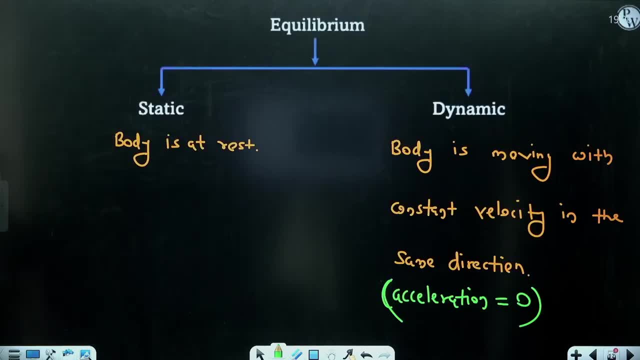 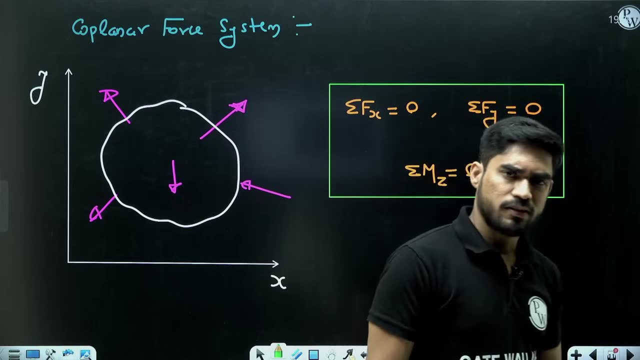 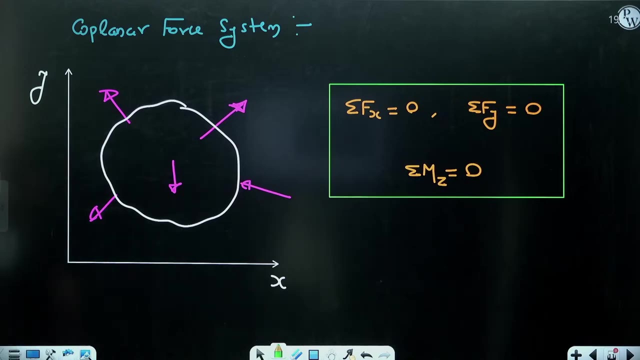 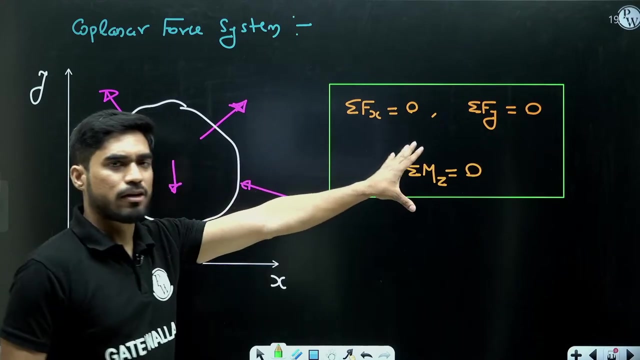 Whether it is static or dynamic. Okay, Chalo, Now let's say you have a question, You draw the free body diagram of the body, There are three reactions Which are unknown And you have three equilibrium equations. So, by applying these three equilibrium equations, 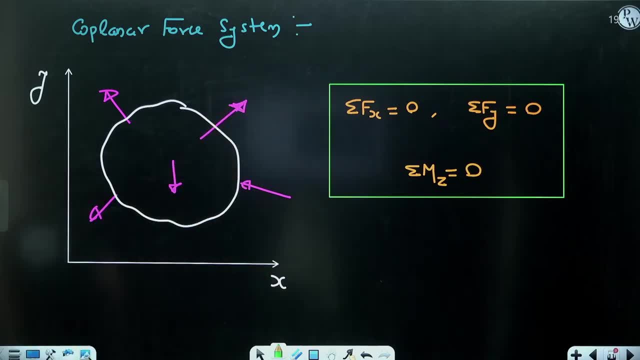 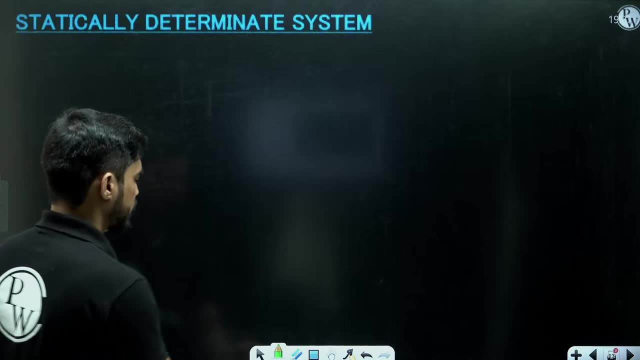 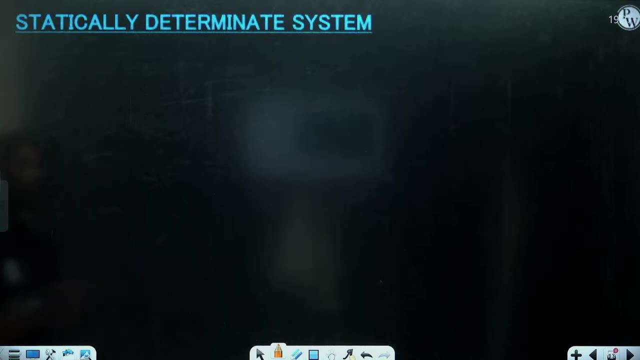 you can find out the three unknown forces. Okay, These type of problems, where the number of equilibrium equations are equal to the number of unknown forces, are known as statically determinate problems or statically determinate systems. What do we mean by statically determined system? 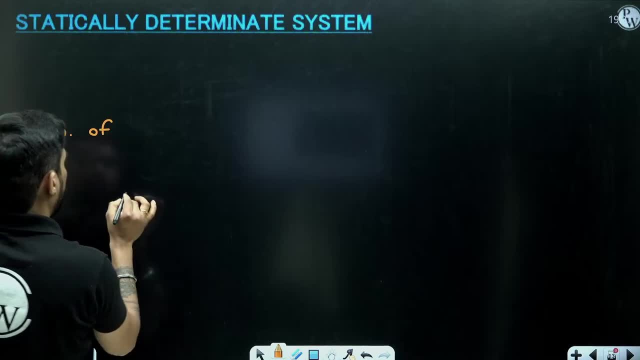 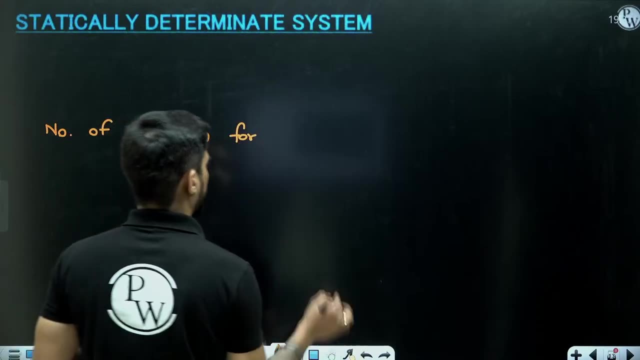 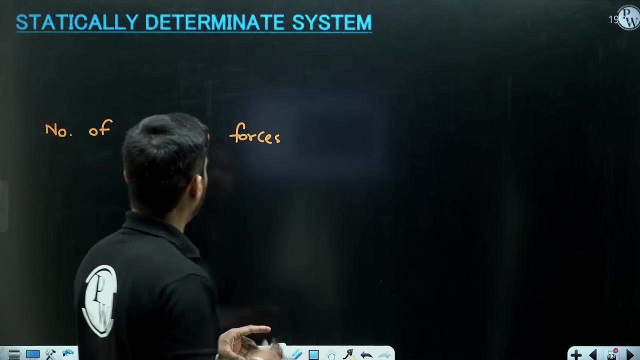 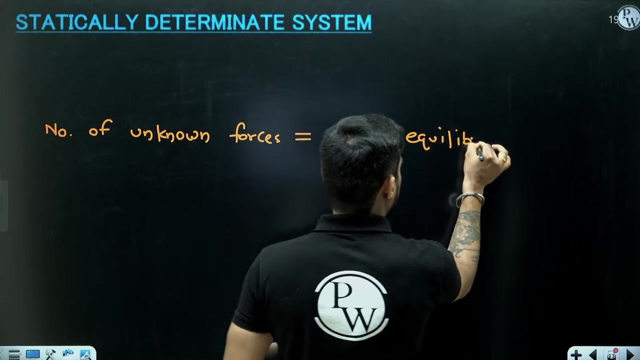 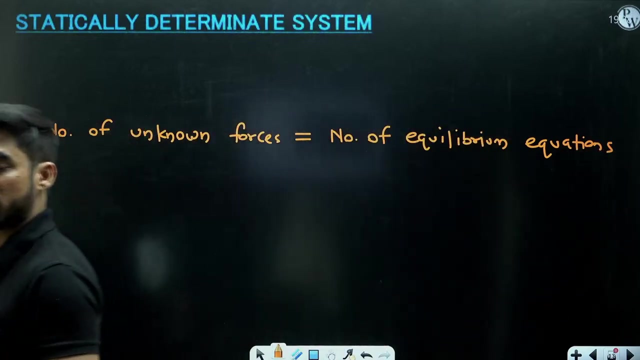 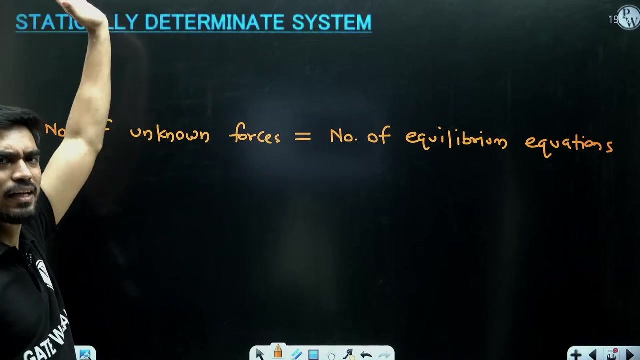 Number of unknown forces Or couple. i will not write forces and couple or couple. Assume the number of unknown forces are equal to number off equations. So if I can find all the unknown forces just by using equilibrium equations, it is known as a statically determinate system. Understand the meaning of this sentence: statically. 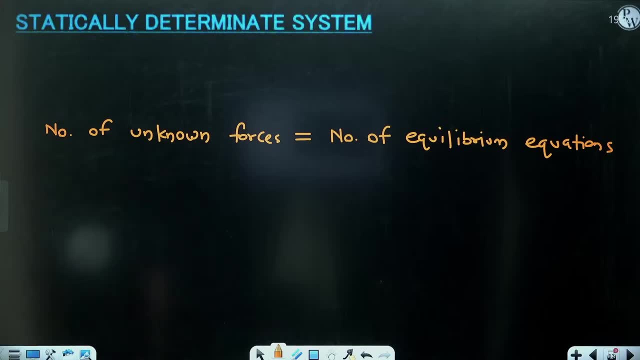 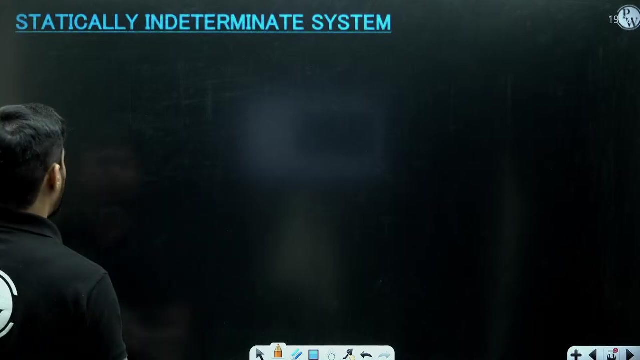 determinate. Determinate means I can determine. Statically means by applying static equilibrium equations. So if I can determine the unknowns just by static equilibrium equations, it this is known as a statically determinate system. But if the number of unknowns are more, 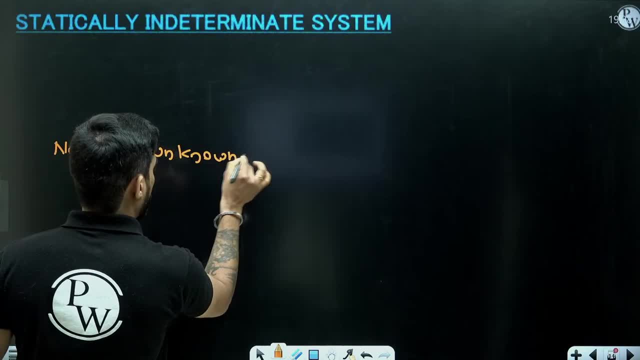 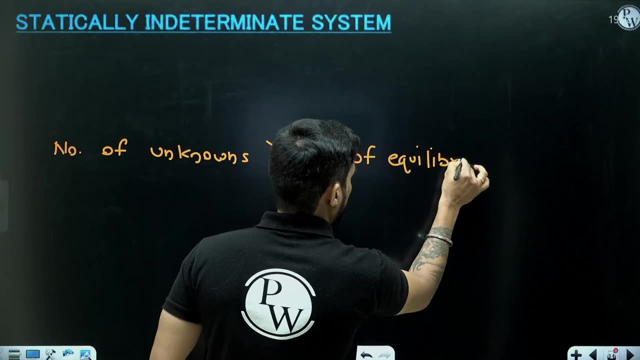 if the number of unknowns are more than the number of equilibrium equations, then what? If the number of unknowns are more than the number of equilibrium equations, then what If the number of unknowns are greater than the number of equilibrium equations? you will 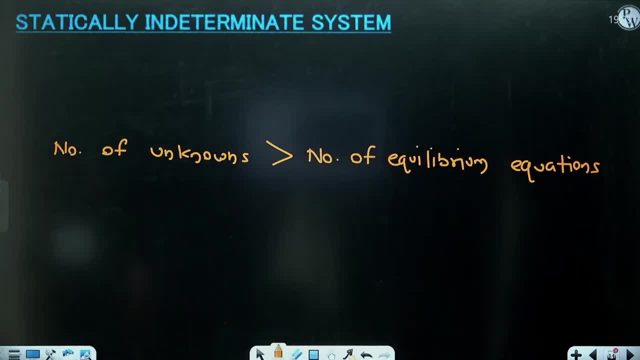 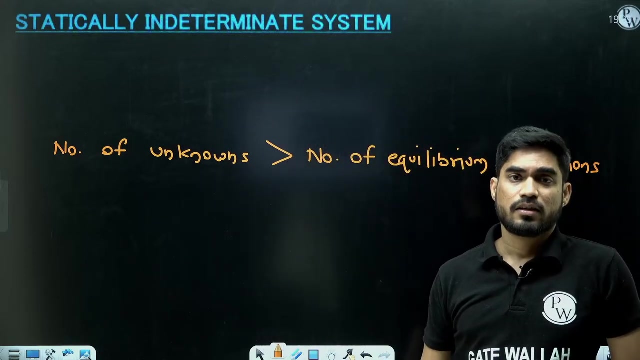 not be able to find all the unknowns. So these type of problems are known as statically indeterminate problems. So how are we going to solve these problems? For solving these problems we have different type of equations and these problems cannot be solved in this. 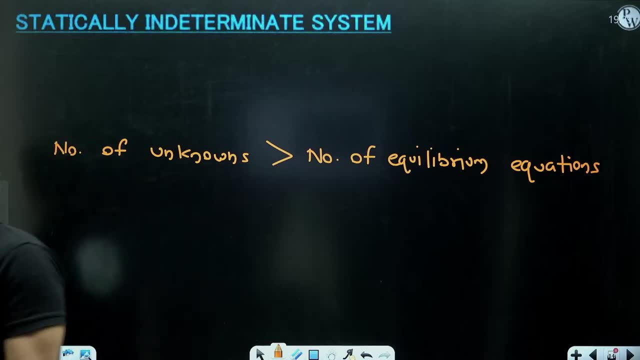 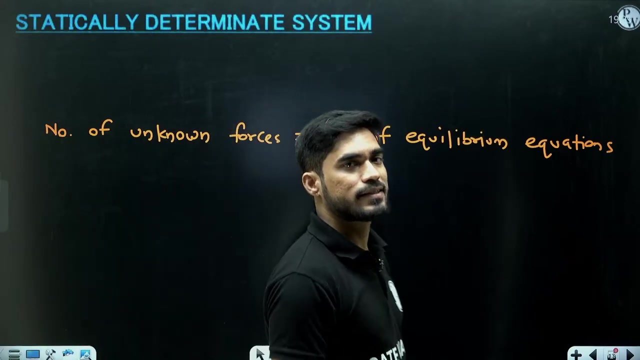 subject For solving these problems, we have to study strength of materials. When you will study strength of materials, you solve statically indeterminate problems. So in engineering mechanics we only deal with statically determinate problems. we do not deal with statically indeterminate. 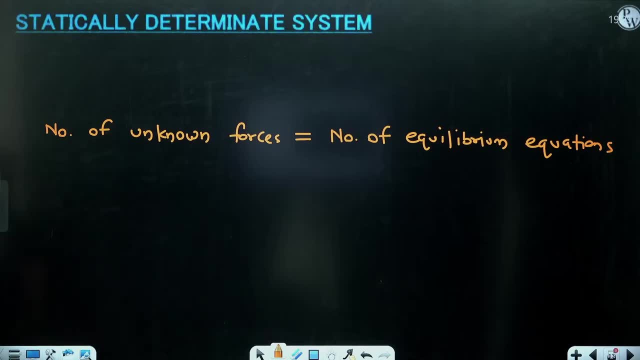 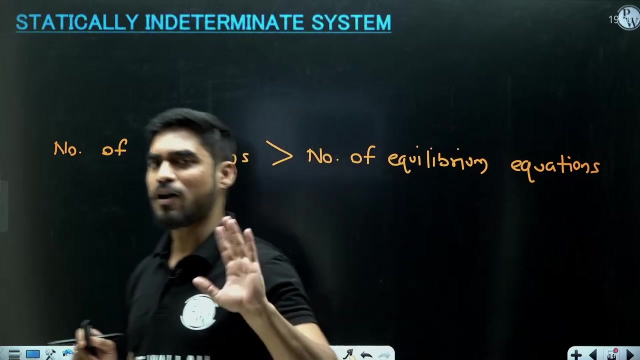 problems. So whenever you find a question of engineering mechanics, it has to be statically determinate. only Indeterminate problems are solved in a statically determinate problem- strength of materials. So let us start solving problems. We have all the concepts we need to. 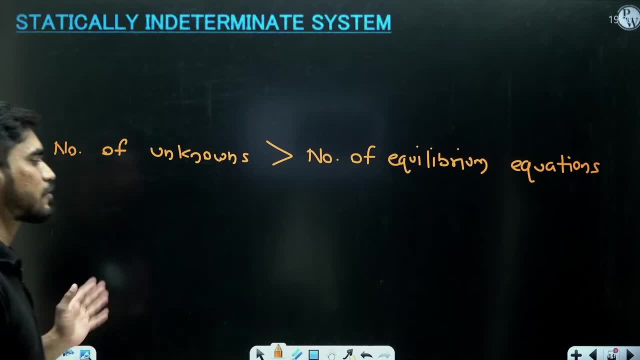 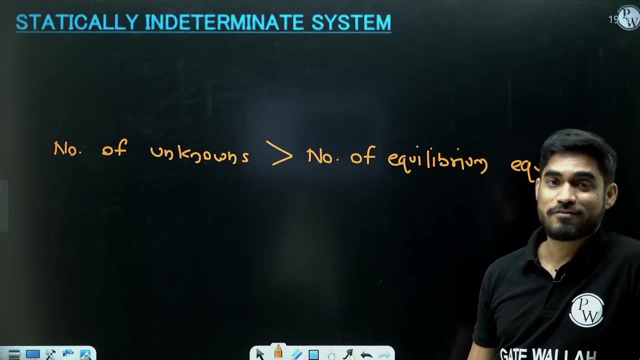 solve the problem. Let us apply these concepts and let us solve problems. But before getting into that, we have some interesting cases of equilibrium. So let us first find out these cases. The first case is equilibrium of a two-force system. Now, what do we mean by? 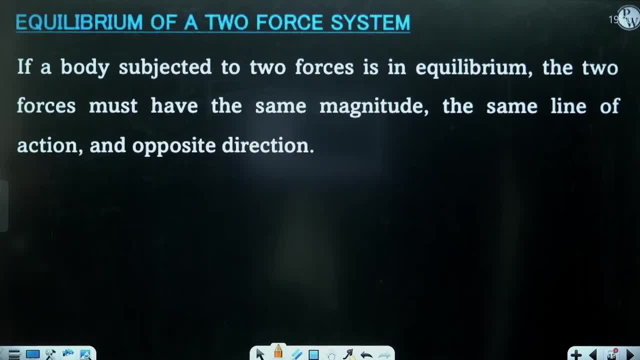 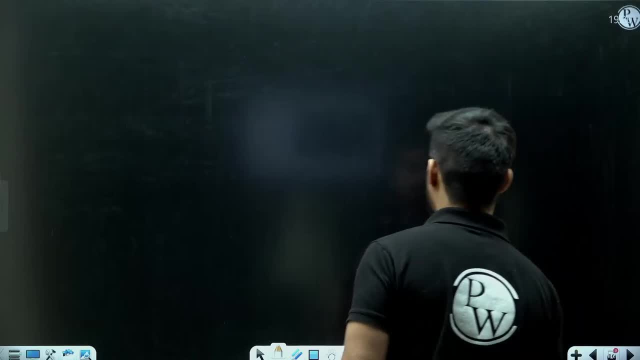 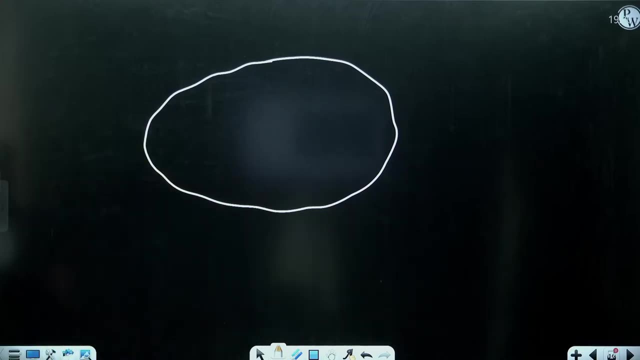 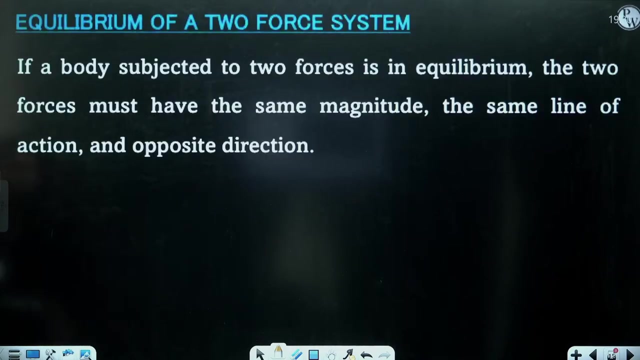 equilibrium of a two-force system. Understand the meaning of this. If a body is subjected to two forces, if a body subjected to two forces, only two forces, there is no third force. If a body is subjected to two forces and it is in equilibrium, it says that the forces must have. 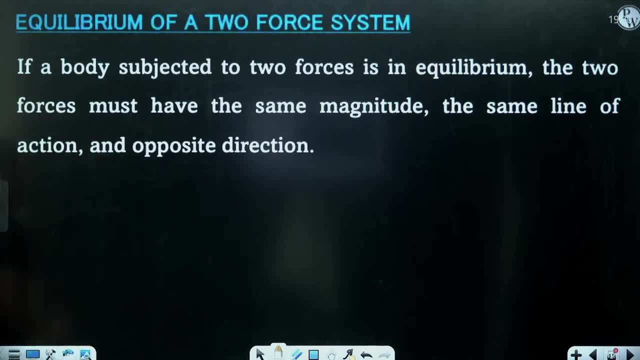 the same magnitude, same line of action and opposite direction. Wait a minute, okay. So what do we mean by equilibrium of a two-force system? Well, the first case is equilibrium of a two-force system. So if a body is subjected to a two-force, 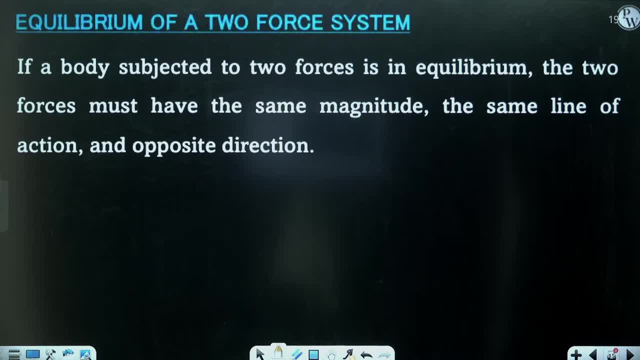 system, it is in equilibrium. So what do we mean by equilibrium of a two-force system? Well, the first case is equilibrium of a two-force system. So what do we mean by equilibrium of a two-force system? Well, the first case is equilibrium of a two-force system. So 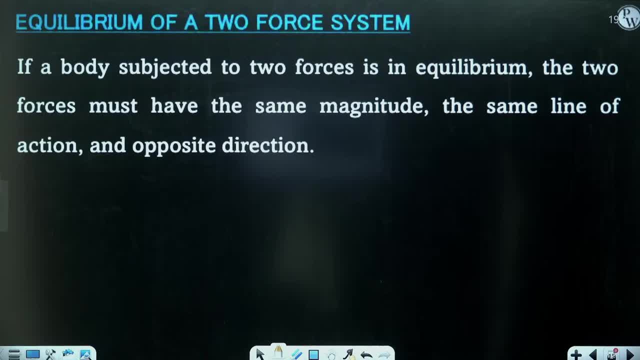 what do we mean by equilibrium of a two-force system? Well, the first case is equilibrium of a two-force system. So what do we mean by equilibrium of a two-force system? you, I'm so sorry, there was an emergency. I have to take a pause. 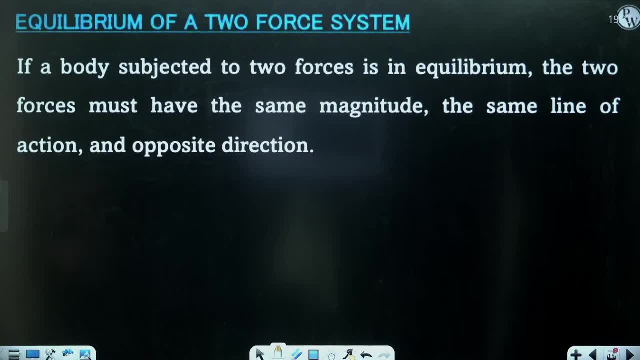 Sorry for that, I'm back, I'm back. I'm back. Okay, So we were discussing this first interesting case, Although it's not a very big case, and you will not find questions from this case because this is a very easy problem. 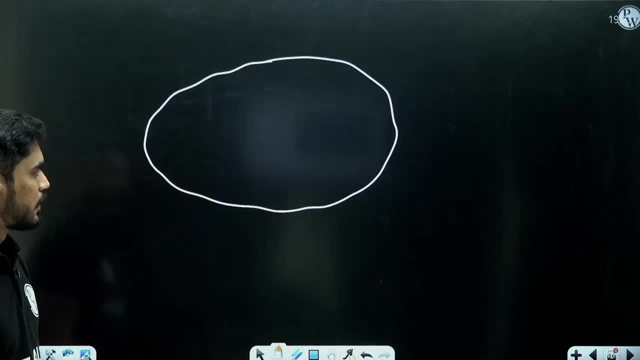 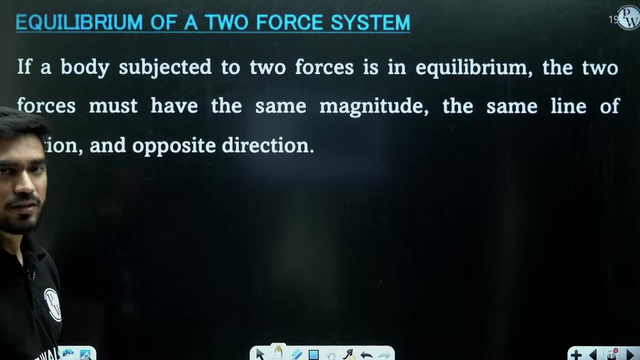 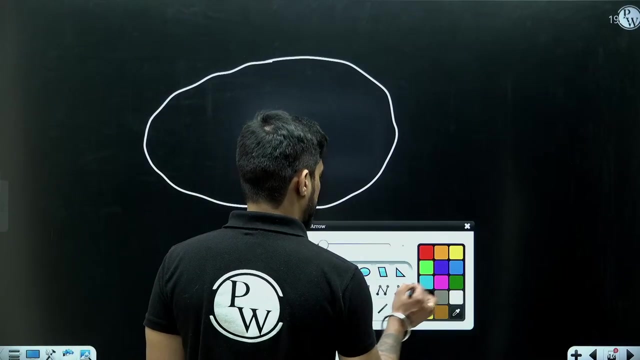 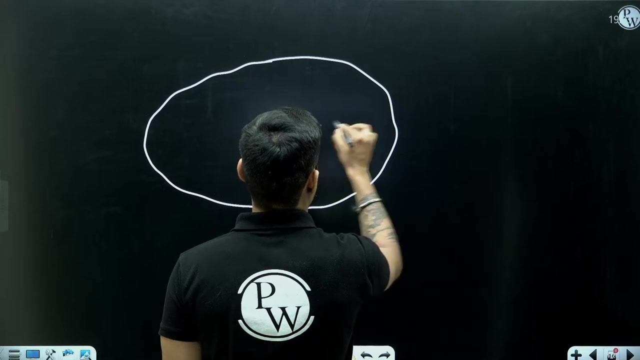 If a body is subjected to only two forces, then according to this case, the bodies, the forces, must have the same magnitude, the same line of action, and opposite direction Means let's say there is one force like this, Okay, And the body is subjected to only two forces. 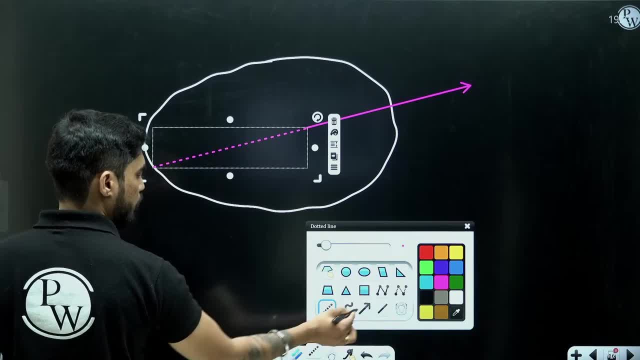 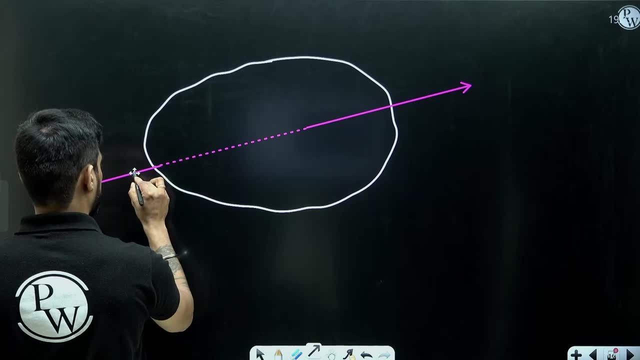 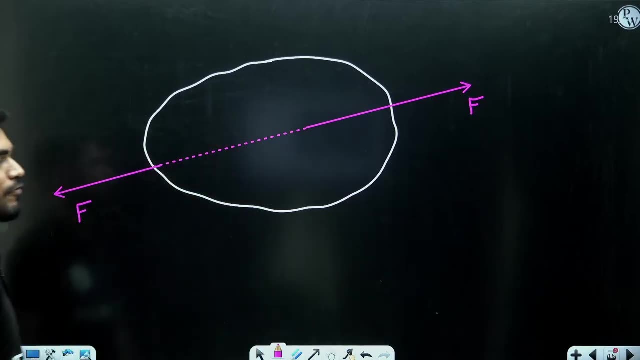 Okay, It means that the second force must be acting like this only, And if this force is F, this must also be equal to F, So they should have the same line of action, same magnitude and opposite direction. Let's say, one force is acting like this. 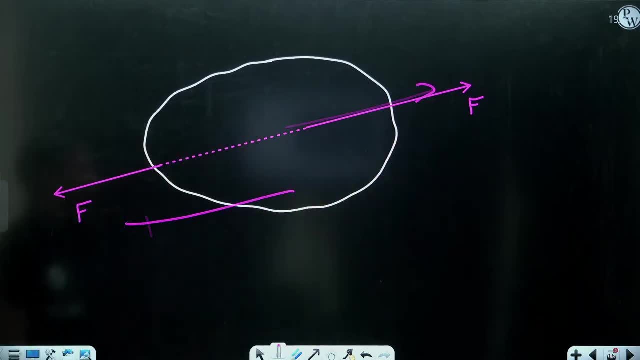 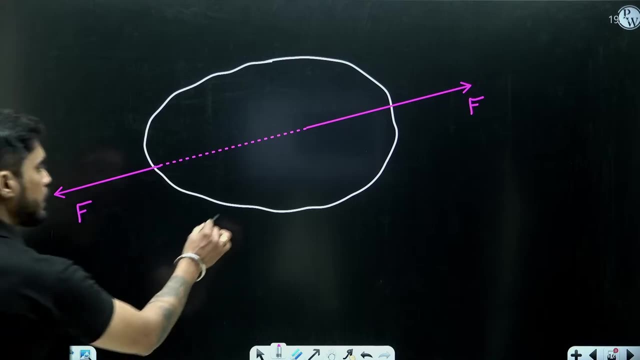 And another force is acting like this. Can the body be in equilibrium? Let's say both are equal and opposite, But their line of action is different. Can they be in equilibrium? No, They will form a couple. The body will start rotating. 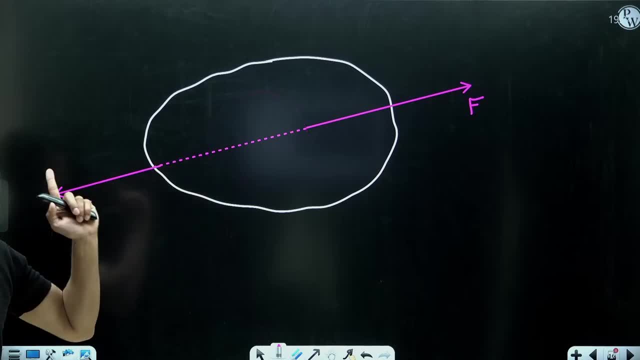 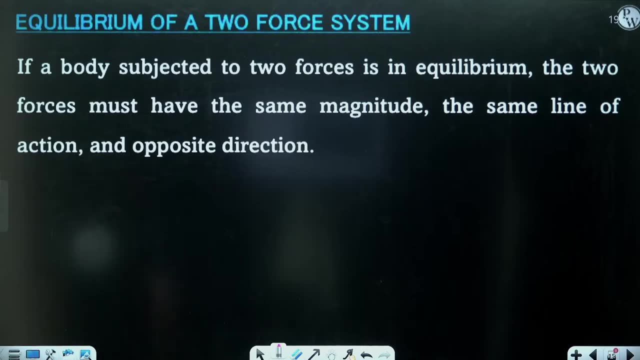 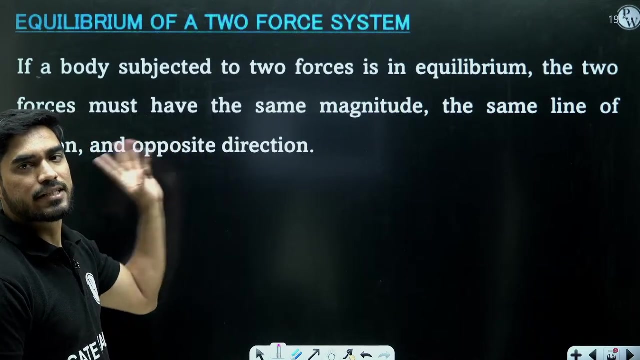 So this cannot happen. If the body is subjected to only two forces and the body is in equilibrium, then the two forces must be equal, Opposite, and should have the same line of action. Okay, Now you will not get questions from this case, because it will be very easy. 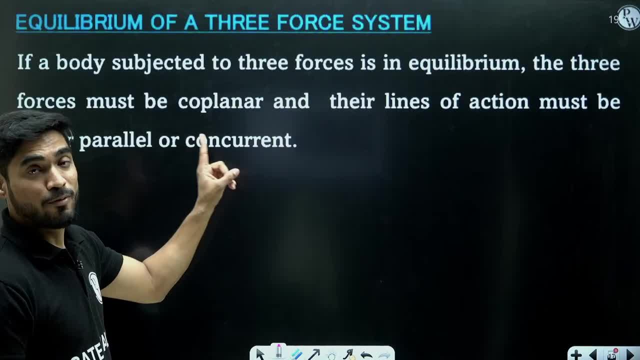 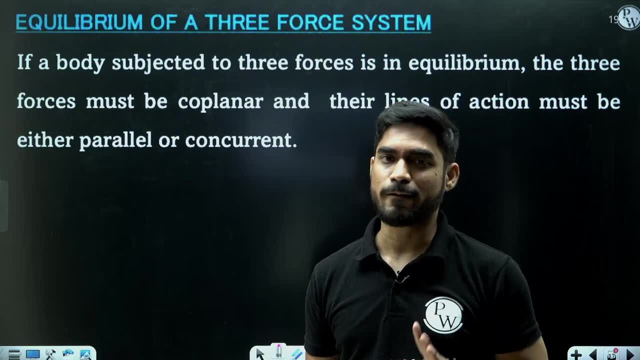 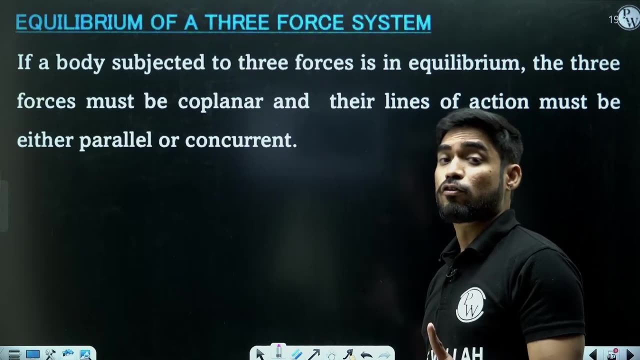 Right Now, this case is very, very important. Equilibrium of three forces. Let me tell you, you will find lots of questions based on this concept. Okay, So understand this concept. If a body is subjected to three forces, and it is. 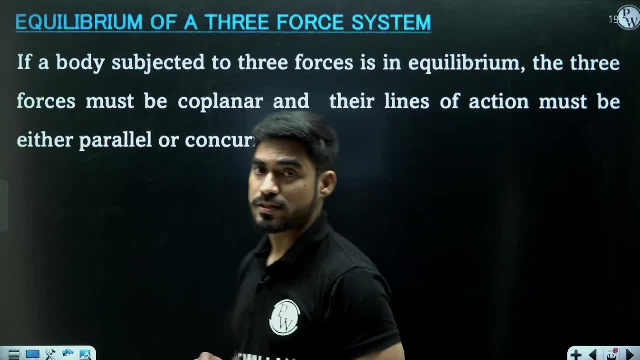 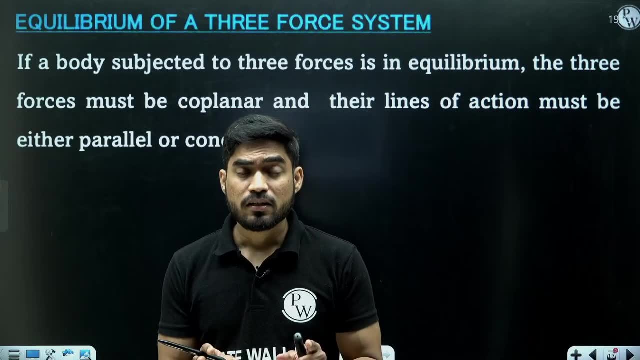 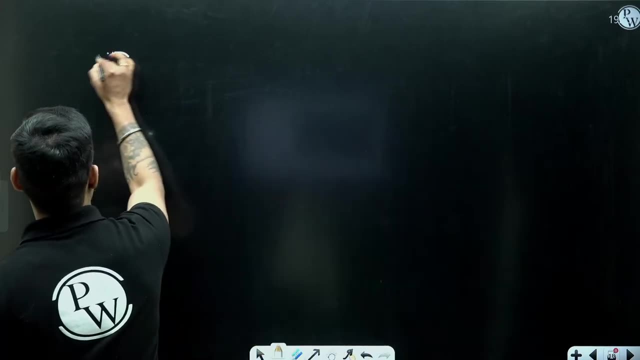 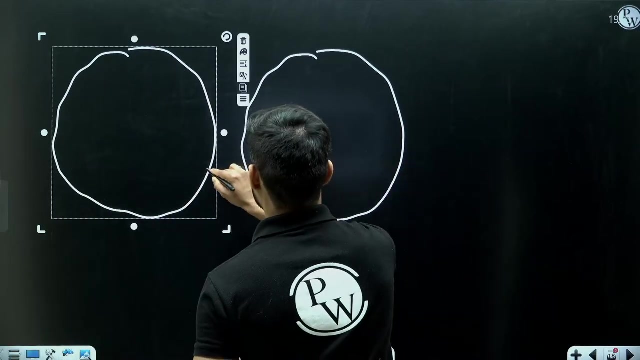 it is in equilibrium, then the three forces must be coplanar, parallel or concurrent. It means, if the body is in equilibrium, let's say this is our body. Okay, Let's say this is our body. Then, according to this statement, 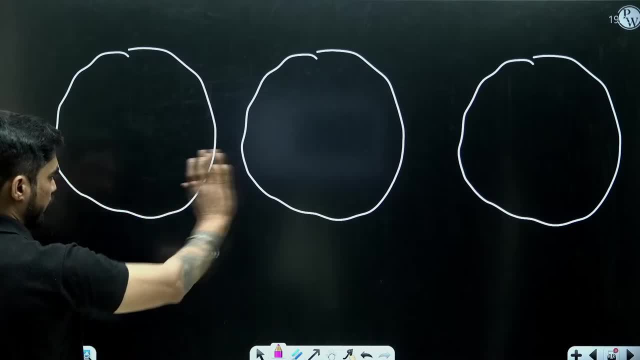 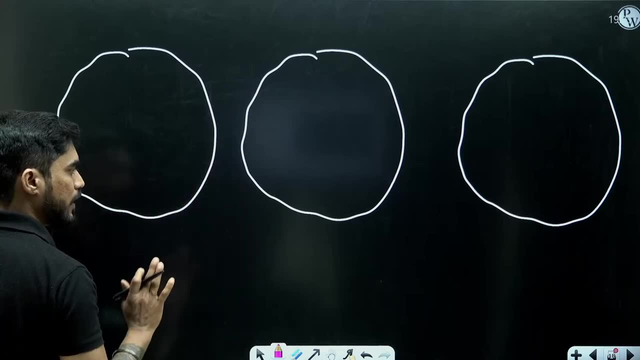 the forces must be coplanar, First of all. they should have, they should have, they should be lying in the same plane. They cannot be in different planes. If there are only three forces, there must, they must be coplanar. 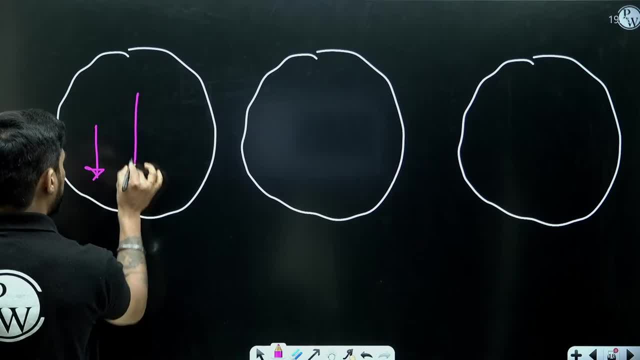 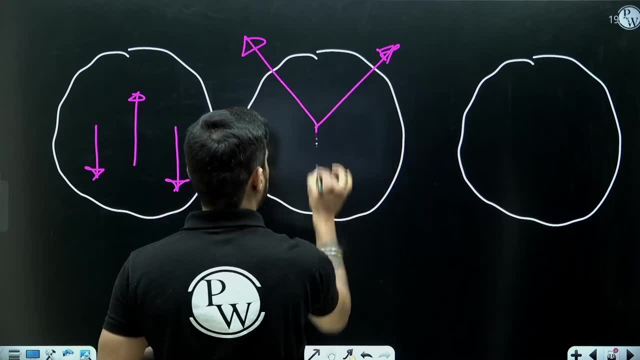 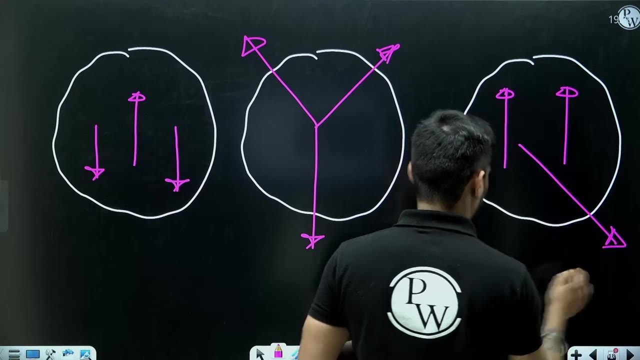 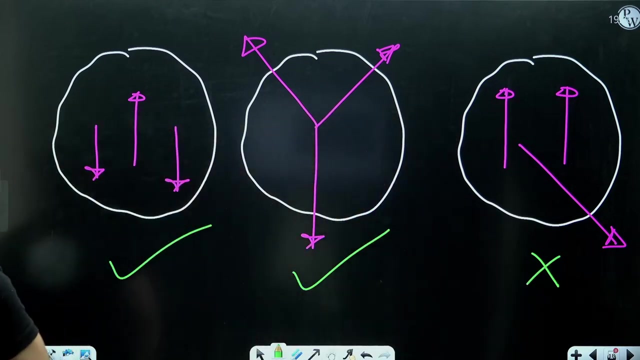 Second thing, they should either be parallel, like this, or concurrent, like this. They cannot be like this. Okay, So this is possible, this is possible, this is not possible, and this is a very interesting concept. Okay, We are going to use this concept in questions. 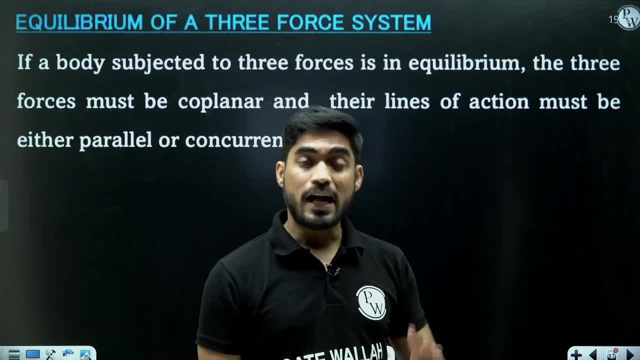 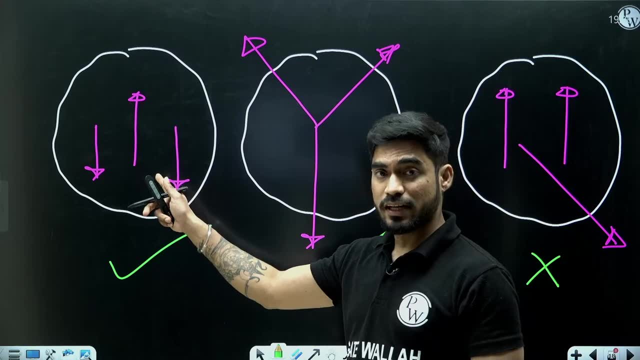 If a body is subjected to only three forces and the body is in equilibrium, the forces must be coplanar and they should be either parallel to each other or concurrent to each other. They should not. they should not be in equilibrium. They should not, they cannot be like this. 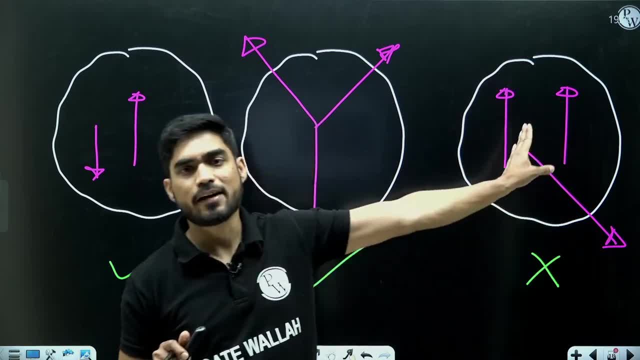 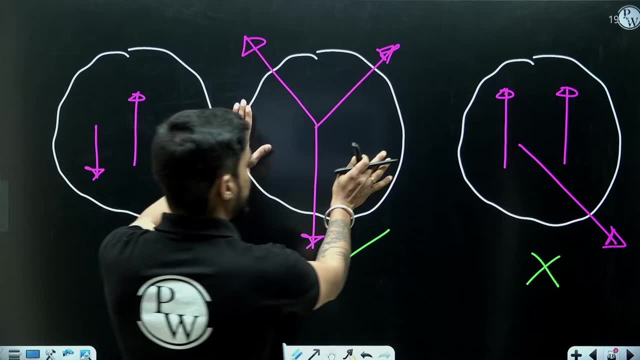 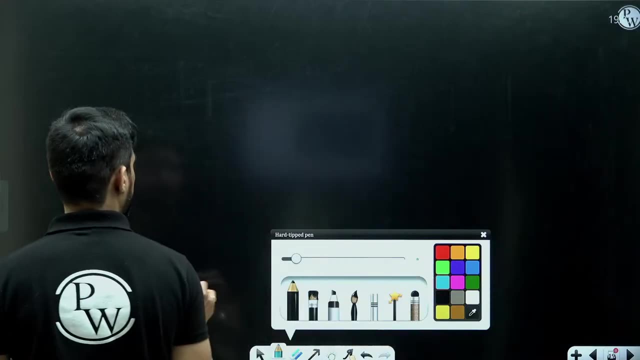 Two forces are parallel and third force is like this. This cannot happen. Okay, Now, if you get this case, then you have a very interesting theorem known as Lamy's theorem. Now, what do we mean by Lamy's theorem? understand? 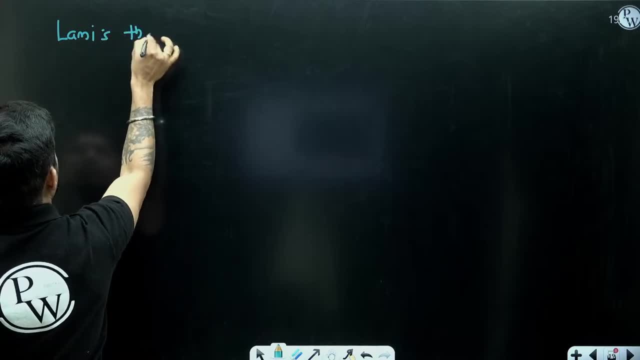 It's a very useful theorem. So let's say that a body is subjected to only three forces. Okay, So let's say that a body is subjected to only three forces. So let's say that a body is subjected to only three forces. 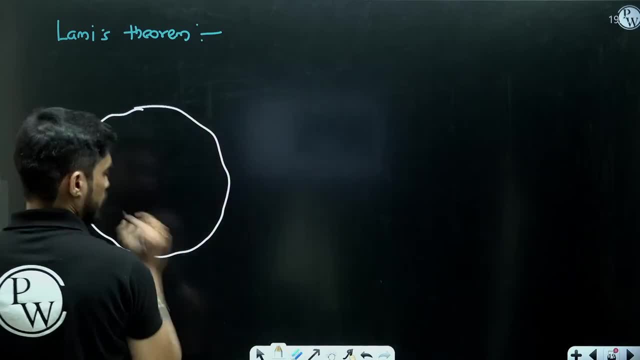 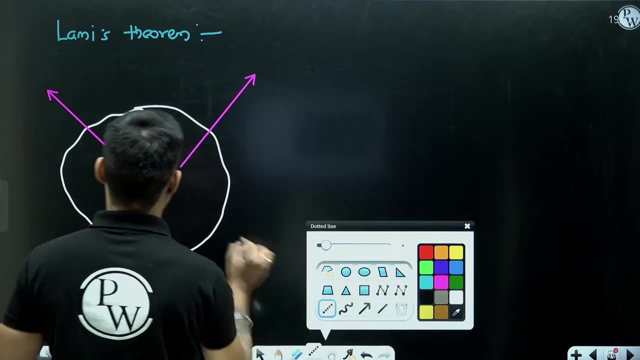 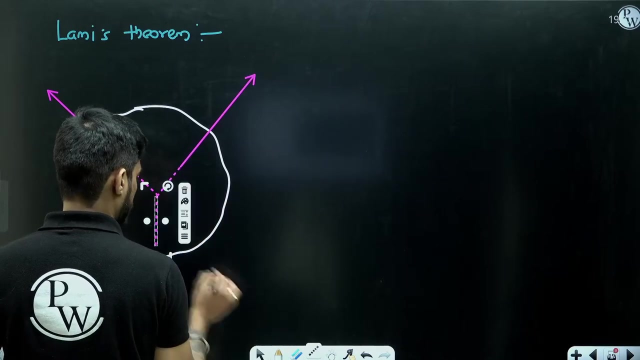 So let's say that a body is subjected to only three forces Like this. So let's say that a body is subjected to only three forces Like this. One force is like this, Other forces like this. If you extend their line of action, they will intersect. 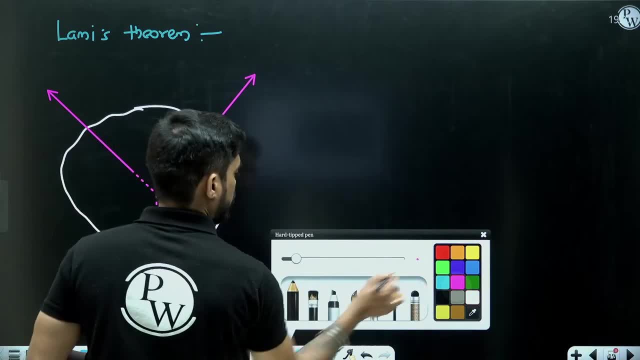 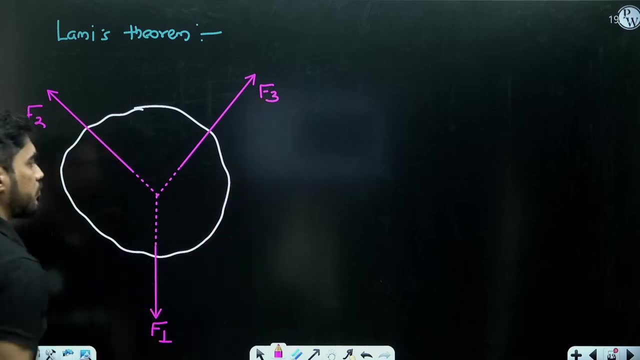 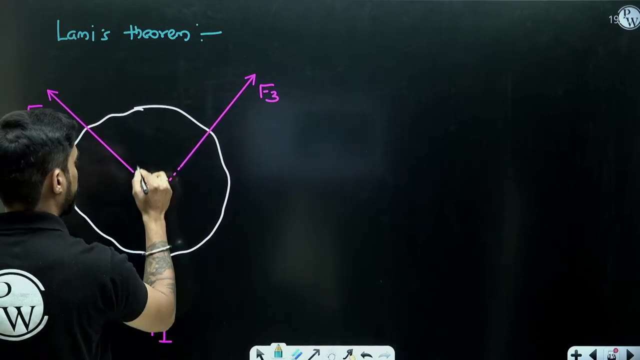 The third force is like this. Let's say: this is F1.. This is F2.. This is F3.. Okay, Let's say the angle between F2 and F3.. F2 and F3 is theta 1. The angle. 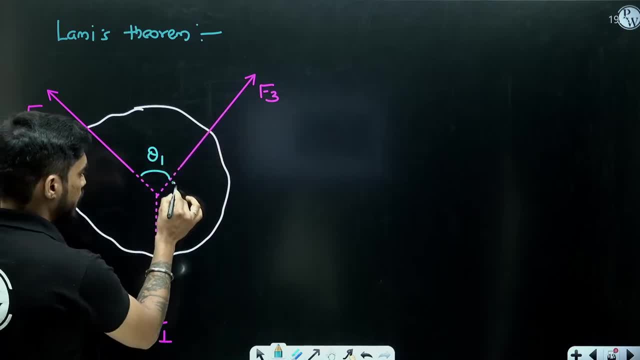 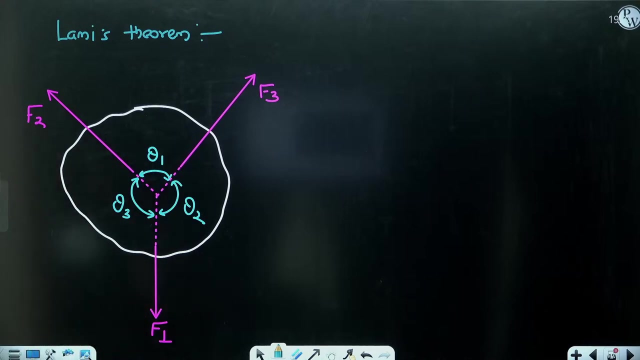 between F1 and F3 is theta 2 and the angle between F1 and F2 is theta 3.. Understand how I am taking the angles. The angle between 2 and 3 is 1.. The angle between 1 and 3 is: 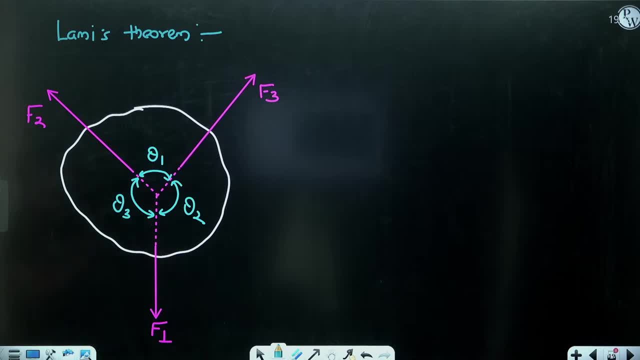 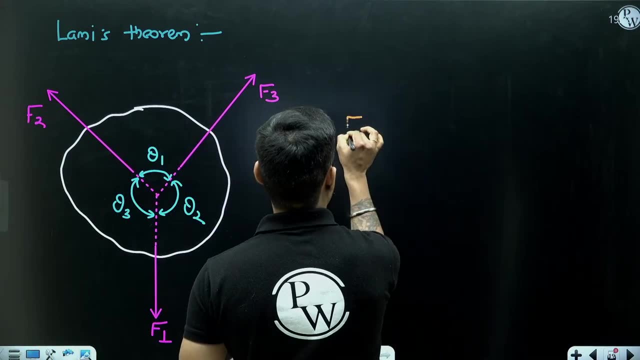 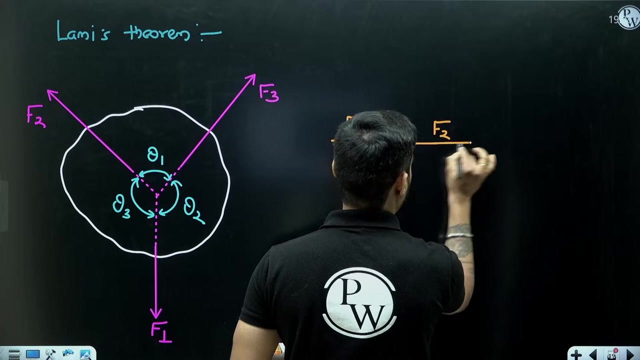 2. The angle between 3 and 1 is sorry. 1 and 2 is 3.. Now, according to Lamy's theorem, F1 divided by sine theta 1 will be equal to F2 divided by sine theta 2 will be equal. 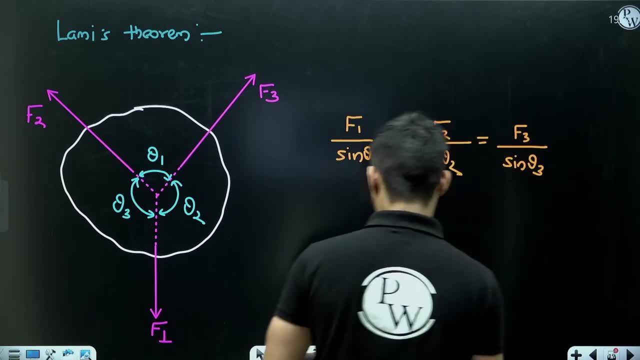 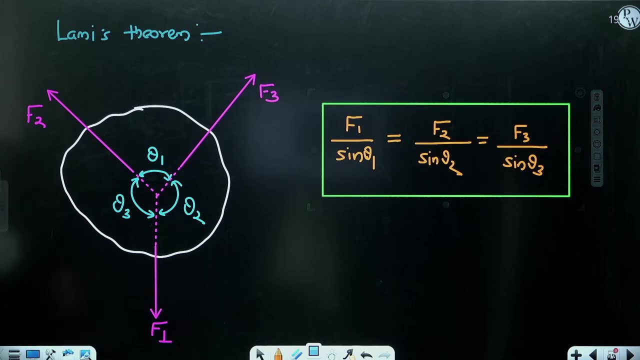 to F3 divided by sine theta 3.. This is also known as sine rule. Okay, And this is a very useful theorem whenever you have a situation like this: Okay, F1 divided by sine theta 1 will be equal to F2 divided by sine theta 2 will be equal. 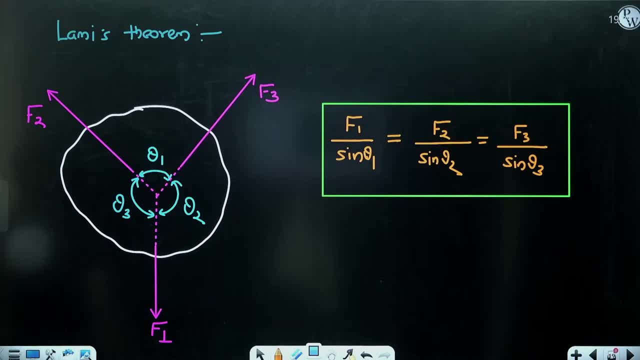 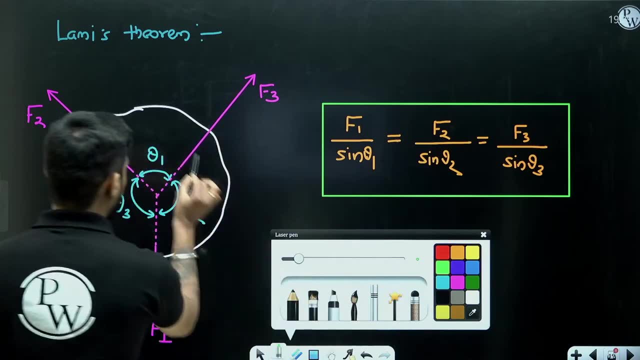 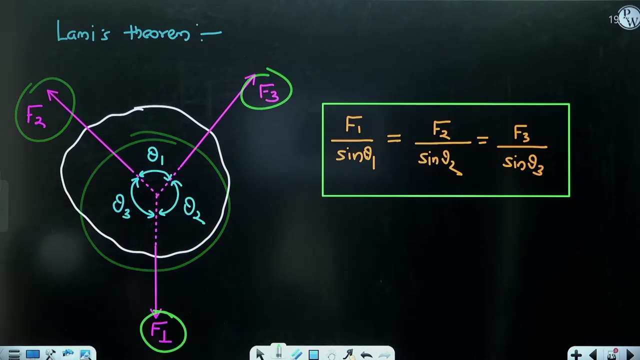 to F3, divided by sine theta 3.. Now, if you want to use this equation, you should know all these angles- theta 1, theta 2, theta 3- and you should know at least one of these forces. Okay, In order to use Lamy's theorem, to find the unknown forces, at least one force. 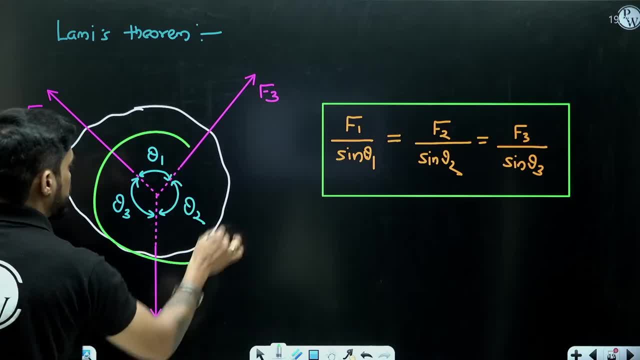 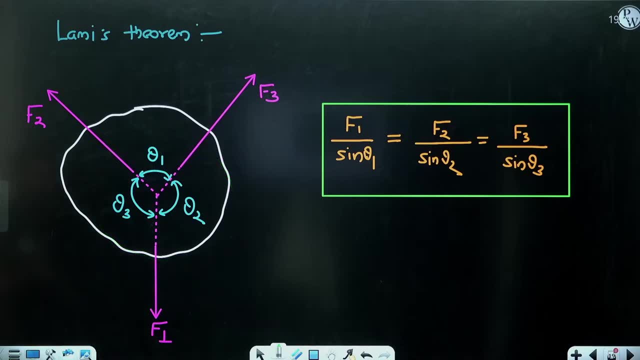 must be known. Okay, At least one force must be known. At least one force must be known, And all three angles must be known. Okay, Then only you can use this theorem to find other two forces. For example, let us say we know F2.. Let us say, we know F2 and we know: 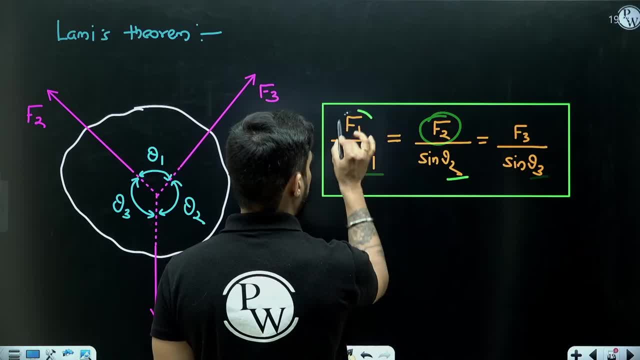 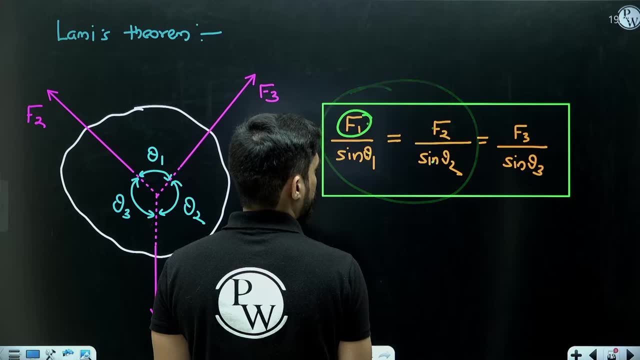 theta 1, theta 2, theta 3.. Now, in order to find F1, I will use this equation: F1 by sine theta 1 equal to F2 by sine theta 2.. And in order to calculate F3, I will use this equation: 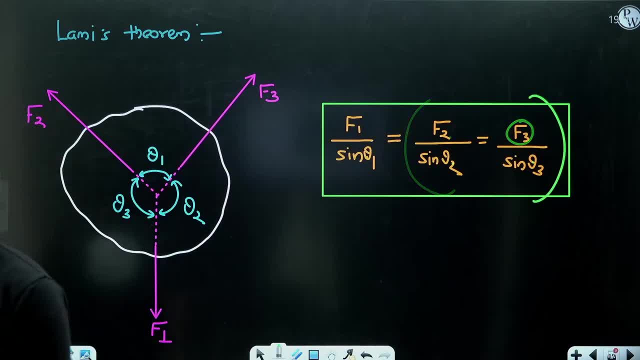 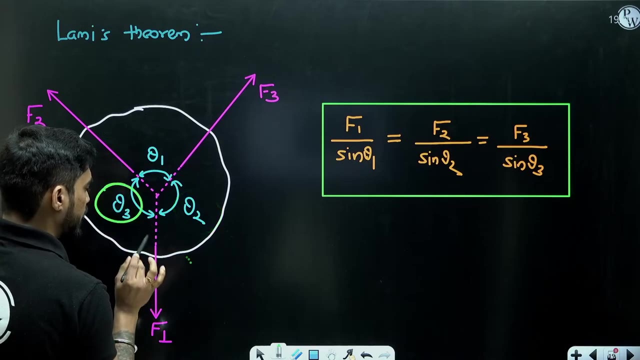 F2 by sine theta 2 equal to F3 by sine theta 3.. So at least one force must be known and all three angles must be known. Okay, And whenever you are drawing this diagram, in order to calculate the angles, you need to either draw all the forces like this coming: 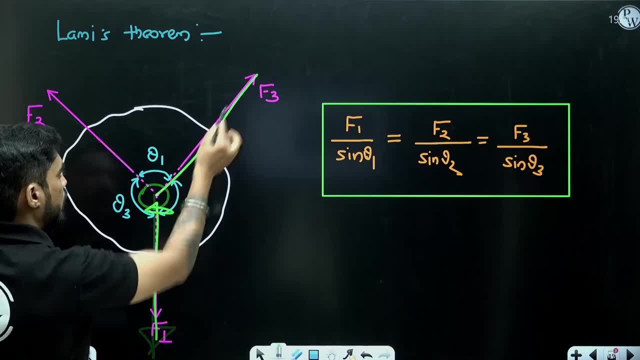 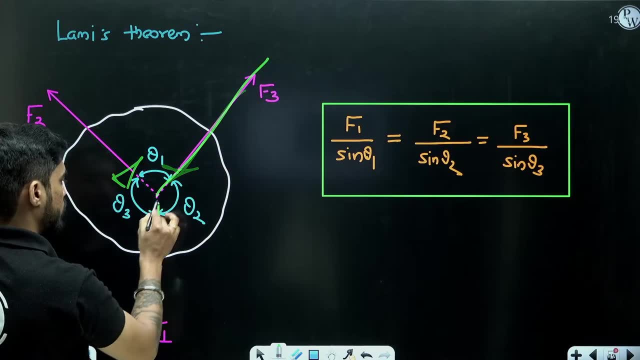 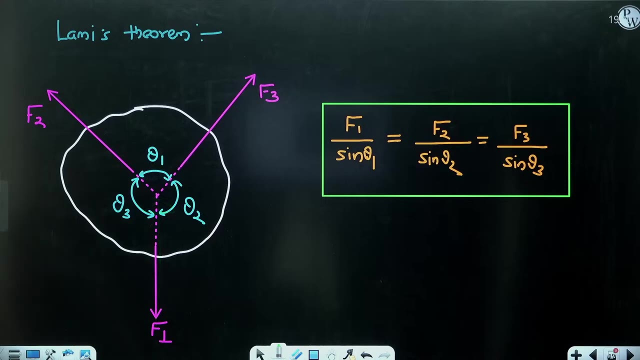 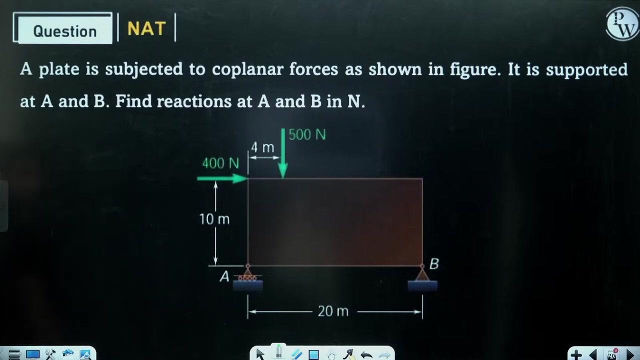 out of this point or going towards the point. like this, You cannot draw two forces towards outside and one forces towards this. Then if you calculate the angles, it will give you wrong answer. Okay, So let us solve some problems, And this is our first problem. A plate is subjected to coplanar forces as shown in figure It. 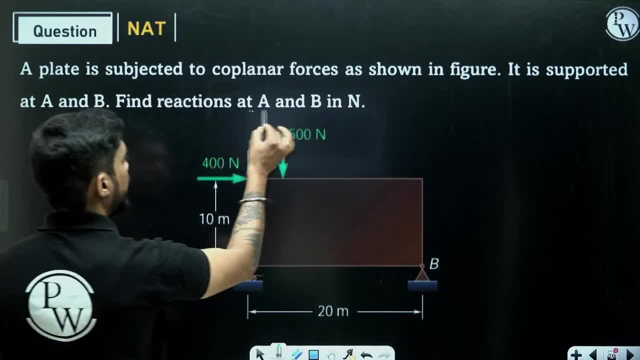 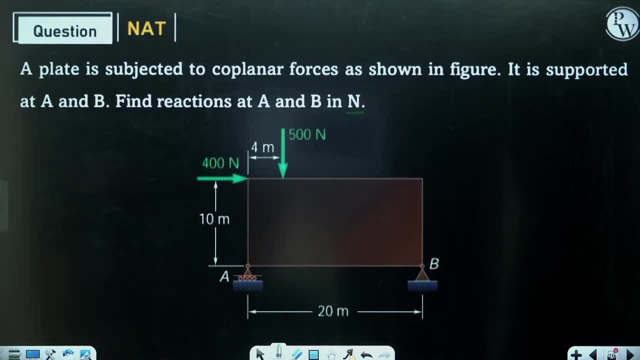 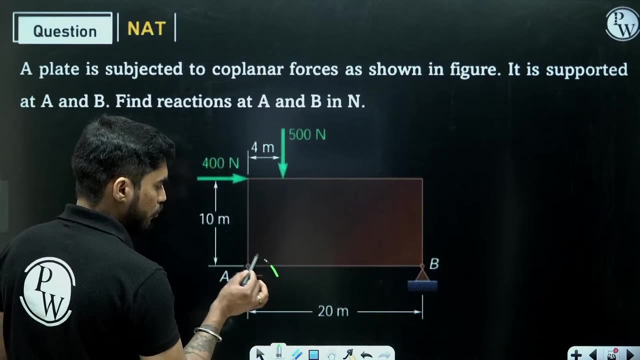 is supported at A and B. Find reactions at A and B in Newton. Okay, It is a simple problem. What is happening here? We have a plate which is subjected to coplanar forces. The plate is roller supported at A. Can you see the rollers? So here at 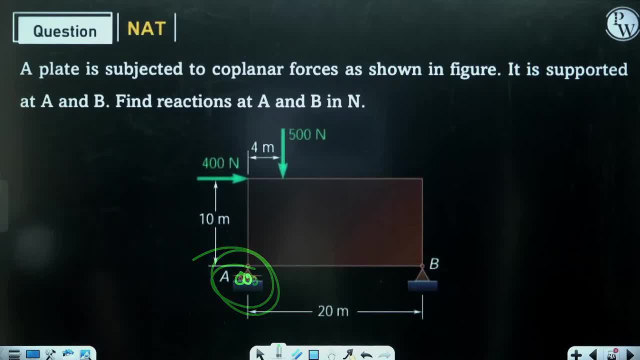 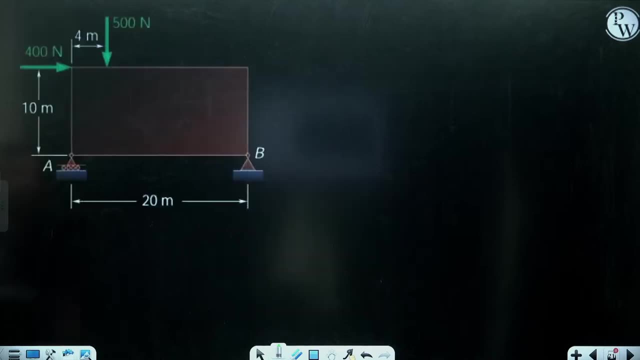 point A. we have a roller support and it is a hinge. it is it has a hinge support at B. Can you see this hinge? And now we need to find reactions at A and B, So we have a plate which is subjected to coplanar forces at A and B. Let us solve this problem Now. 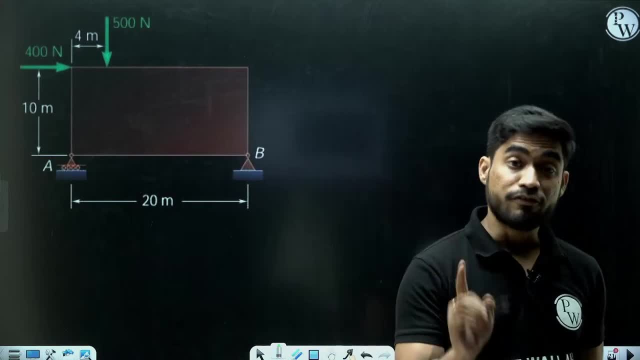 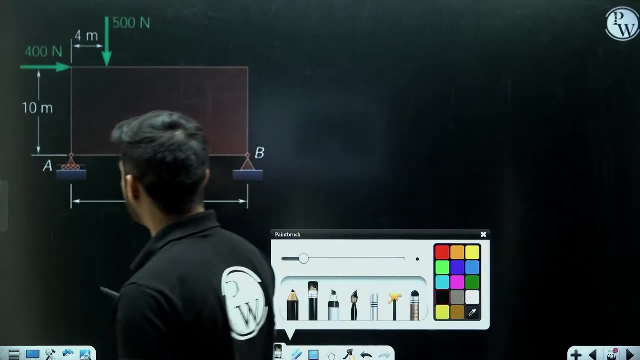 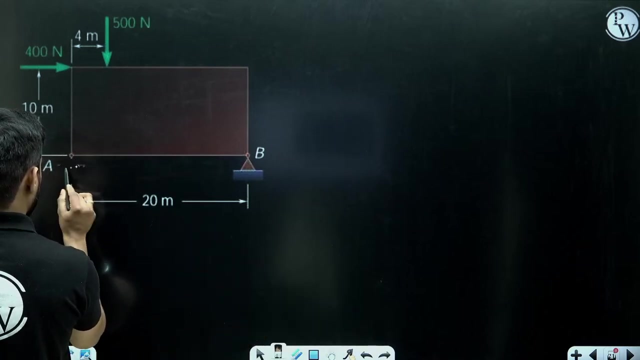 first thing you need to do is you need to draw the free body diagram. How to draw a free body diagram? You need to first remove these supports. Remove the supports Now. if you remove the support, then you need to apply the equation. So here at point A, you have a ring Teaching this example at point A. Ok, How to draw this free body diagram Is, in this case: grab the edge of the Creek Port to the corresponding angle. How to do this, There is going to be pawn here: How to draw this free body diagram With this side, change the. 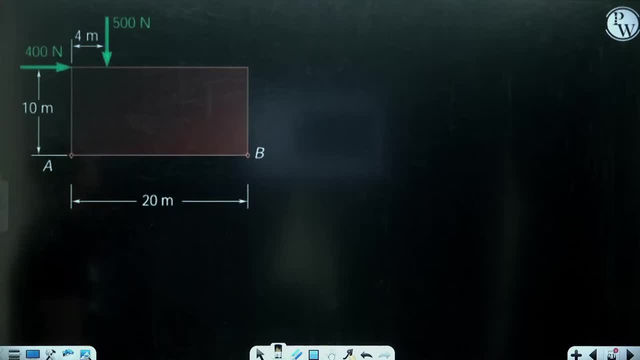 goes in to the right way Because my sleeve aims so the weight depend on the right region, at the 90 degree. Now, if you remove the, it goes to the right. Now, if you remove the, remove the support, then you need to apply the reactions, proper reactions If you remove. 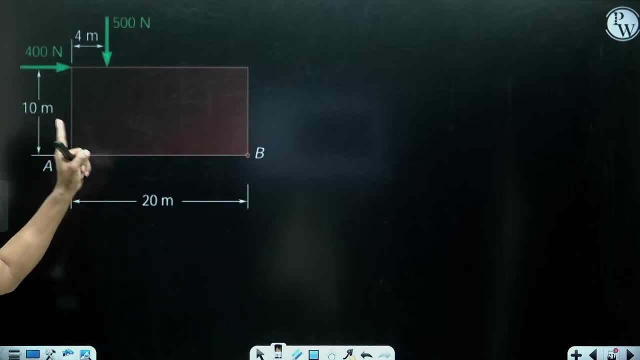 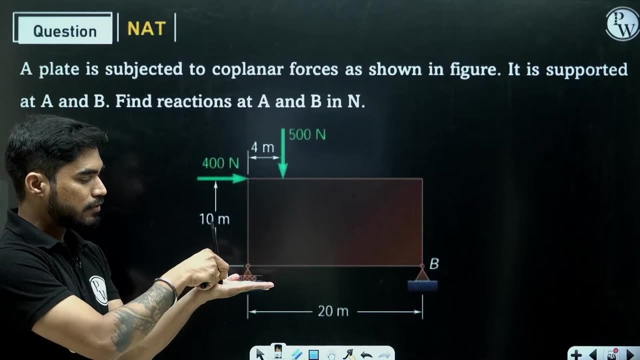 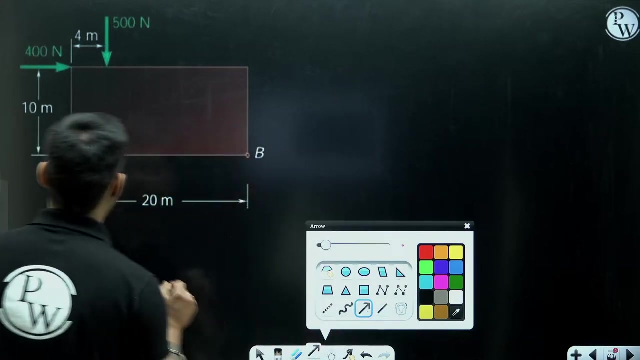 the roller support, you will have to apply a reaction normal to the surface of roller. So this is the surface of roller. So the force, the reaction force, must be normal to it. It can be in plus y or minus y direction, it is up to you. So I will assume that the 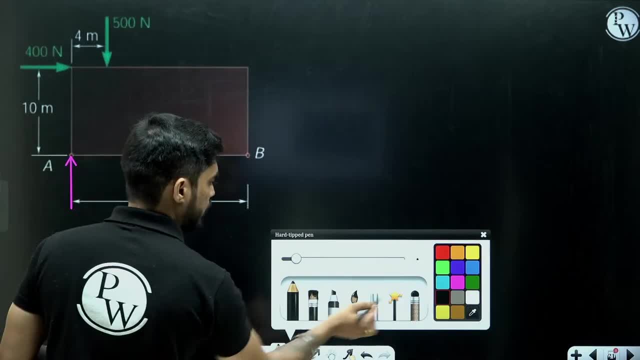 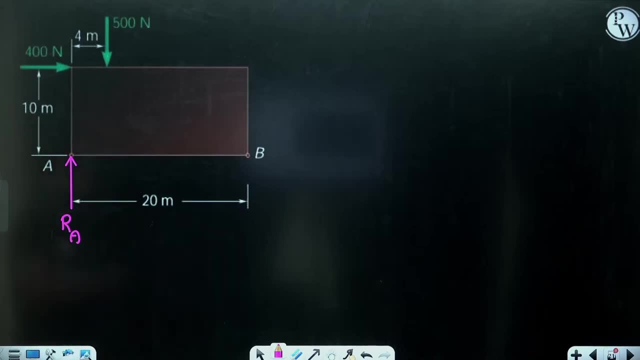 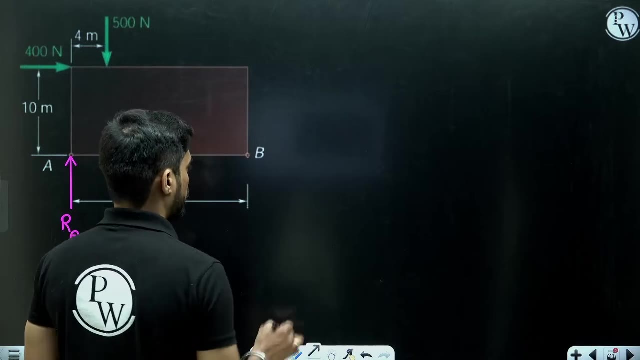 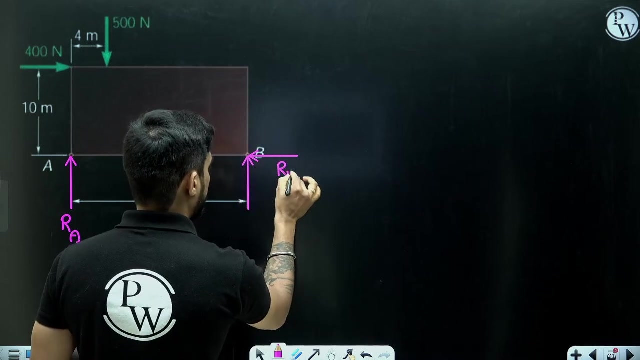 reaction force at A is upward. Let me call it RA. Now, at point B, we have a hinge support. So if you remove the hinge support, you will have to use two reactions, One like this, one like this. I will call it RBX. I will call it RBY. Now you can see. 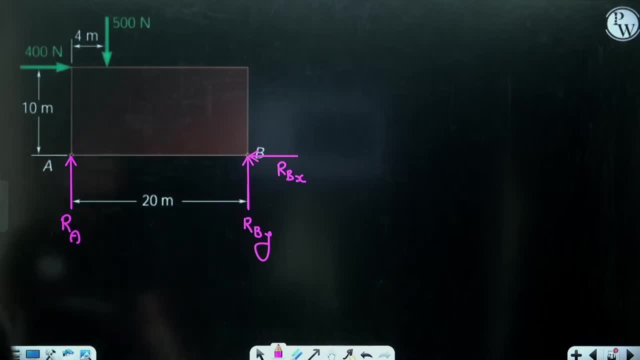 this is the free body diagram of the plate. What is this? This is free body diagram, also known as FBD. So we have isolated the body from all the other bodies. Now, how many unknowns do you see here? You see three unknowns. So you see three unknowns. So you see three unknowns, So you see. 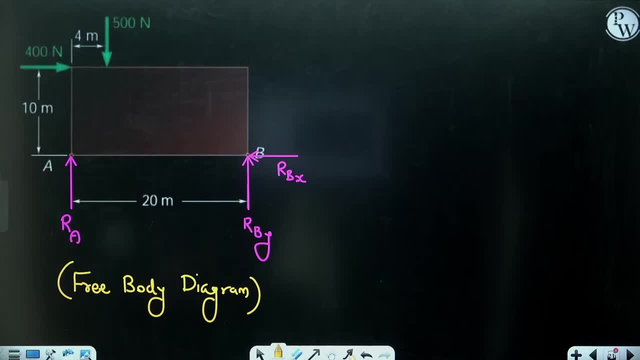 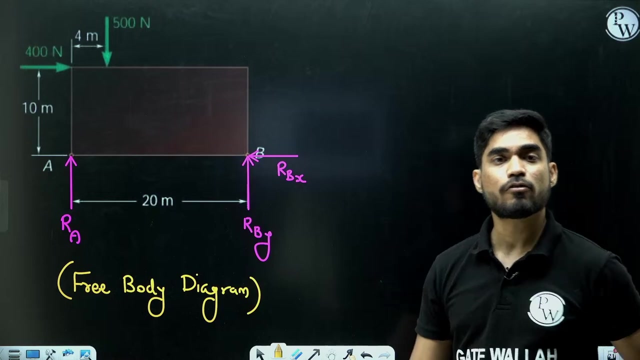 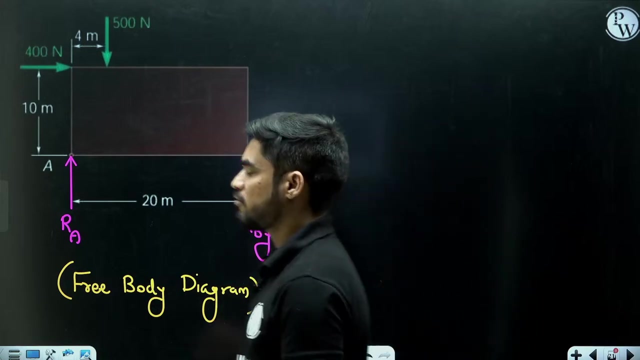 three unknowns: RA, RBX and RBY. And how many equilibrium equations do you have? You have three equilibrium equations. You can use all these three equilibrium equations and you can find these unknown forces. Let me use the third equation first. I will apply the moment equation first. 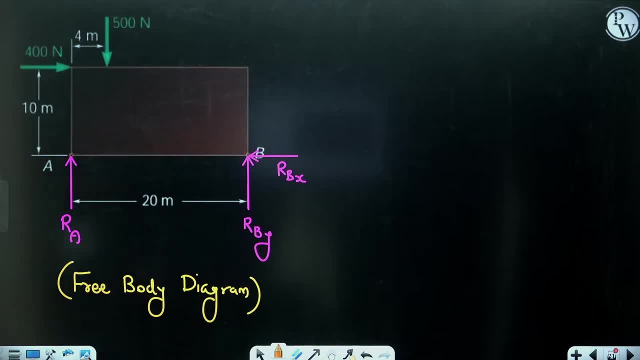 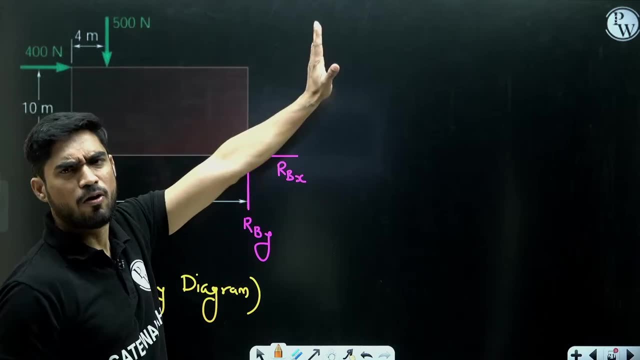 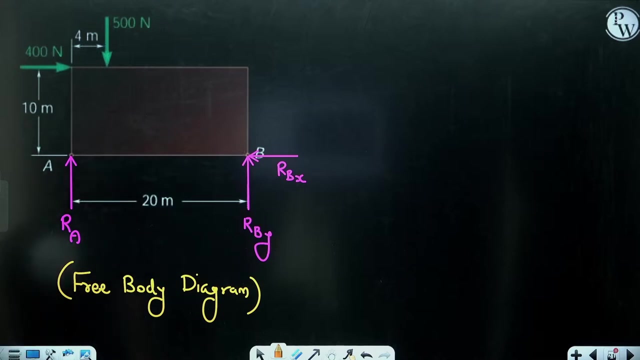 Now where I will take moment. You can take moment. you can take moment about any point. You can take moment about any point inside or outside the body, doesn't matter. But here I will take moment at B. Why I will take moment at B? Because if I take 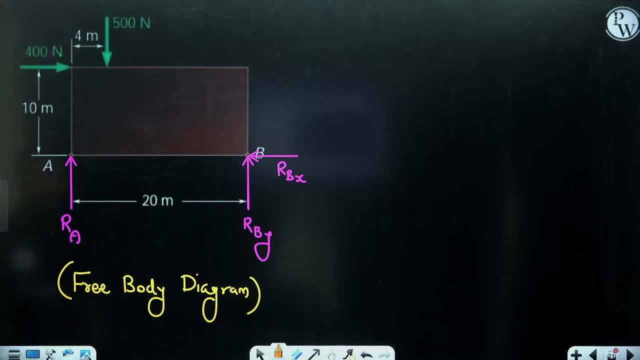 moment at B, the moment of RBX and RBY will be 0.. I will get the moment of RA, this 400 newton, this 500 newton, So there will. there will be only one unknown in the equation, RA. So I will get the value of RA, So I will apply. 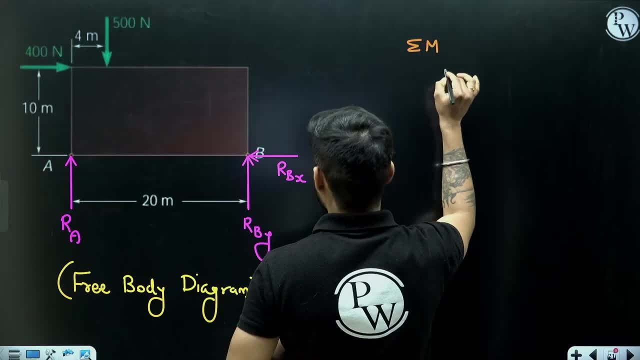 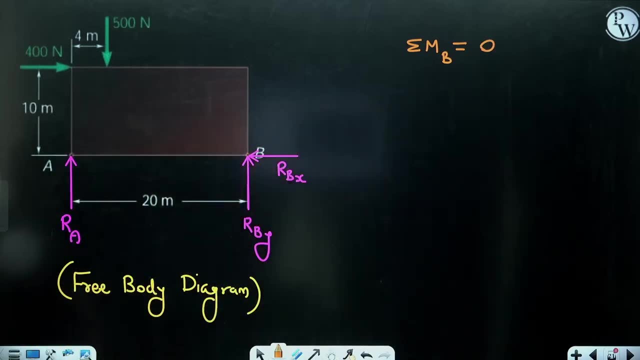 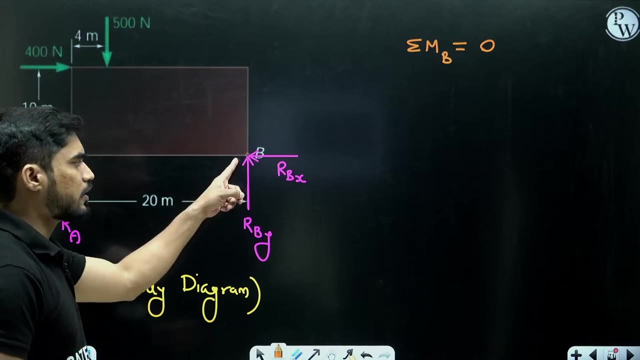 this equation, Net moment at point B equal to 0.. You can take moment about any point. Net moment about any point must be 0. But if you take moment about B, you will have the advantage of getting the moment of RBX and RBY 0.. 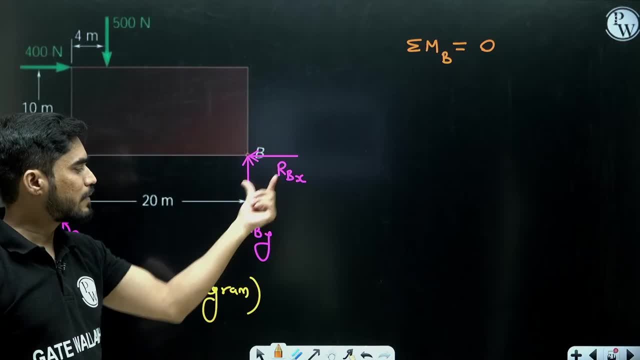 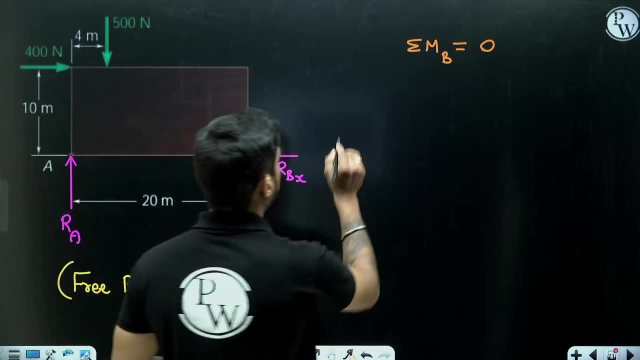 So net moment at point B equal to 0.. So moment of RBX and RBY will be 0 because they are acting at B. Moment of RA will be clockwise. What will be the moment RA into 20.? It will be clockwise. 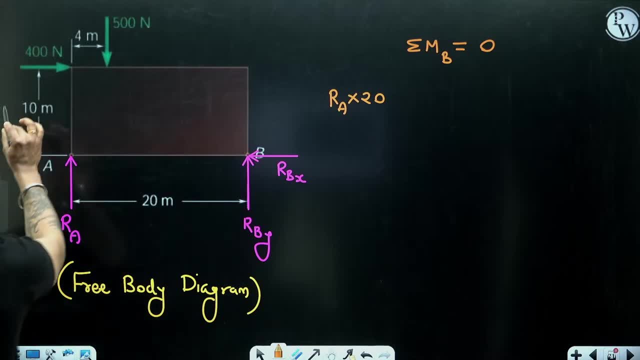 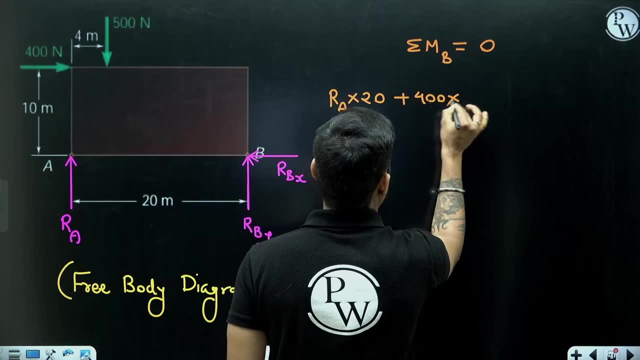 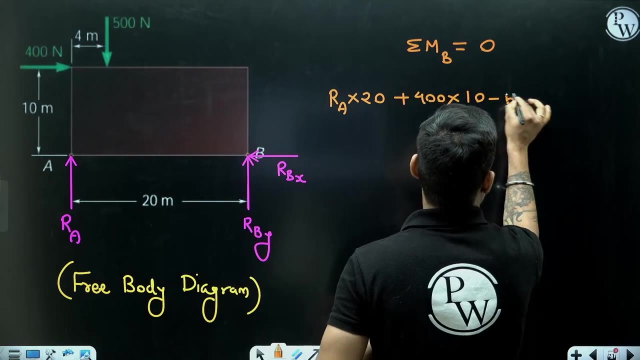 Now, moment of this 400 newton will also be clockwise. Moment of this 400 newton will also be clockwise, Plus 400 into 10. But the moment of 500 newton will be anti-clockwise. So minus 500 multiplied by this will be. 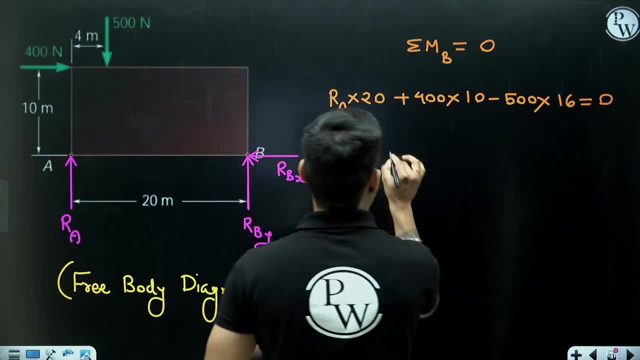 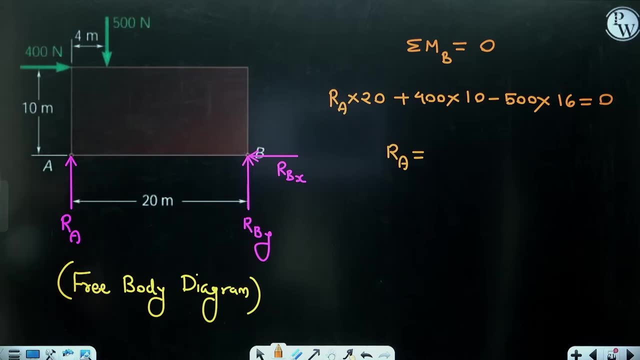 16.. So from here I will get the value of RA. There is only one unknown See. So 500 into 16, minus 400 into 10.. 4000 divided by 20.. So I am getting RA equal to 20.. The moment. at point B, equal to 0.. I will take the new moment at point B. The moment of this 400 newton will also be counterclockwise: 500 into 10 minus 400 into 10.. So I will take the new moment. 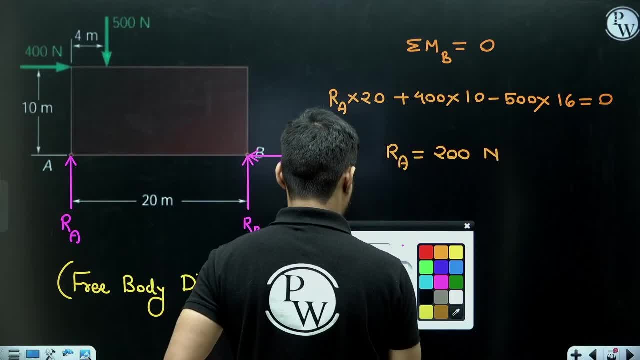 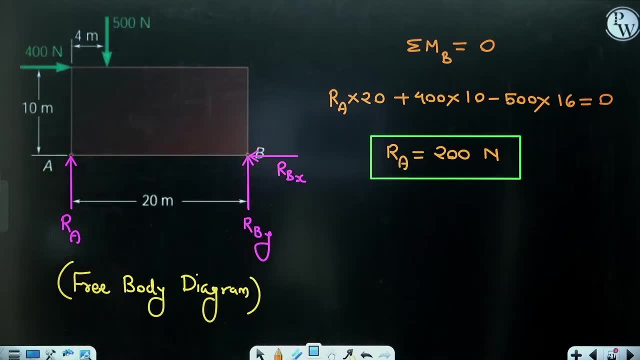 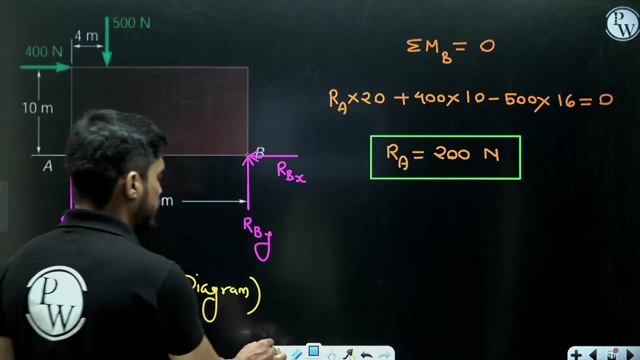 of this 500 newton. That is it The moment at point B- equal to 0. So I will take the new moment, Ra equal to 200 Newton. So I have got Ra, 200 Newton. Now I will calculate Rbx by applying. 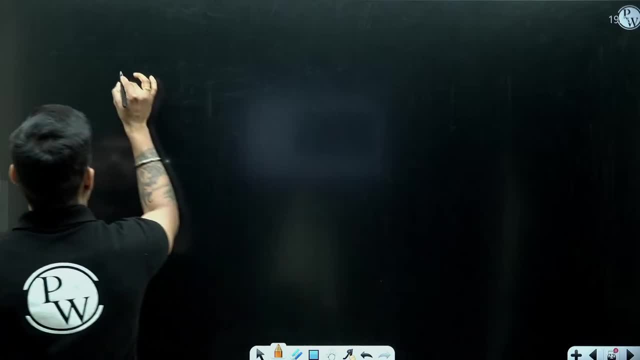 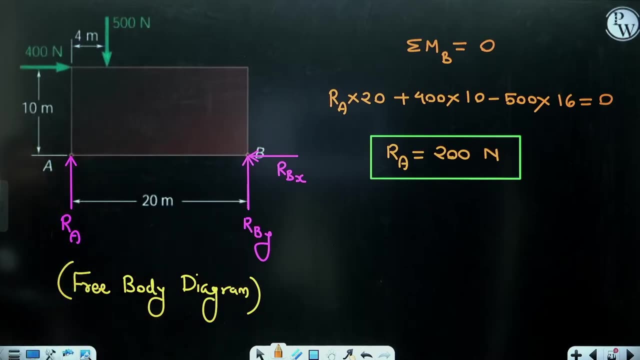 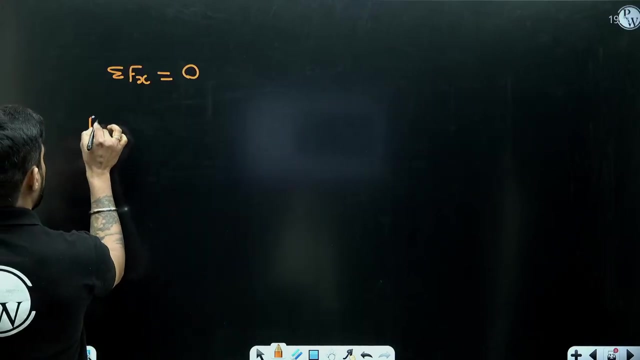 the second equilibrium equation. So I will apply summation of- sorry, first equilibrium equation. summation of Fx equals to 0.. So you can see that in x direction you have two forces, 400 and Rbx. So I can write this: Rbx equal to 400 Newton, because both must. 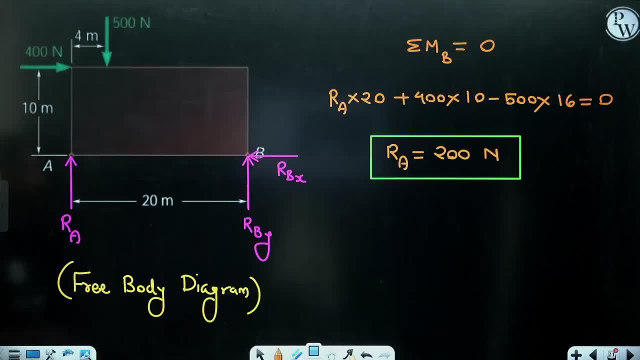 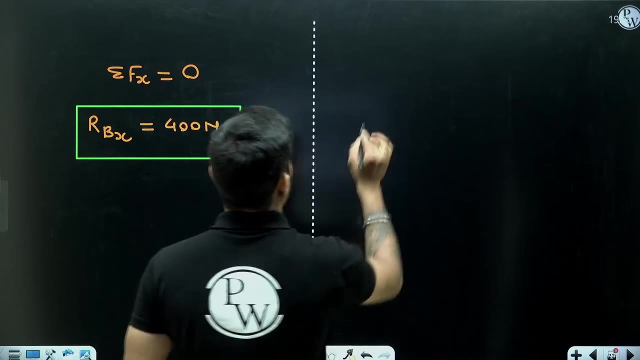 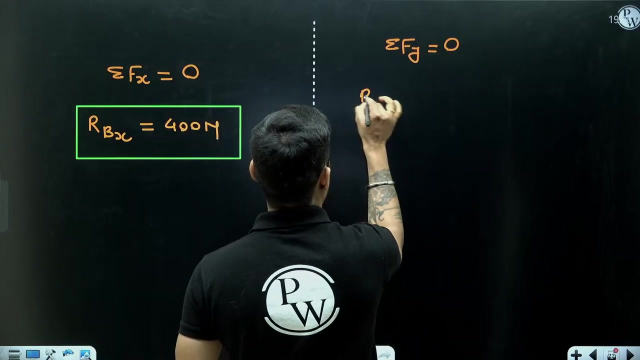 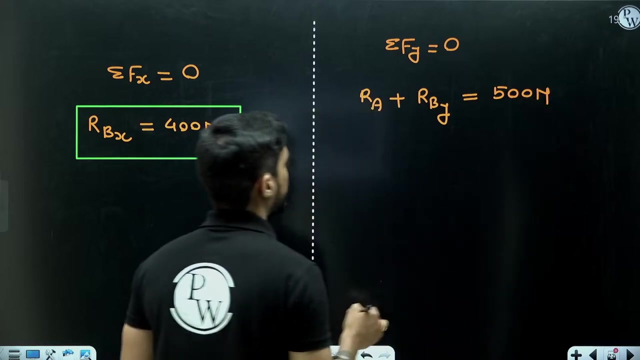 be equal and opposite. Then only net force in x will be 0. So Rbx will be equal to 400 Newton. Now how do we calculate Rby? Summation of Fy equal to 0. So I will get Ra plus Rby equal to 500 Newton And Ra is: 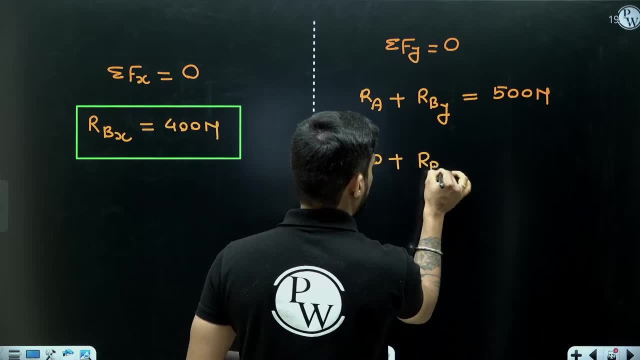 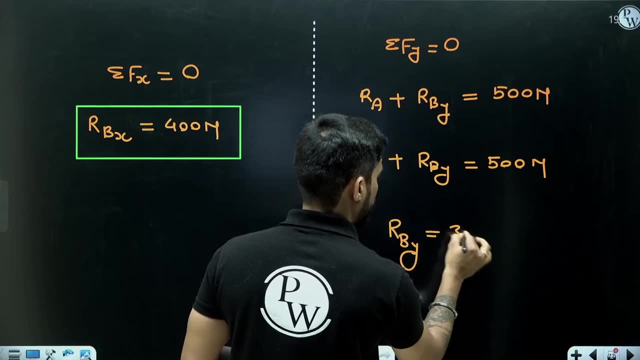 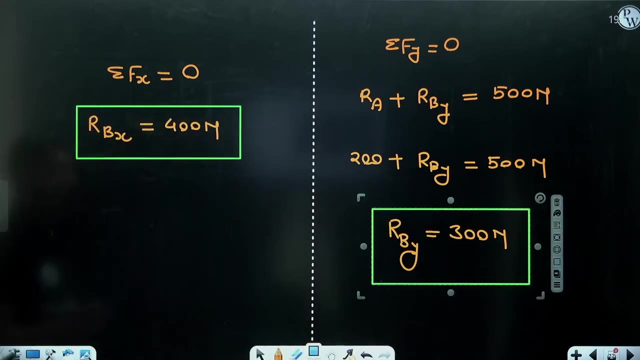 how much? 200 Newton. So 200 plus Rby equal to 500 Newton. So Rby will be equal to 400 Newton. So I have got Rby also Now. if you want, you can take the resultant of Rbx. 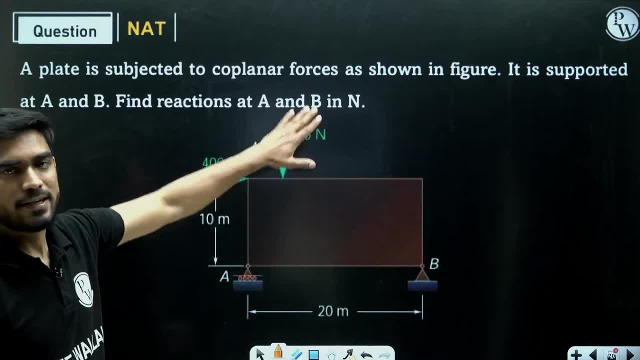 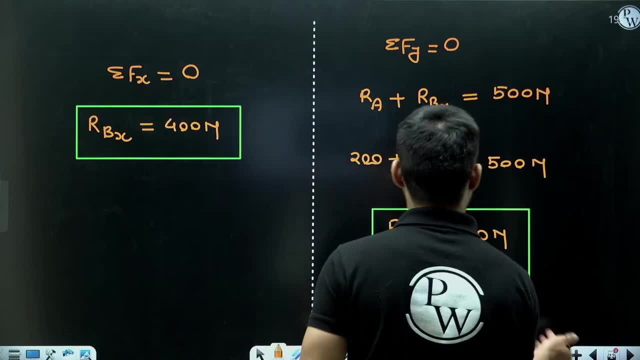 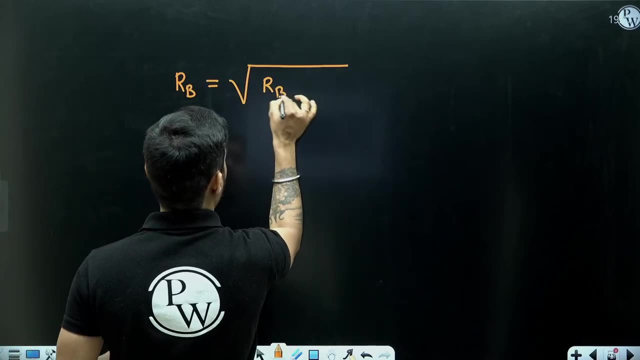 and Rby. Now, although it is not clear in this question whether you need to find components of Rb or the resultant of Rbx and Rby, Let us calculate the resultant In GATE. they will tell you whether you need to find the components or you need to find the resultant. 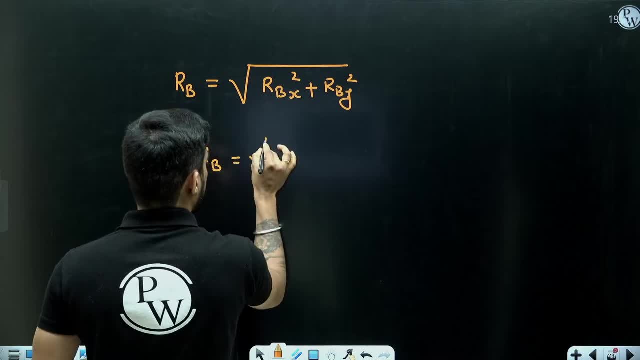 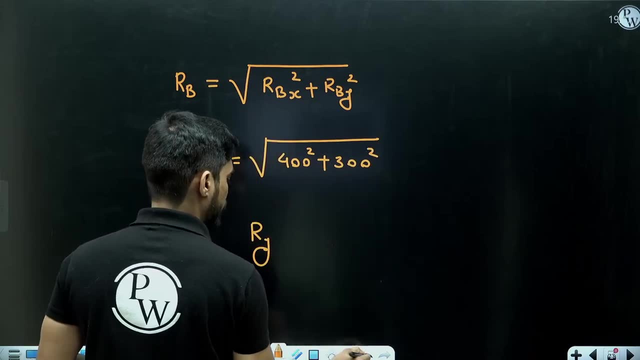 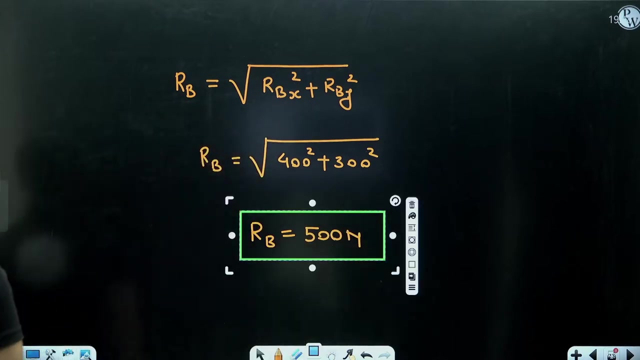 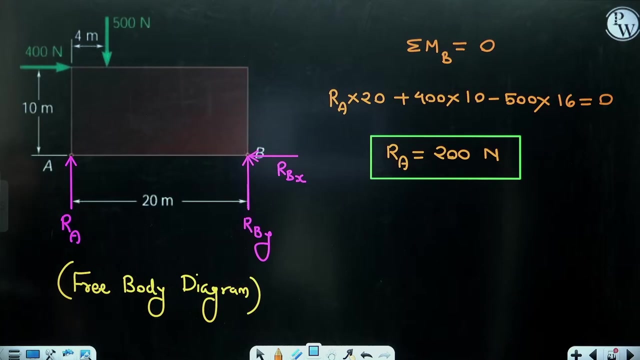 Here I have not mentioned. So it will be 400 square plus 300 square, So Rb will be 500 Newton. Very good, Sanjay, Very good. Rb is 500 Newton and Ra is 200 Newton. So 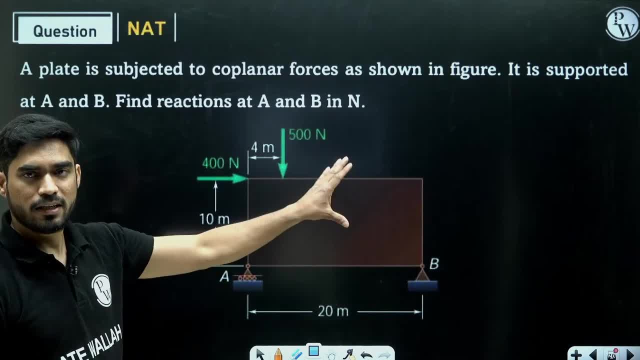 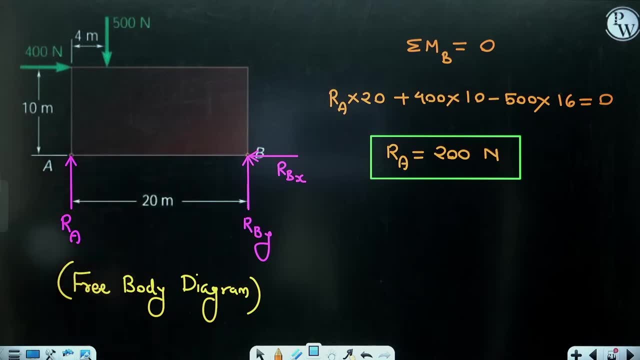 understand this procedure. First, I isolated the body from the surface. So I isolated the body from the surface. So I isolated the body from the surface. So I isolated the supports. Then I applied the reactions, Then I applied the equilibrium equations. 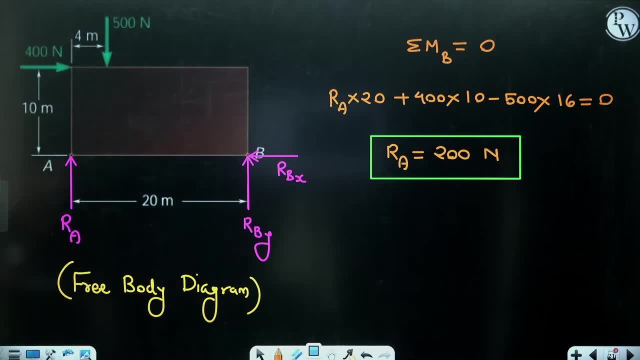 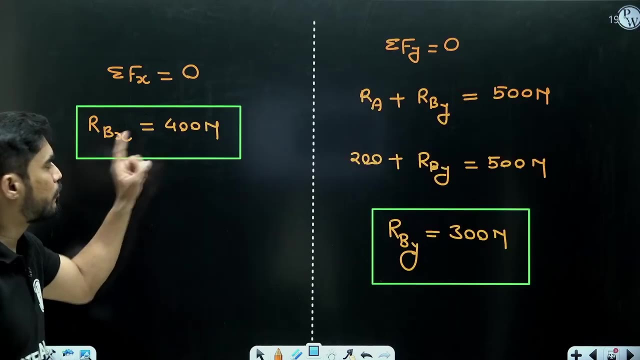 START xy NG p T sq 집 and Nw p θ sq74, solve the equations. found the values. Now look at the values. All the values I am getting are positive. It means that my directions were correct. Let us say you are assuming RbX to be like this, Then here you will get. 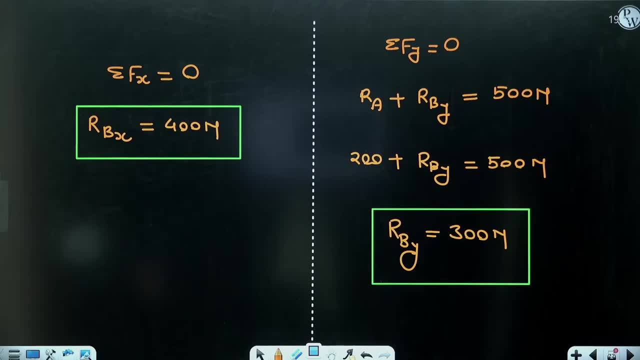 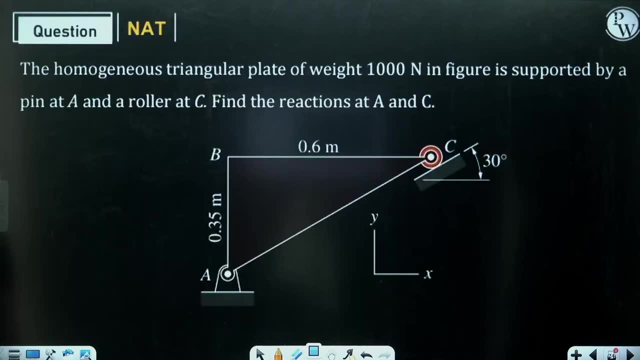 –400 means your direction is wrong. Let's solve another question, solve this one. This is an interesting one. The homogeneous triangular plate of weight 1000 Newton is supported by a pin at A and a roller at C. Find the reactions at A and C. 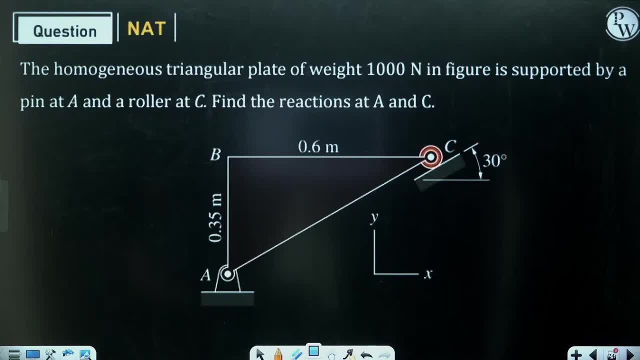 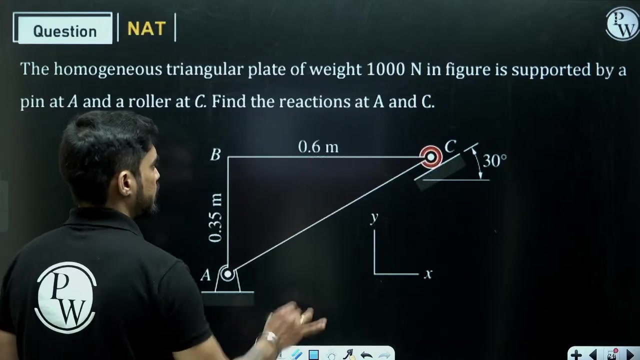 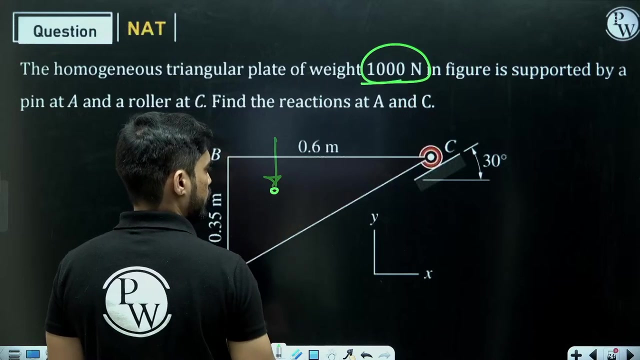 So we have a triangular plate which is hinged at A and there is a roller at C. The plate has a weight of 1000 Newton. It is homogeneous means the weight is equally distributed. It means we can assume the weight to be acting at the centroid of this plate. 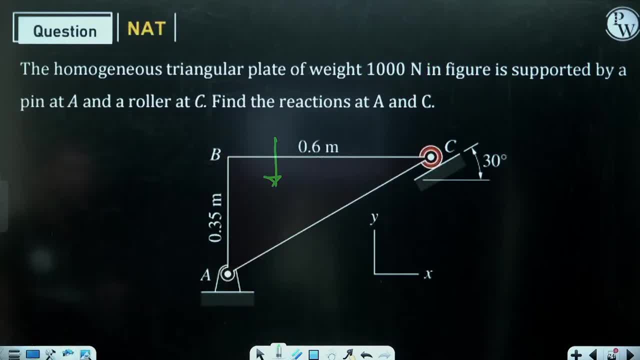 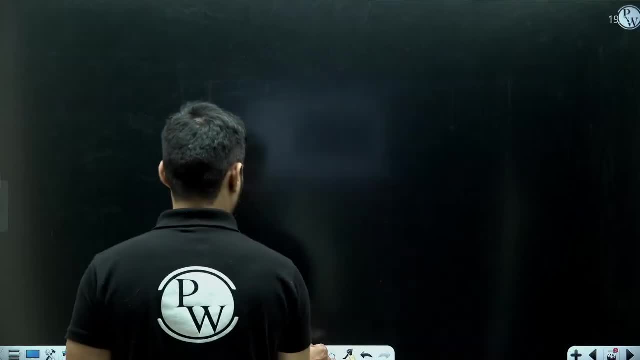 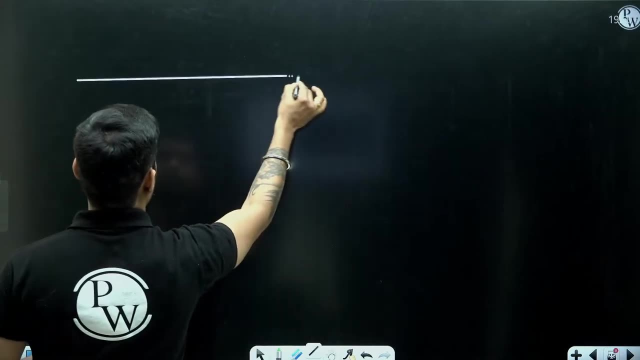 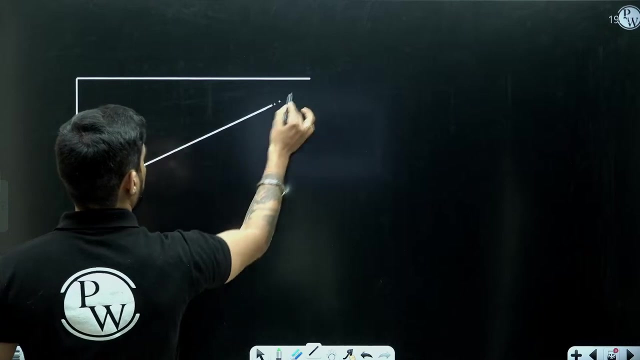 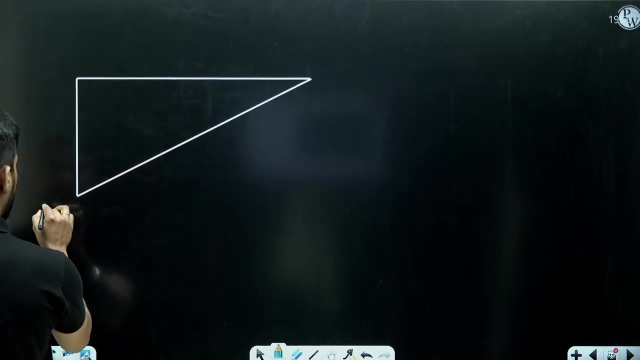 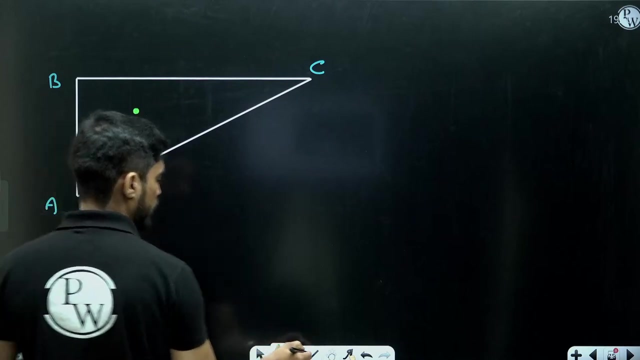 Now I have to draw the FBD of this plate. Look at the FBD. The plate is something like this: This is A, this is B, this is C. Now where will be the centroid of this triangular plate? Centroid of the triangular plate will be somewhere here. 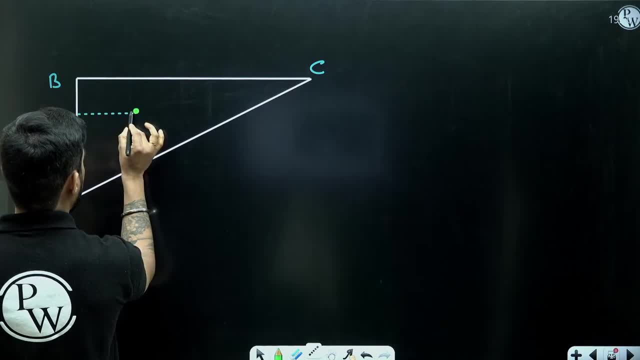 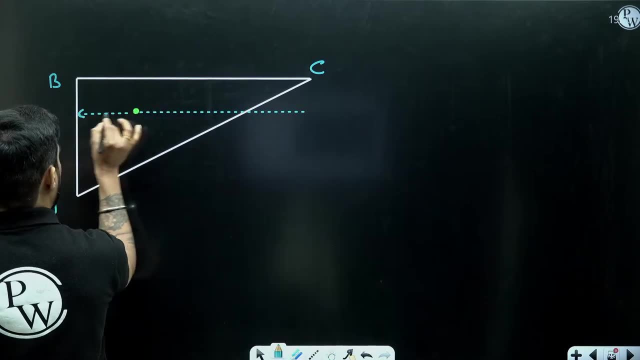 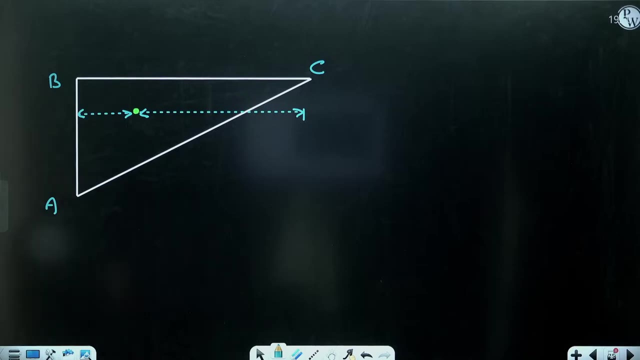 L by 3 from here And 2L by 3 from here. If you don't know about centroid, don't worry, I will take a special class. I will take a lecture on centroid also, So don't worry about it. 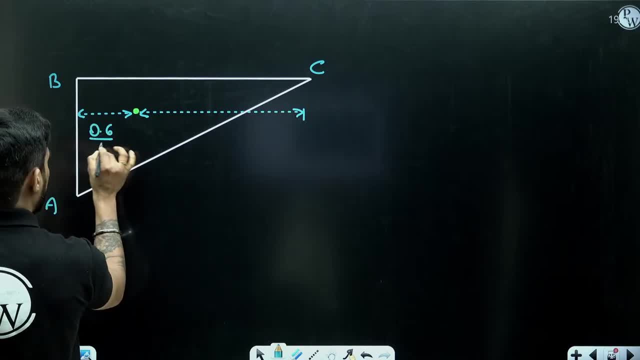 So this will be 0.6 by 3 and this will be 2 into 0.6 by 3.. Okay, So the weight of 1000 Newton will be 0.6 by 3.. So the weight of 1000 will be acting here. 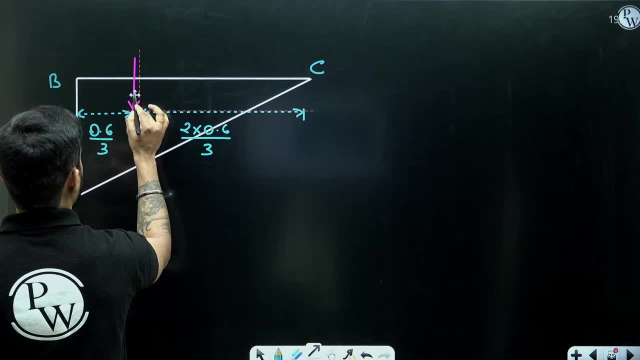 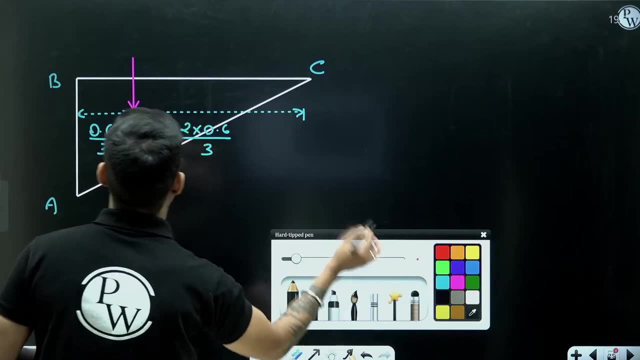 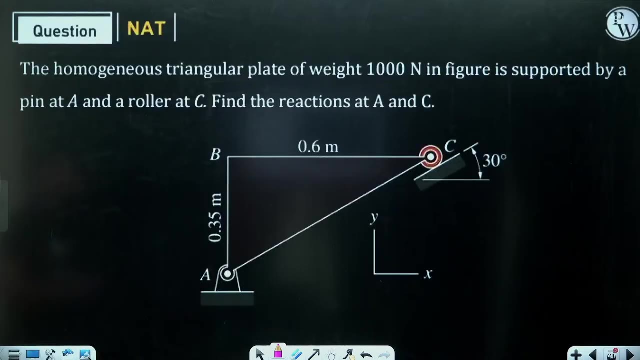 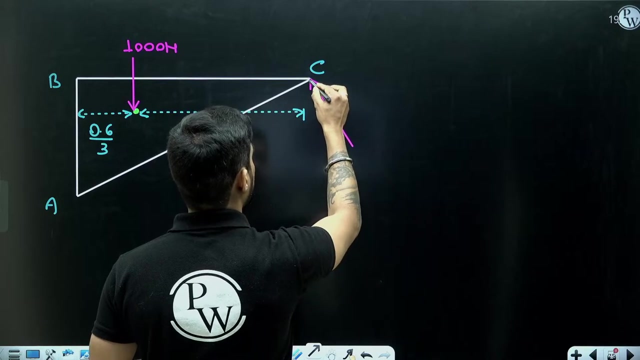 Now there is a roller support at C, So the reaction at the roller will be normal to the surface like this. Now understand this very important thing. This surface is making 30 degree with horizontal. This is the surface and it is making 30 degree with horizontal. 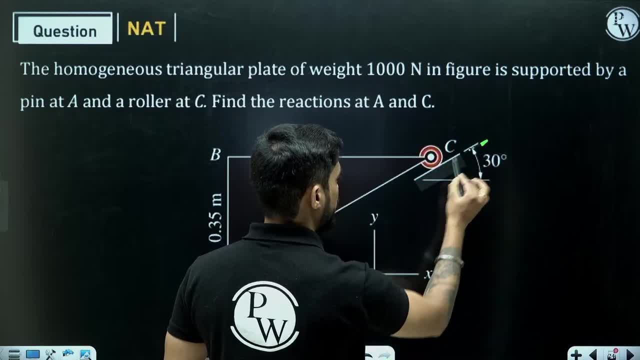 So the reaction which is normal to the surface, the reaction will be normal to the surface, It will make 60 degree with horizontal. The surface is making 30 degree with horizontal. So the reaction which is normal to this surface: it will make 60 degree with horizontal. 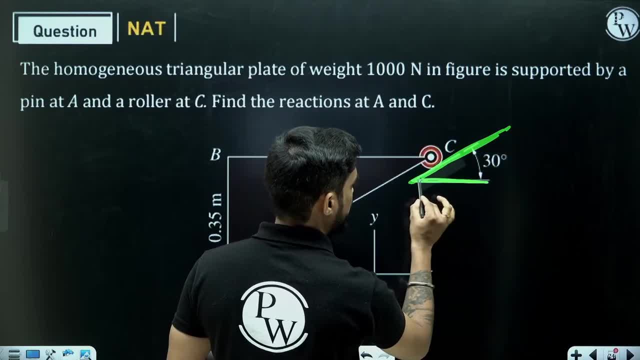 The surface is making 30 degree with horizontal. So the reaction which is normal to this surface: it will make 60 degree with horizontal. The surface is making 30 degree with horizontal, So the reaction which is normal to this surface: it will make 60 degree with horizontal. 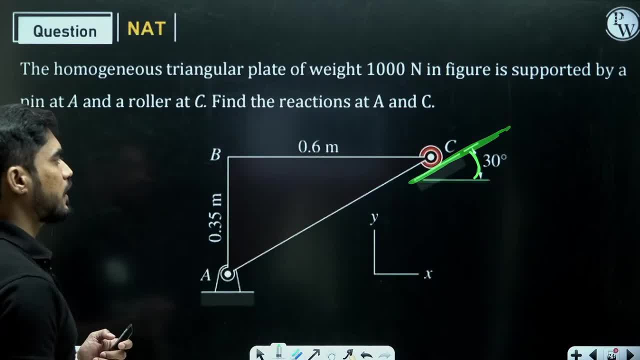 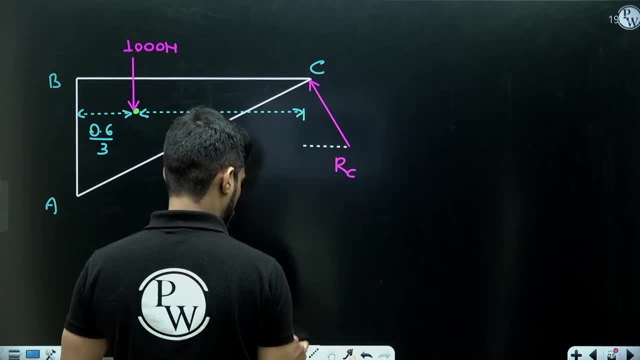 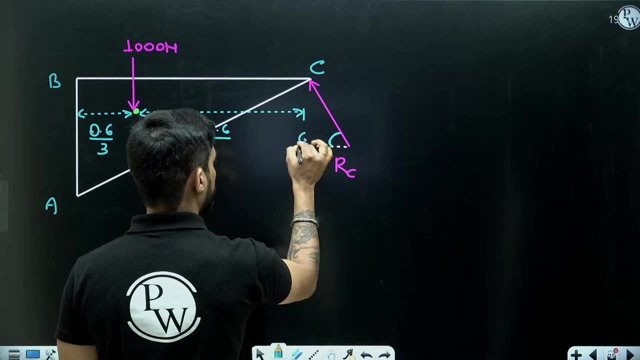 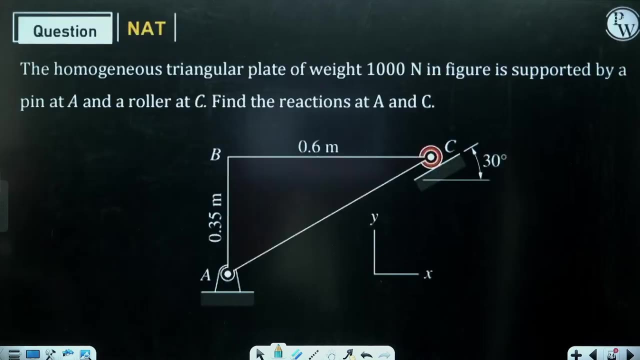 So the reaction which is normal to this surface, it will make 60 degree with horizontal. So this angle will be 60 degree. normal to the surface Surface was making 30 with horizontal, so the reaction is making 60 with horizontal. 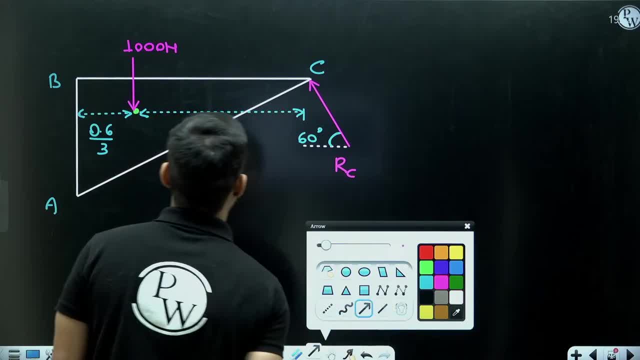 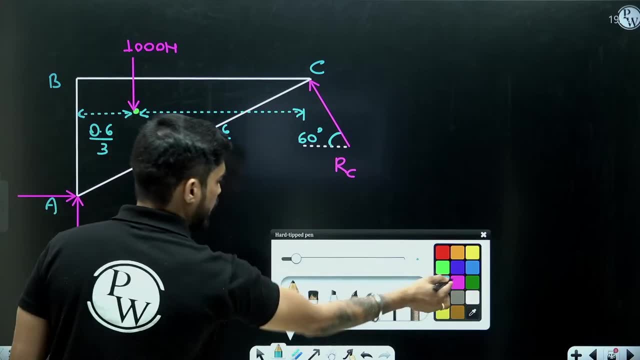 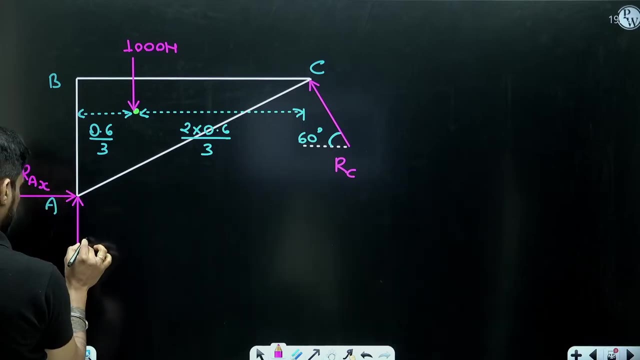 Now at point A, you will have two reactions. One is: let us say like this. another one is: let us say like this: This is just my assumption. I do not know whether the x? wala reaction will be in this direction or this direction. 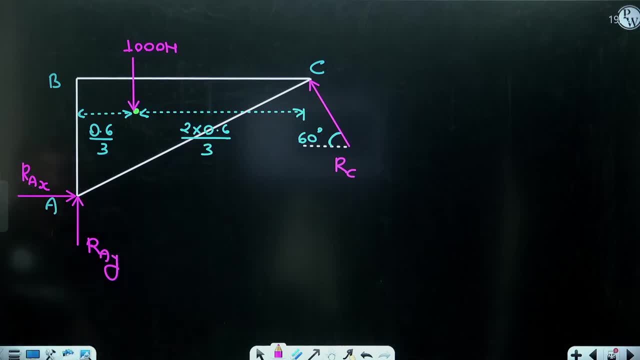 I have just assumed it. So Ra x, Ra y. Now, how many unknowns do we have? Again, we have three unknowns: Ra x, Ra, y and R c. So again, we have three equilibrium equations. Now which equilibrium equation are we going to use first? 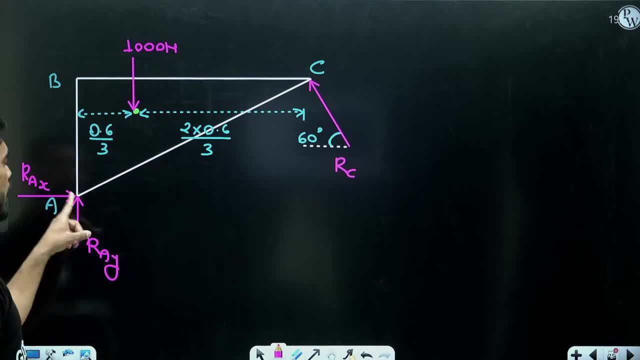 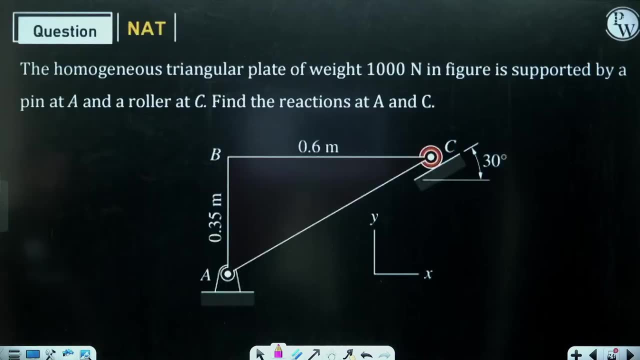 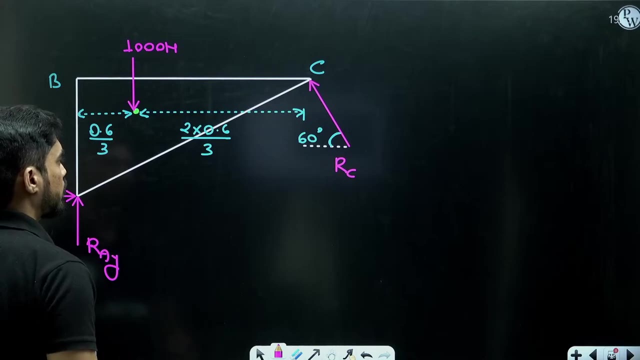 Let us take moment at A and calculate R c. Let us take moment at A and calculate R c. Now, if I take moment at A moment of Ra x and Ra y will be gone. Moment of Ra x and Ra y will be gone. 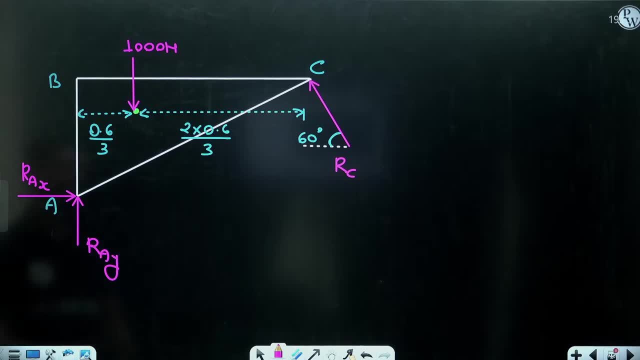 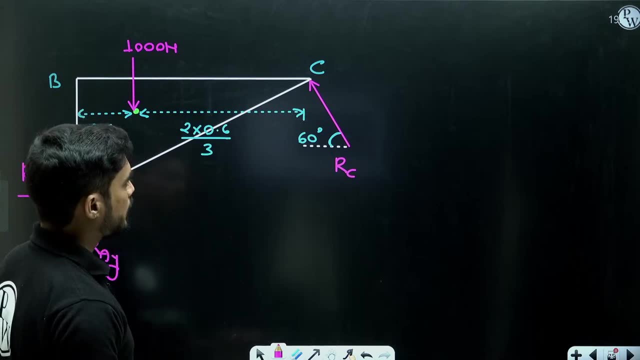 I will have to calculate the moment of R c. So I will have to calculate the moment of R c. So the moment of R c is here and this 1000 Newton. Now R c is inclined. So what you can do is you can resolve R c into two components. 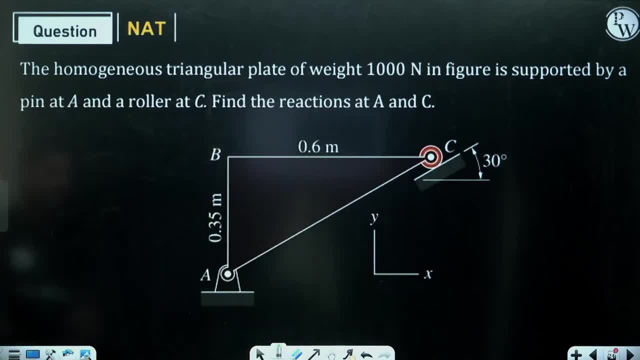 You can resolve R c into two components, or what you can do is let us calculate this. This angle is 30 degrees. almost 30 degree means this R c is inclined and this 1000 Newton is inclined. It means that, hey, here I am. 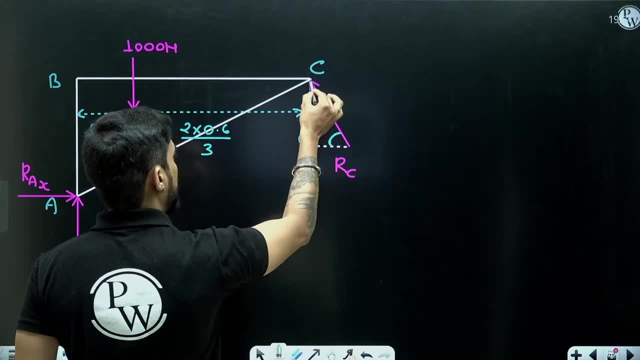 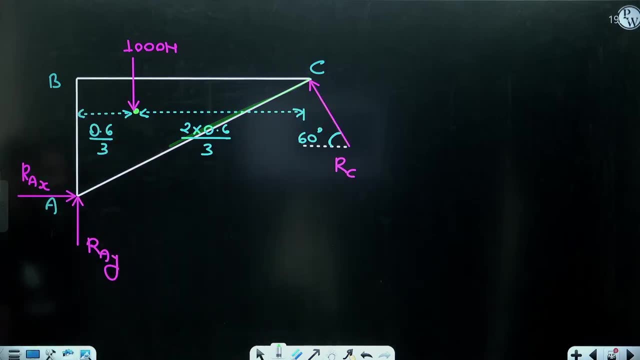 This is the R C. Here you are, So I have to calculate R c. this RC is normal to this surface also. But it will be confusing for you. There will be too many questions. Those who have understood it. let me tell you this: that RC is also normal to this. 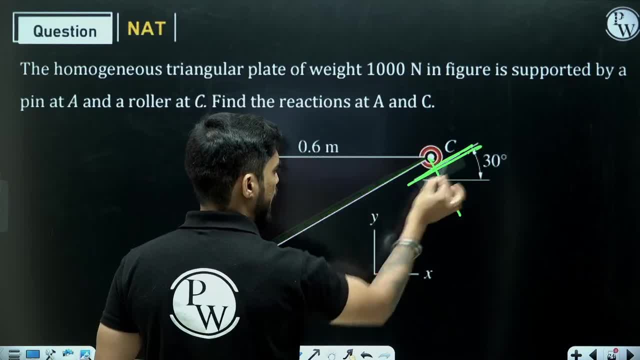 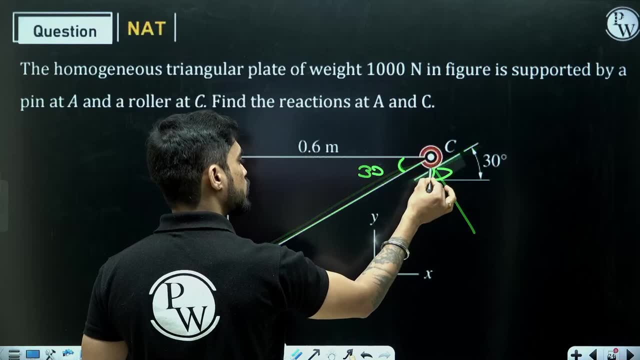 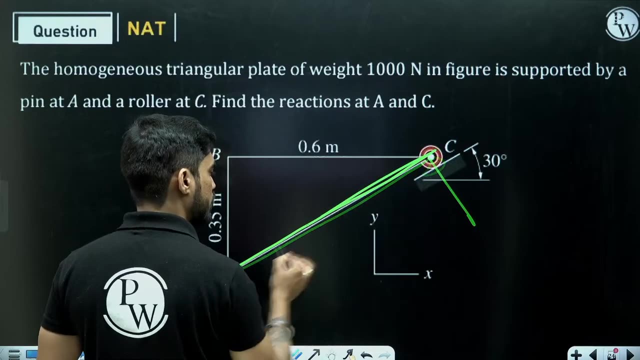 surface. This surface and this surface are parallel to each other, it seems, Because this angle is almost equal to 30 degree, So the reaction is also normal to this surface. So you know the perpendicular distance of RC from A. it will be equal to this distance, So you can directly. 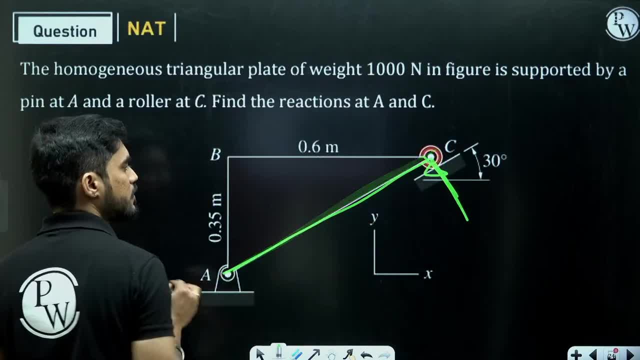 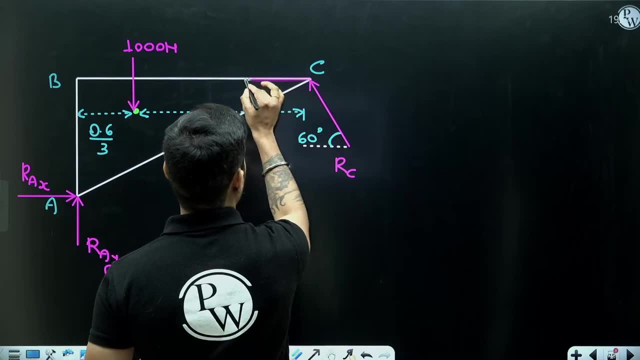 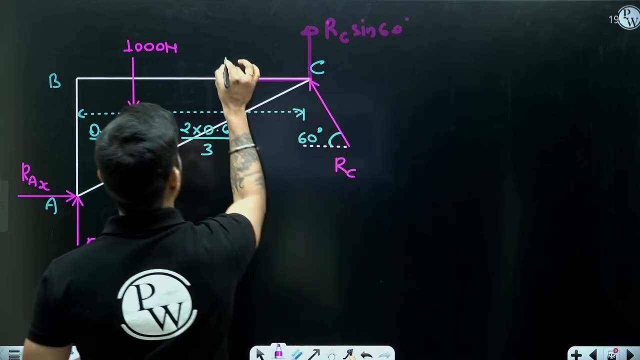 calculate moment of RC: RC multiplied by this distance. But if you are not able to get that, don't worry, Just resolve RC into two components. This will be RC sin 60. This will be RC cos 60.. Right, So now. 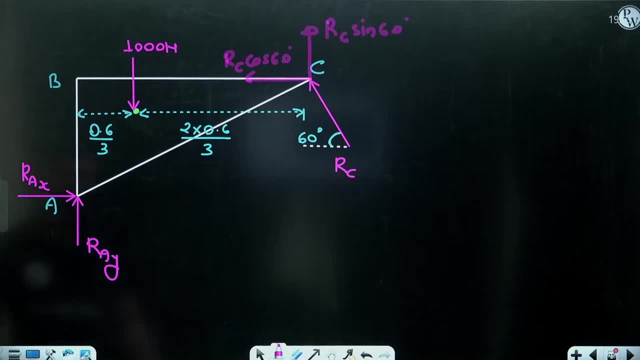 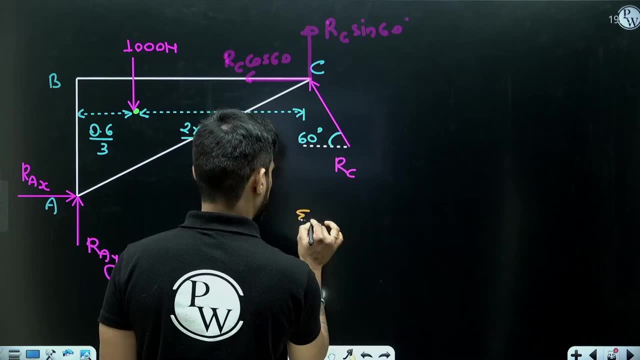 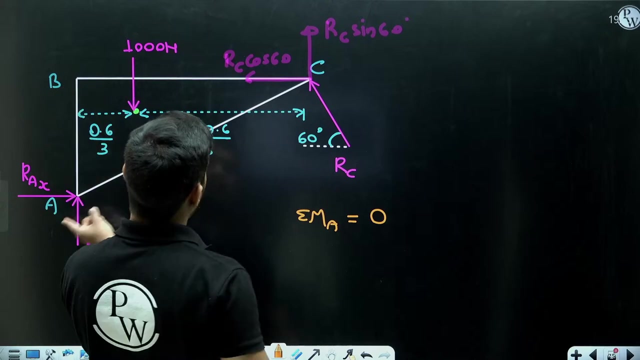 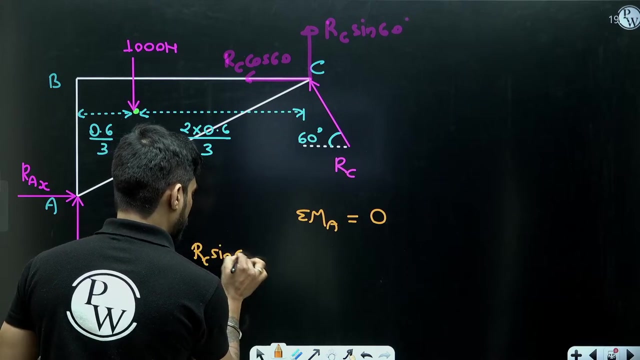 we can take moment at point A, So moment at point A must be 0.. Now moment of RC sin 60 and RC cos 60, both will be anticlockwise at point A. So RC sin 60 multiplied by this distance. How much is this distance? 0.6.. 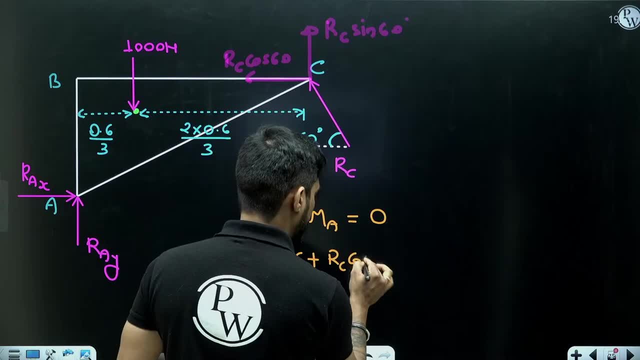 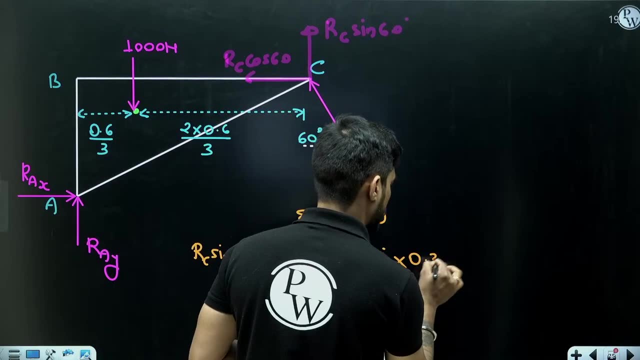 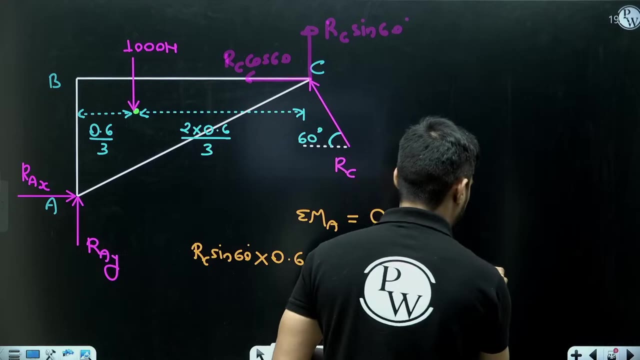 Plus RC cos 60,. multiplied by this distance, How much is this .35?? Both these moments are anticlockwise, But moment of 1000 will be clockwise. So it will be minus 1000 into 0.6 by 3.. well, by 3.. 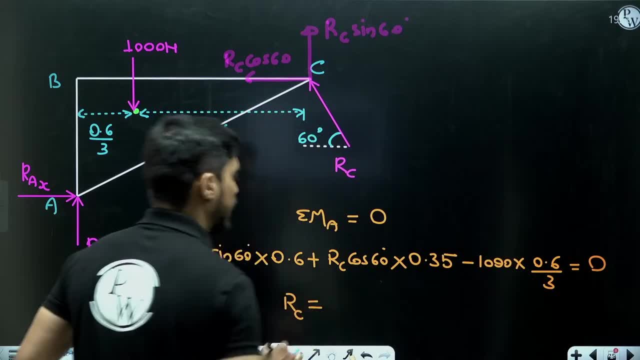 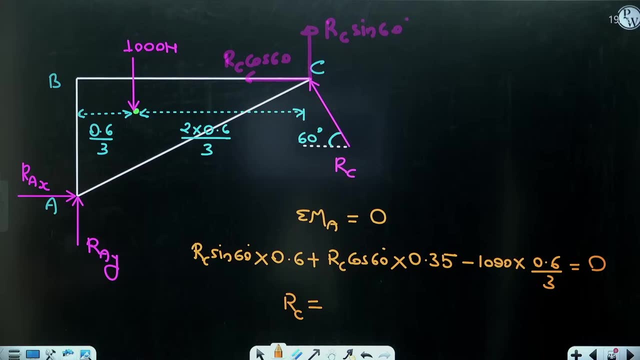 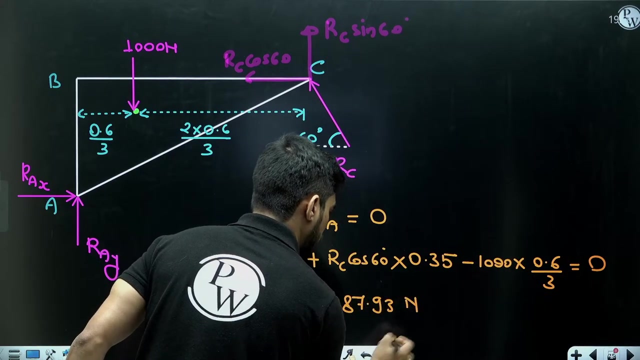 So from here you will get the value of RC. So it will be 200 divided by 0.6 sin 60, plus 0.35 cos 60. I am getting 287.93 Newton. 287.93 Newton. 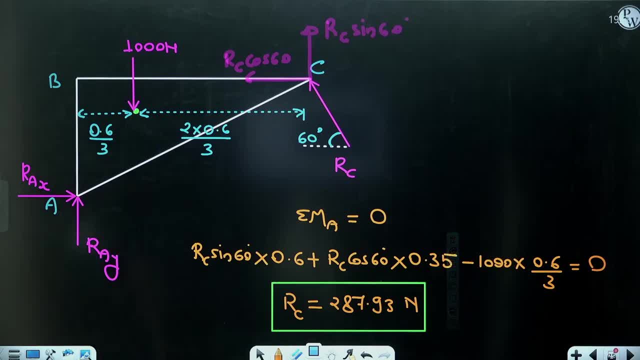 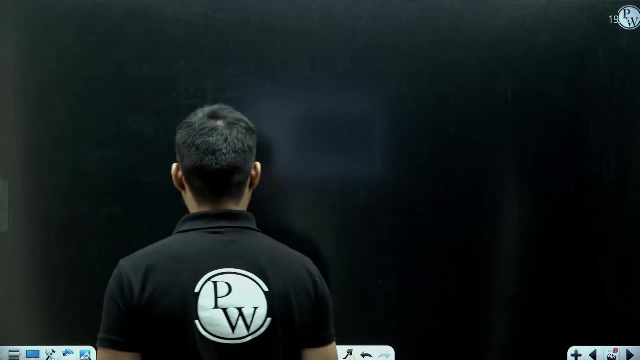 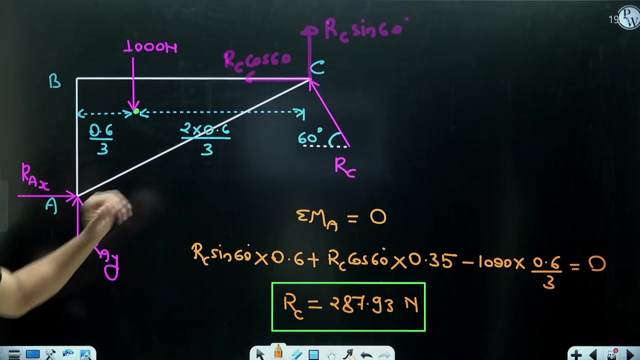 I hope you also are getting the same. So it will be 287.93 Newton. Now we can find out RAx and RAy. So if I apply, summation of Fx equals to 0, RAx is towards right and RC cos 60 is towards left. 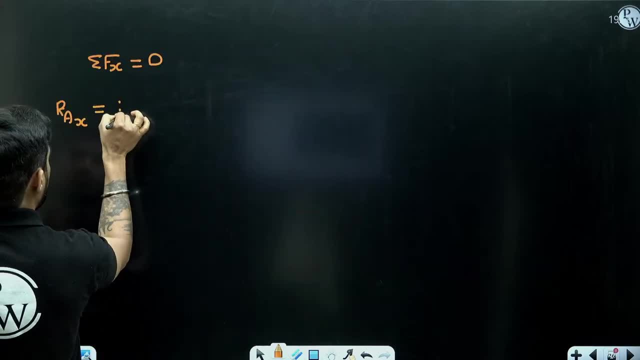 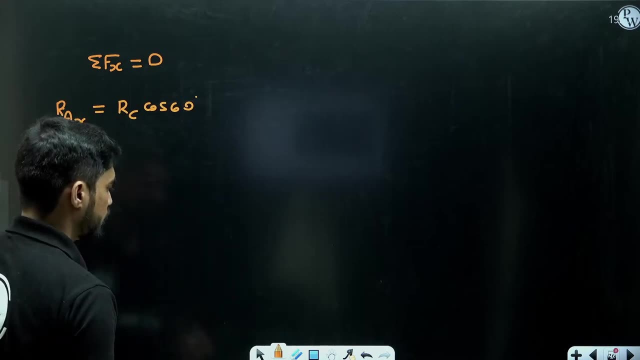 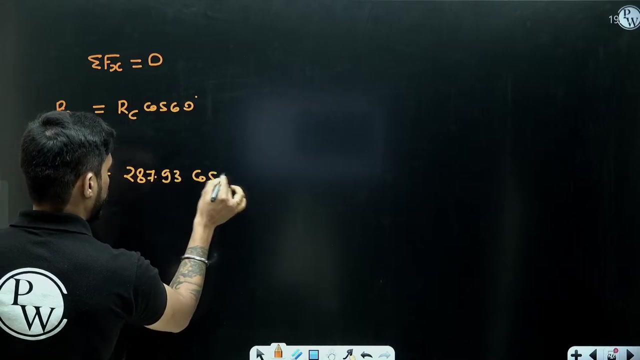 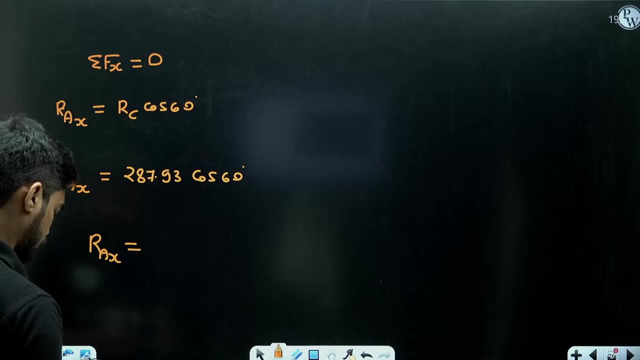 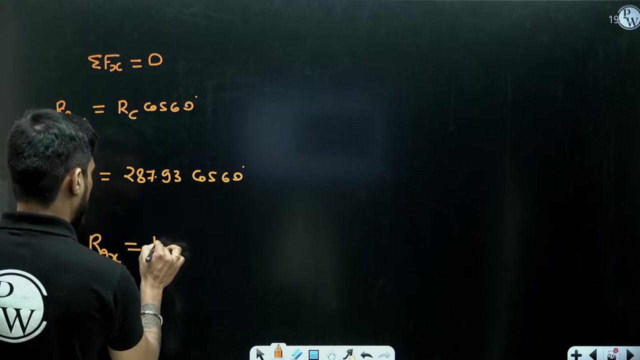 So it will be. RAx equals to RC, So it will be. cos 60 means RAx will be equal to RC. which is how much? 287.93 cos 60.. So RAx will be 143.96.. 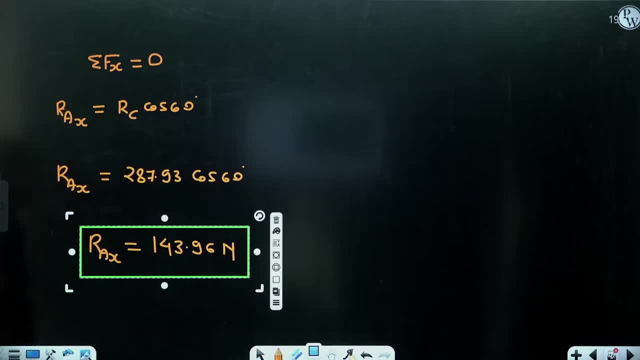 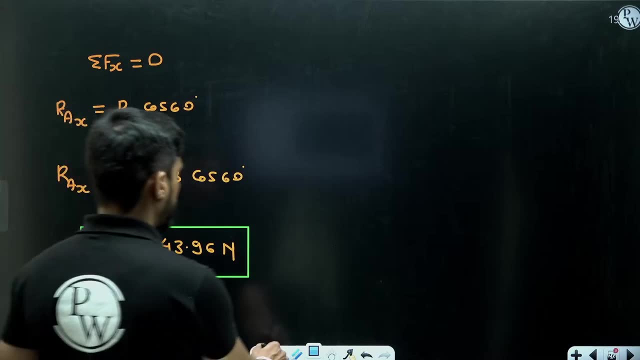 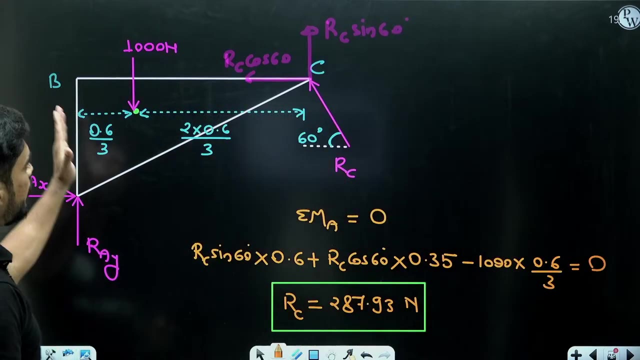 143.96 Newton. Very good, Now summation of Fy equal to 0.. So if I apply summation of Fy equal to 0 in y direction, you have RAy RC, sin 60 and 1000.. 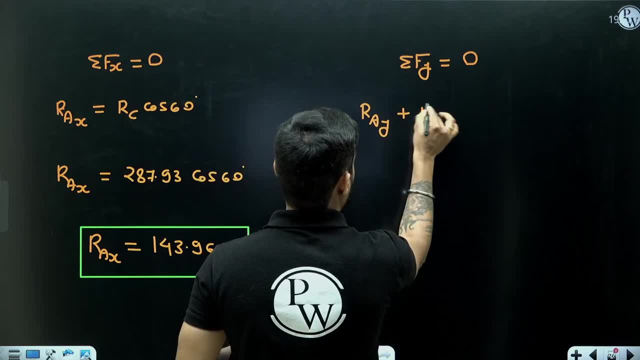 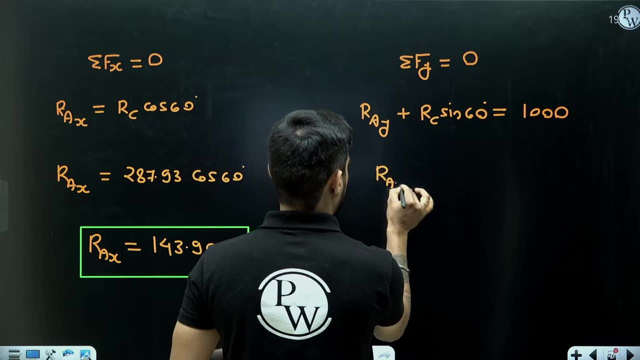 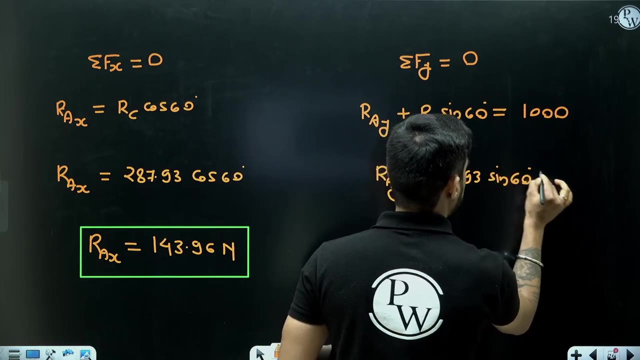 So it will be RAy plus RC, sin 60.. Both are upward and 1000 is downward. So RAy plus 287.93, sin 60, equal to 1000.. So from here you get RAy. 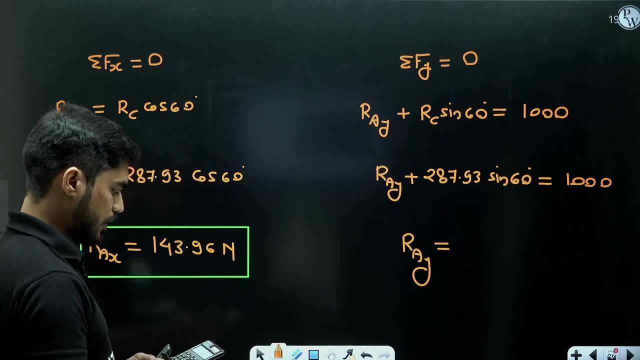 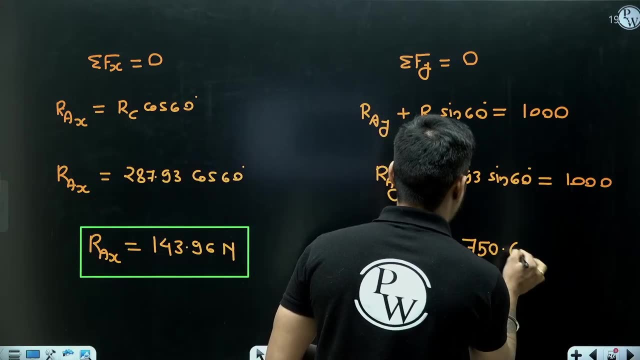 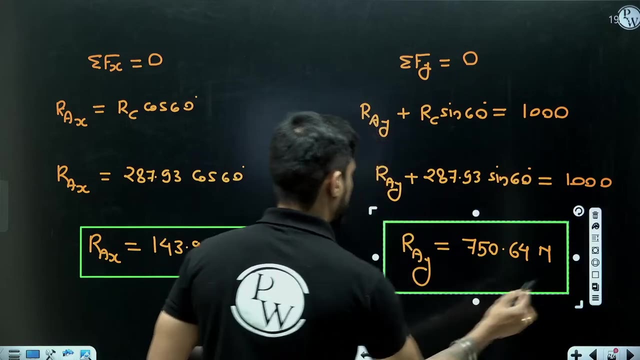 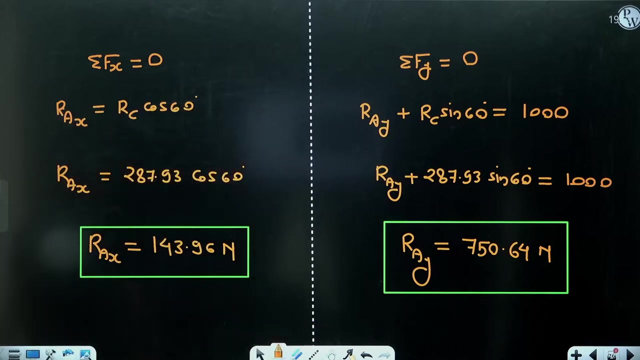 So 1000 minus 287.93 sin 60.. I am getting 750.64.. So I am getting 750.64.. So I am getting 750.64.. 750.64 Newtons, 750.64 Newtons. 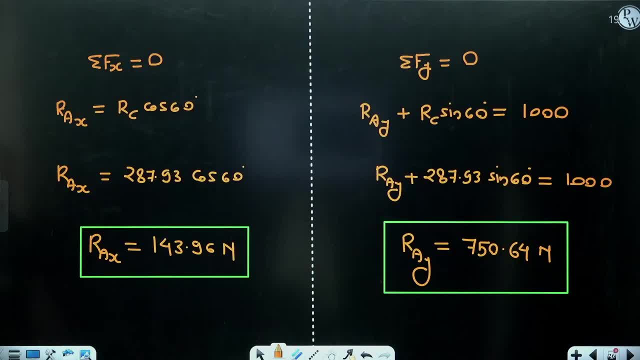 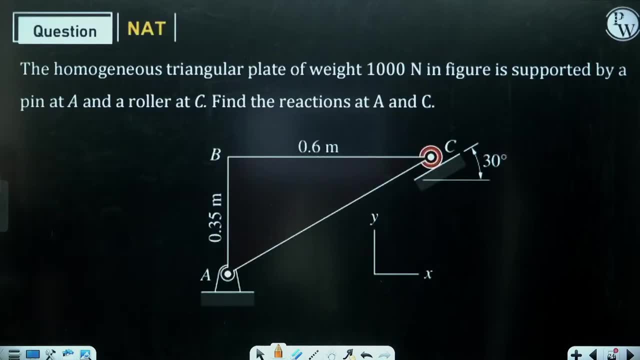 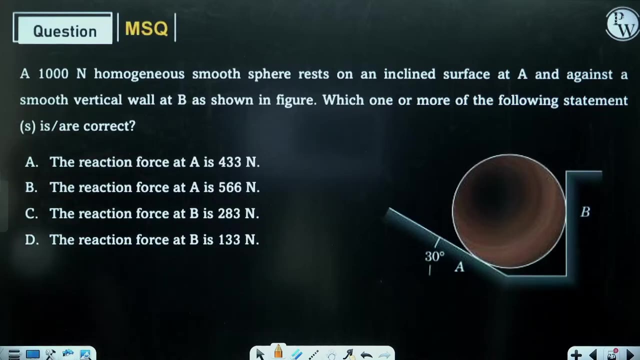 So these are the values of RC, RAX and RAY. I hope this is clear to you. Let's move on to the next question. Now this is an interesting one. This is an MSQ question. What do we mean by MSQ question? 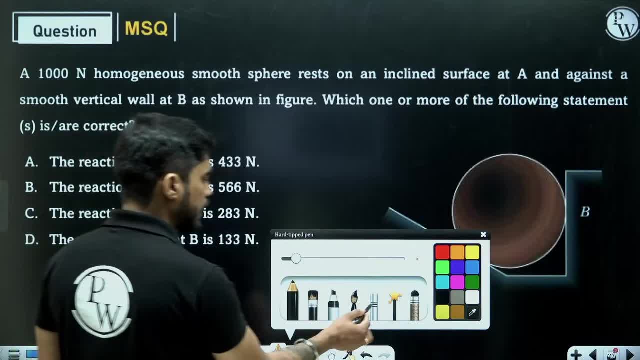 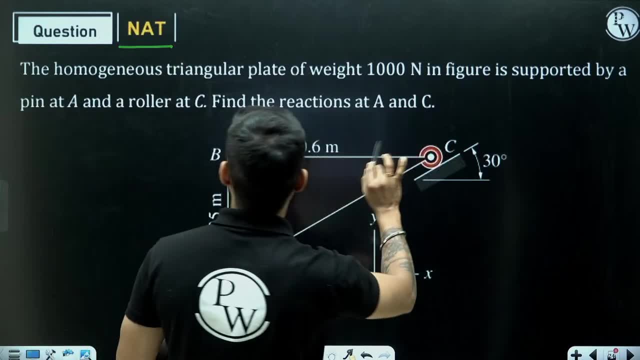 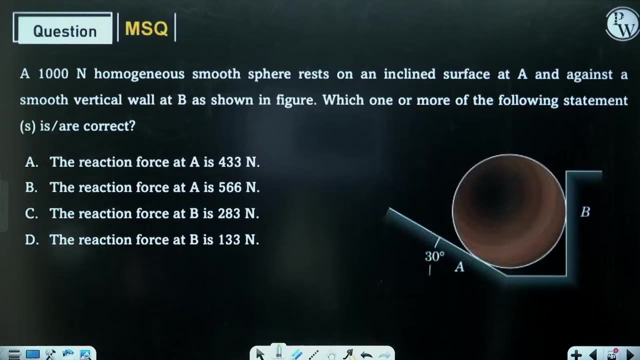 In GATE you have three types of questions: NAT, which is numerical answer type, where you have these blank spaces and you have to fill the answers. Then MCQ, multiple choice question, where you have four options and one of the option is correct. 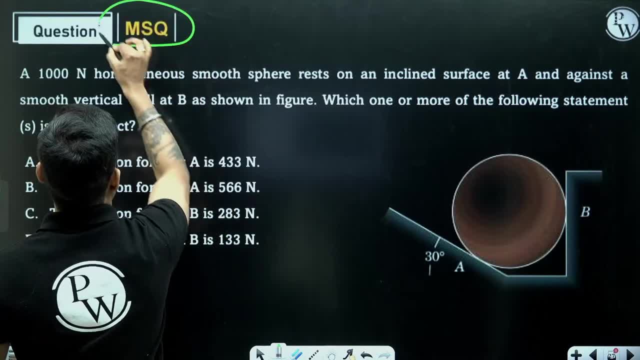 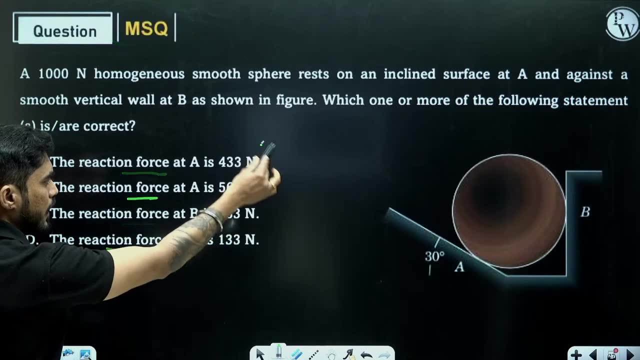 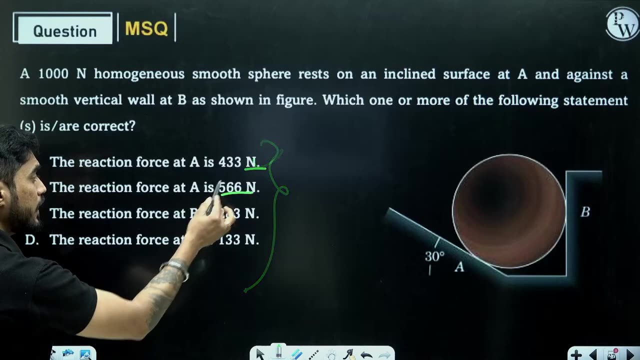 And then MSQ, multiple select question, Where you have multiple options, which can be correct. Four options are there, So maybe there is only one correct answer, Maybe there are two correct answers, Maybe there are three correct answers, Maybe there are four correct answers. 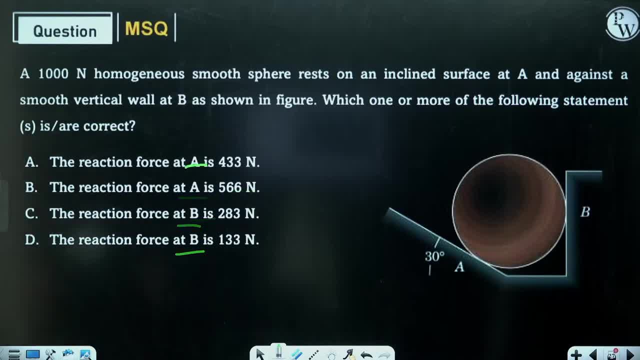 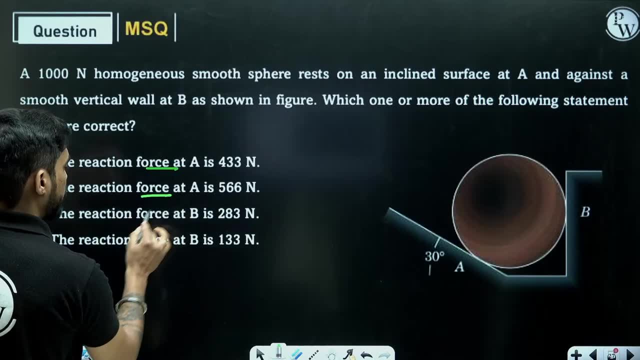 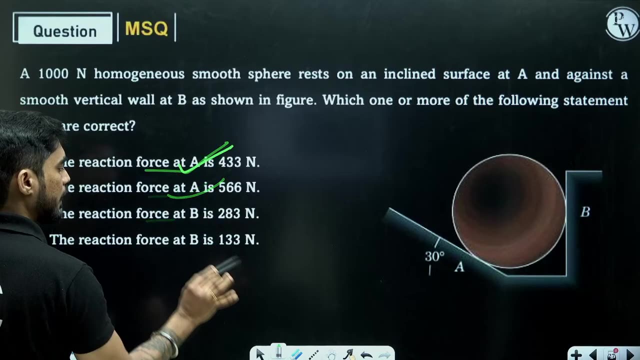 But here is a catch In these type of questions. let's say there are three correct answers, but you have given only one or two. There are three, but you have given only one or two. You will not get any marks, you will get zero marks. 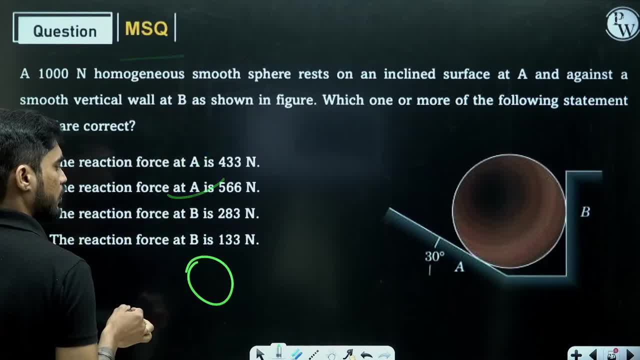 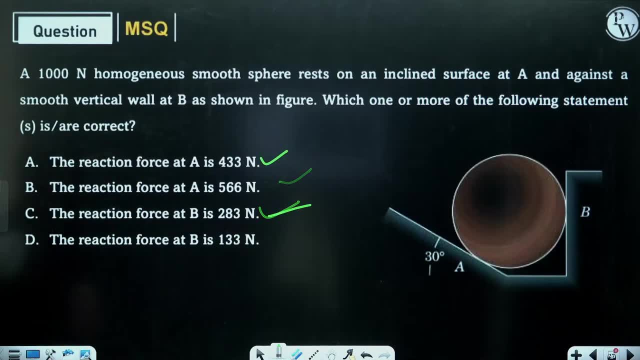 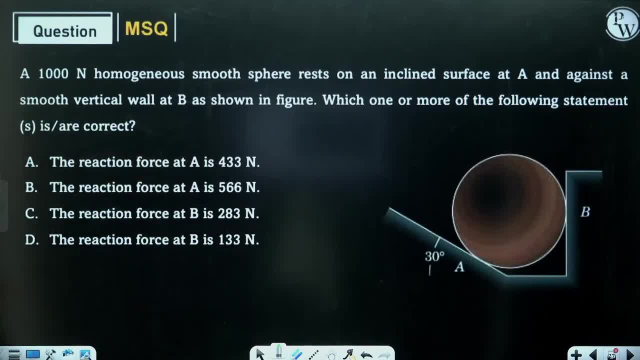 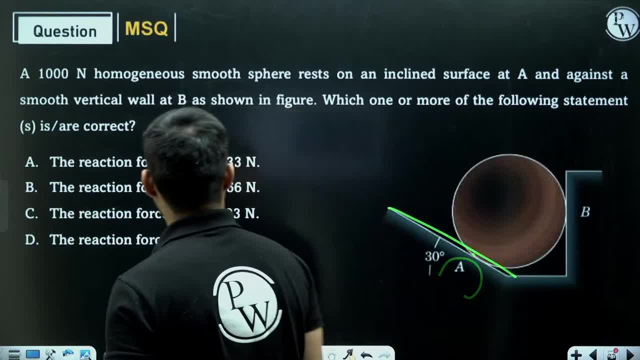 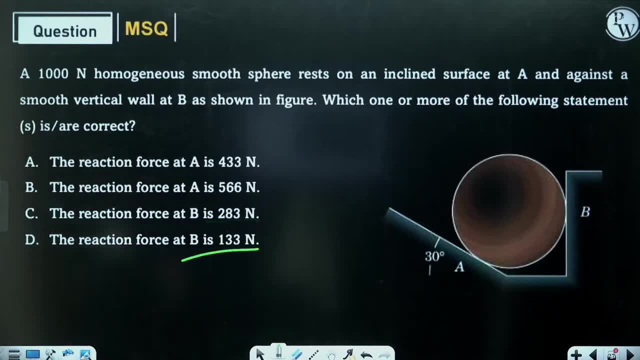 Reaction at A is 566 Newton, Reaction at B is 283 Newton And reaction at B is 133 Newton. So basically, you need to calculate reaction at A and reaction at B. So how are we going to solve this problem? 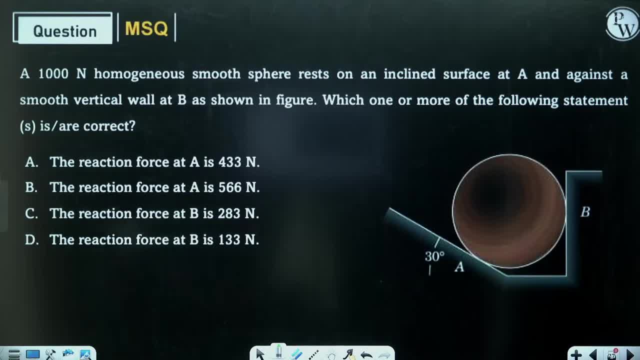 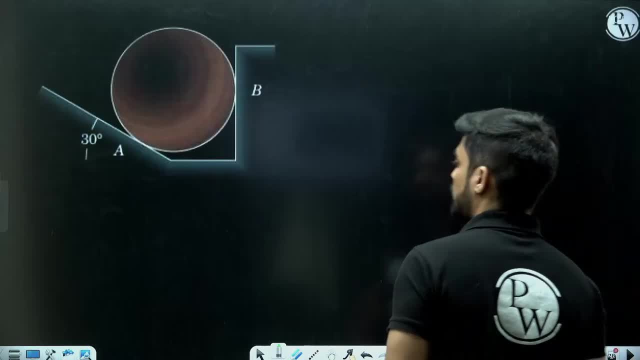 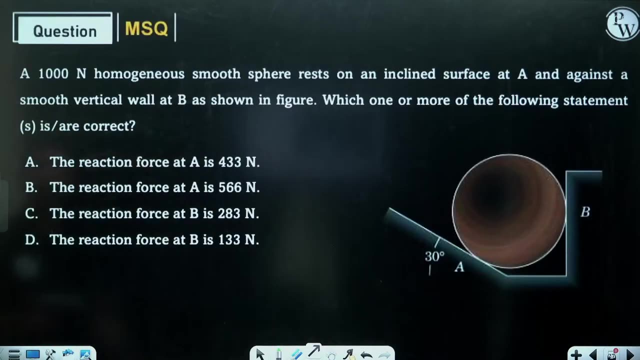 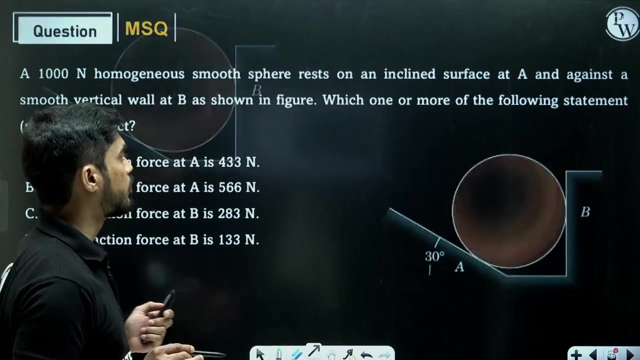 First you need to apply- sorry, draw- the free body diagram. Okay, You need to draw the free body diagram. So here this sphere. it has a weight of 1000 Newton and it is homogeneous. Homogeneous means the weight is equally distributed. 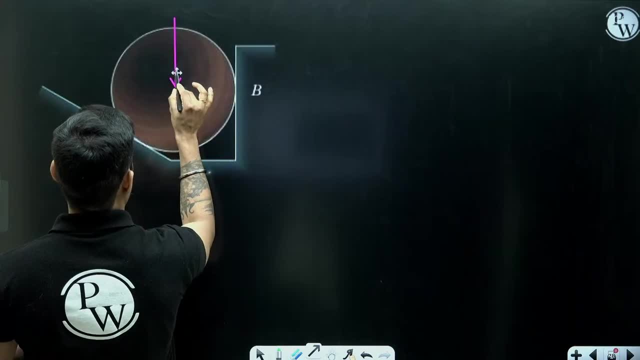 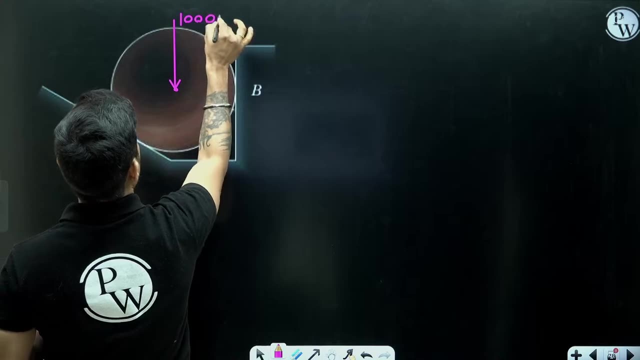 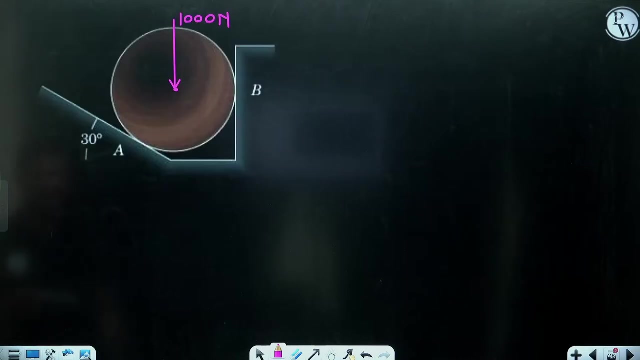 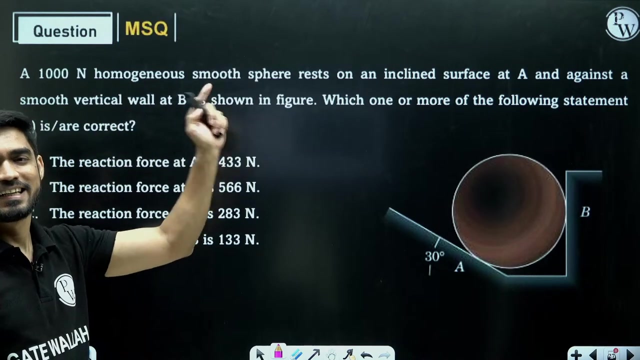 So the weight will be acting at the centroid. Centroid of the sphere will be at the center. Okay, So this is 1000 Newton. Now, at point A and B we have frictionless surfaces. Okay, Smooth surface means frictionless surfaces. 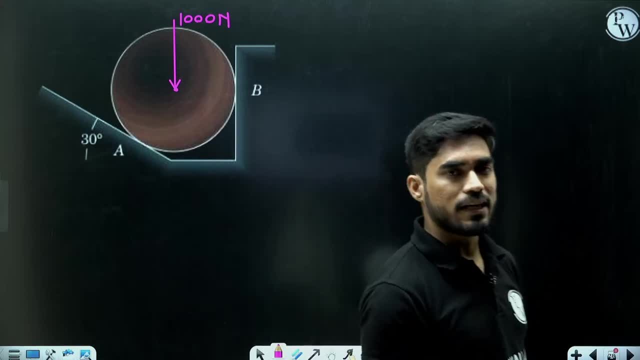 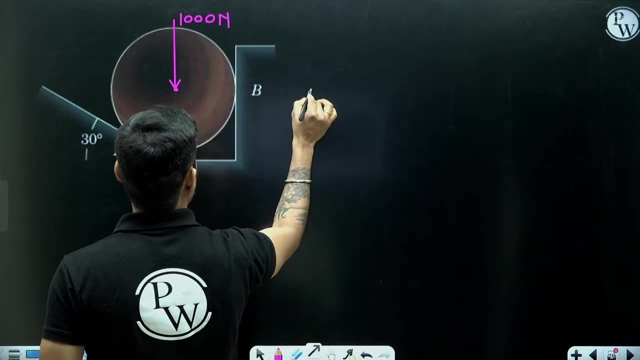 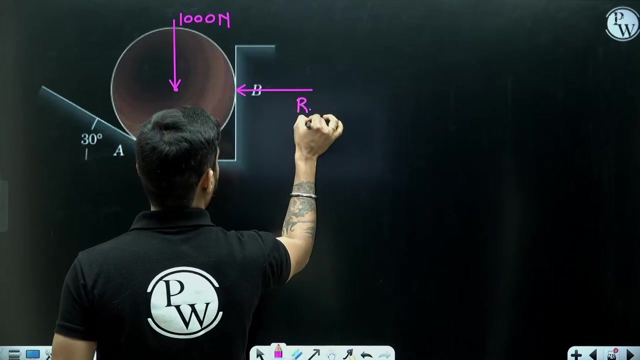 And in case of frictionless surfaces you get the reaction Normal to the surface. So at point B the surface is vertical, So the reaction will be horizontal, So it will be RB. Similarly, at point A the surface is inclined. 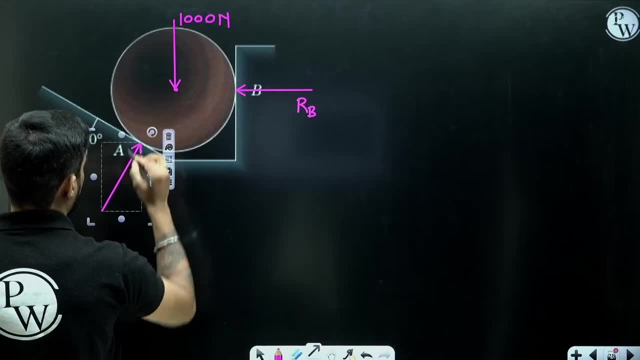 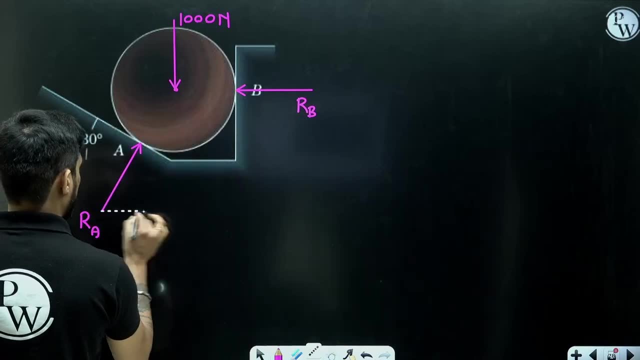 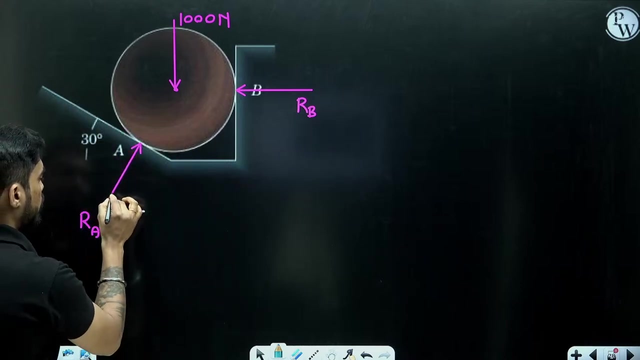 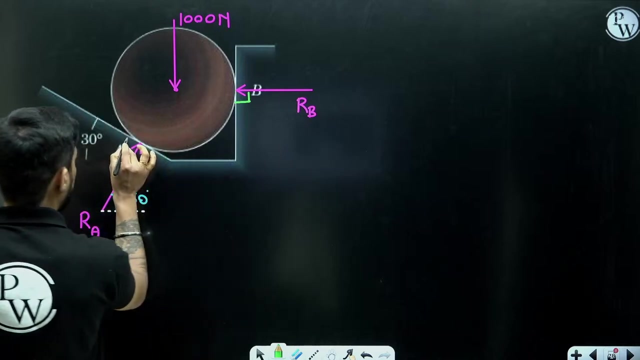 So reaction will also be inclined. How, What will be the angle? The angle will be, see, the surface is making 30 with horizontal, So the normal of surface will make 60 with horizontal. Okay, This angle is normal 90 degree. 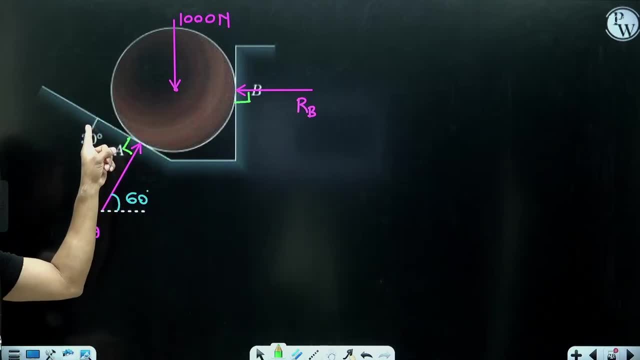 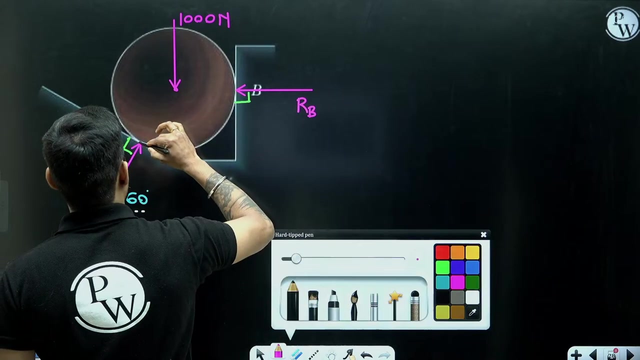 This angle is 90 degree, So the surface is making 30 with horizontal, The reaction will make 60 with horizontal. Okay, Now, how many forces do we have? We have three forces, So these three must be either parallel or concurrent. 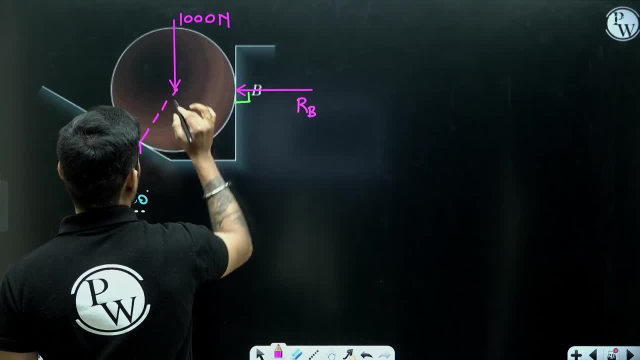 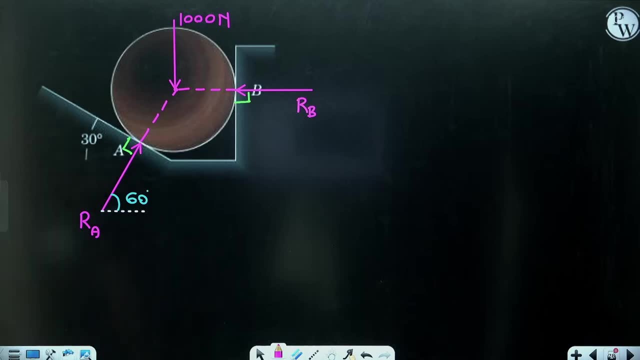 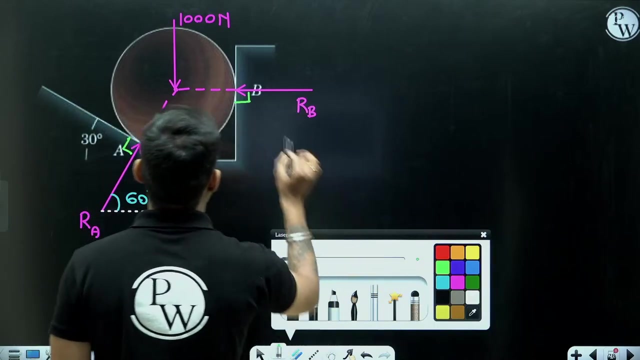 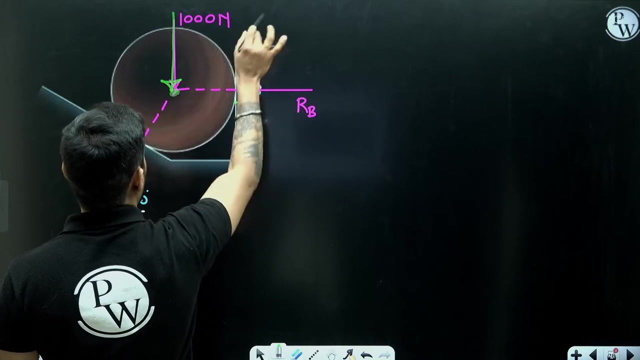 They don't seem parallel, It means they must be concurrent, Okay, And in this case you can apply Lamy's theorem. You can apply Lamy's theorem. Okay, Now either all three forces must be acting towards the center or away from the center. 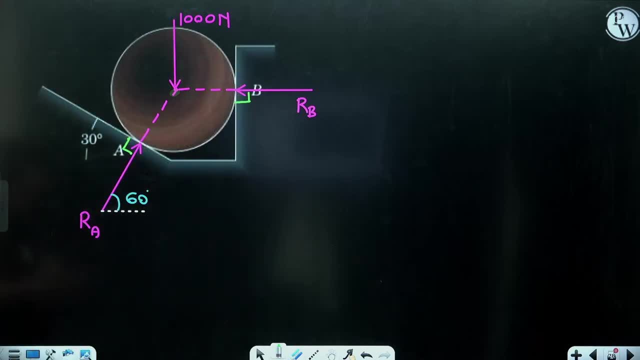 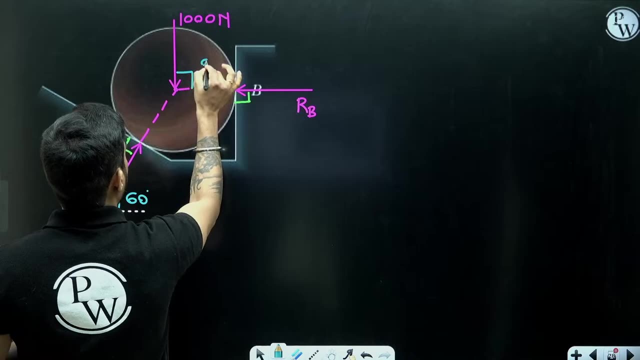 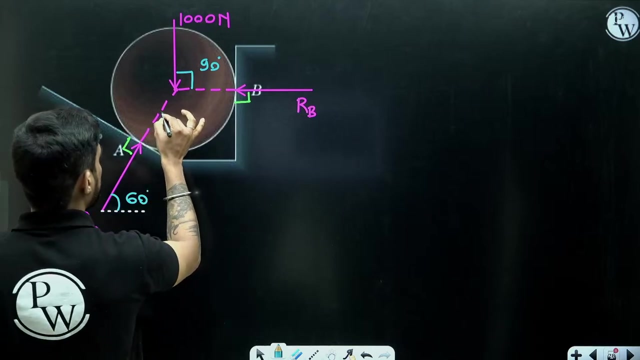 So here all three forces are acting towards the center. So I can calculate the angles from this diagram. What will be this angle? It will be 90 degree Right. What will be this angle? What will be this angle? See, 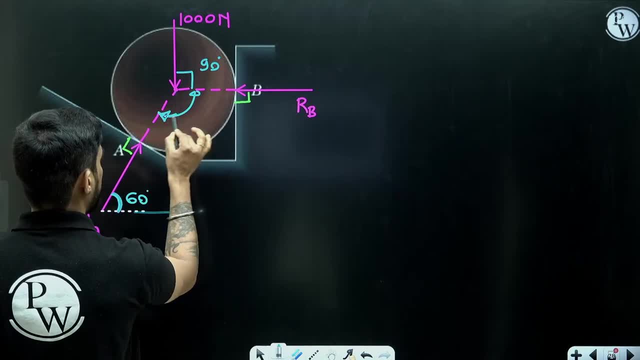 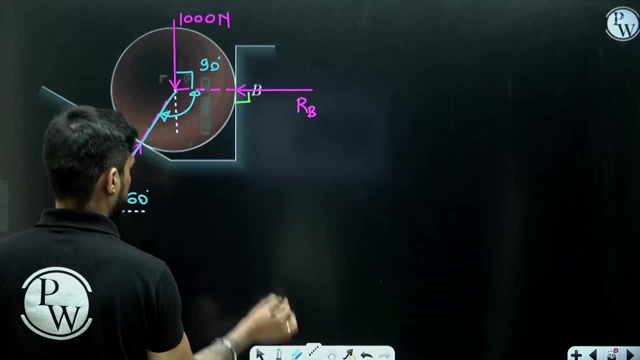 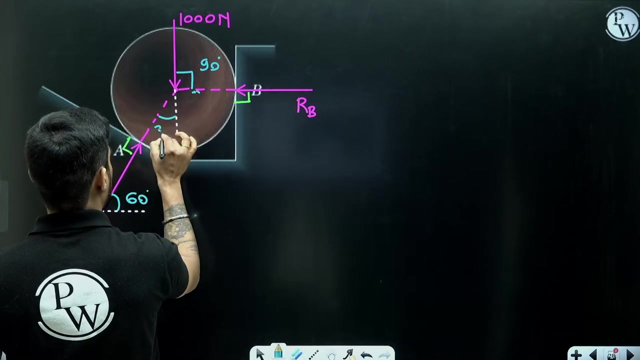 This is 90.. This is 60. So this is 30. Right, Let me draw this And let me divide the angle into 2.. This is 30. And this is 90. So the total angle is 120.. 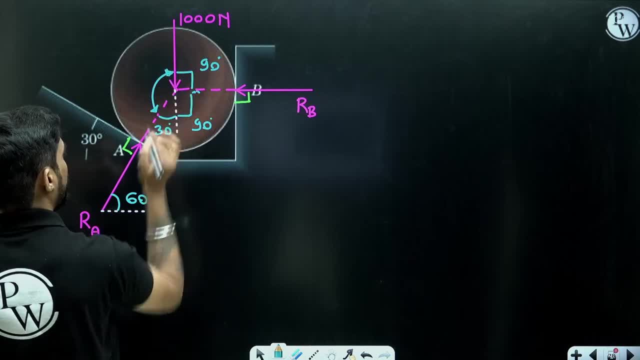 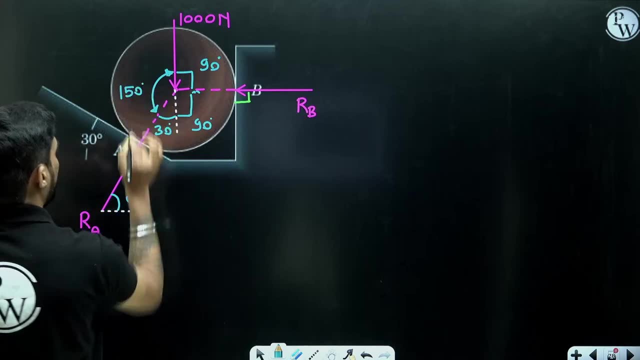 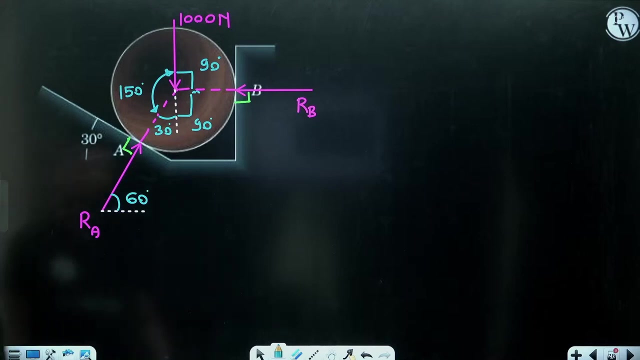 Okay, Now, what will be this angle? Now you can easily calculate this: 90, 90, 180.. 180 plus 30, 210.. This will be 150.. Okay, Now I can apply Lamy's theorem. 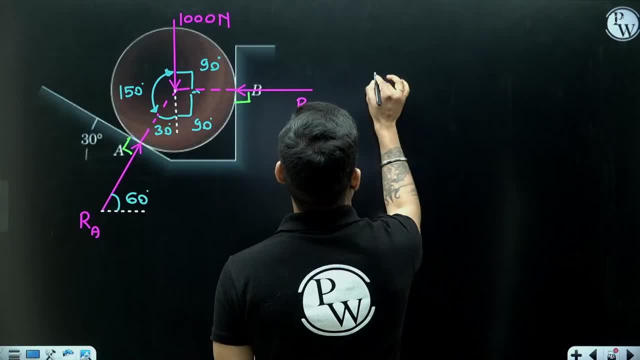 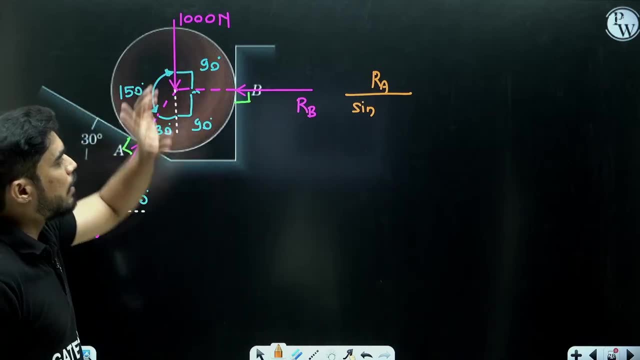 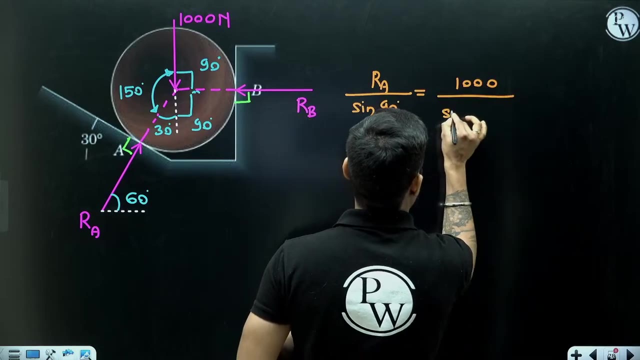 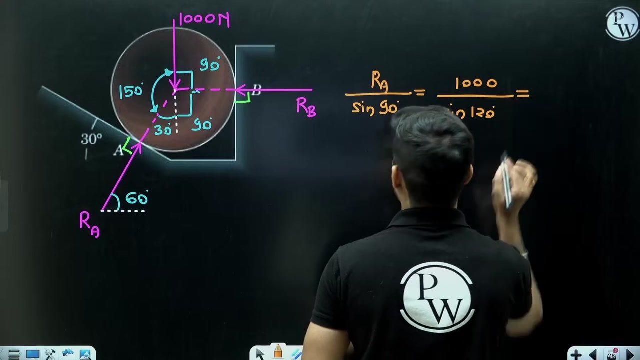 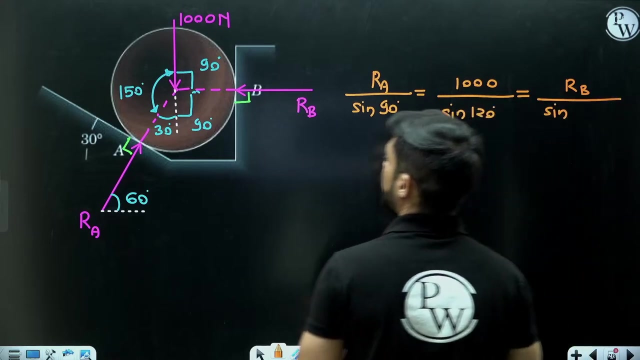 So, according to Lamy's theorem, Ra divided by sin of angle between Rb and 1000 is 90- equals to 1000. divided by sin of angle between Ra and Rb is 120, equal to Rb. divided by sin of angle between 1000 and Ra is 150.. 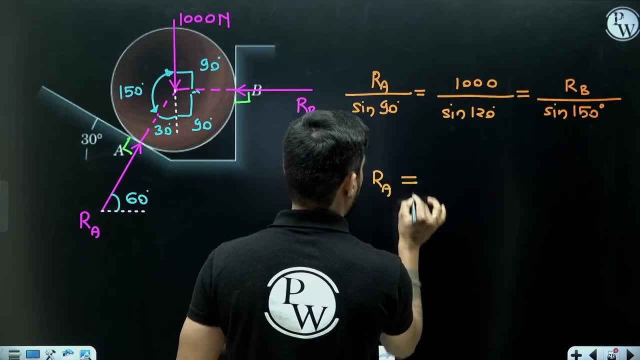 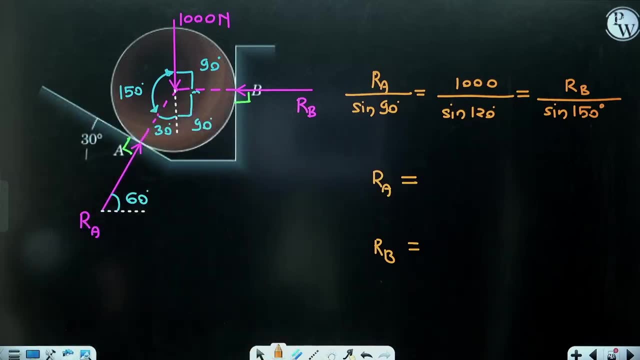 So from here I can find the value of Ra as well as Rb. What will be Ra 1000 into sin 90 divided by sin 120.. Sin 90 is 1.. So it will be 1000 divided by sin 120.. 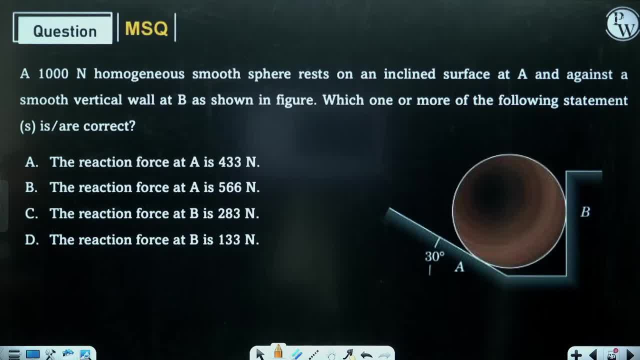 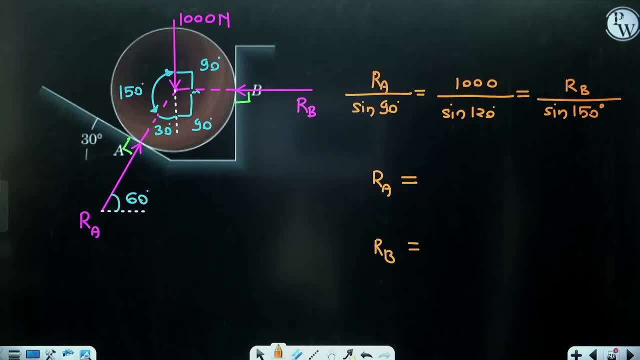 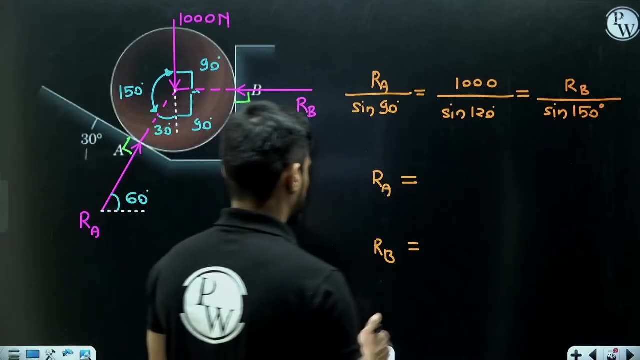 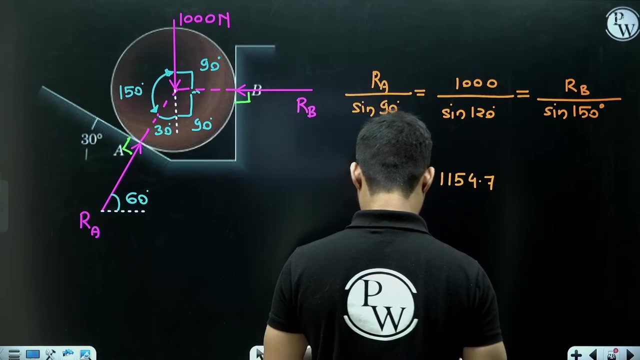 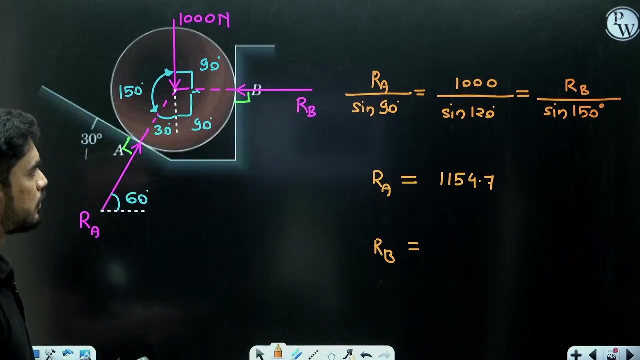 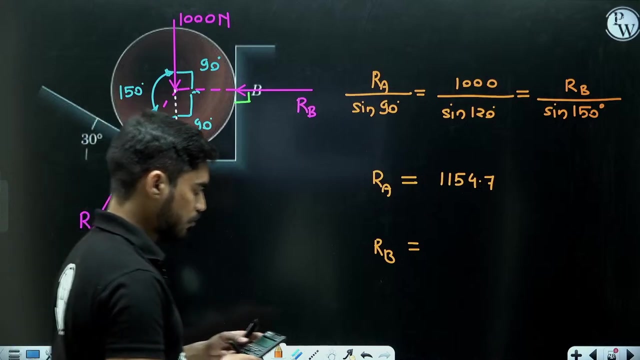 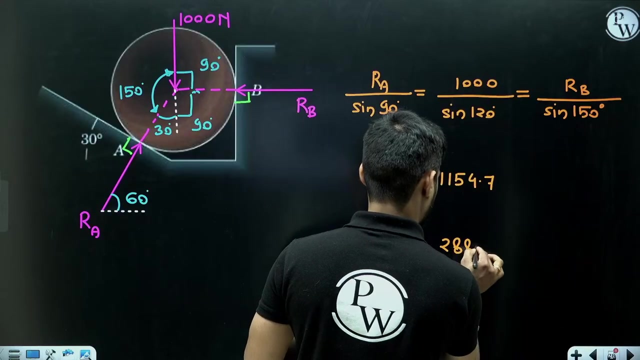 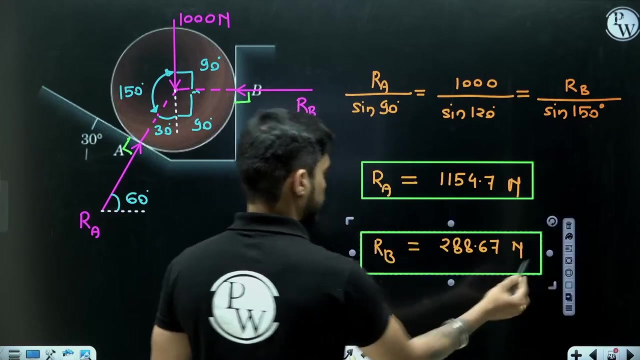 Am I correct? Yes, So here I am getting 1154.7.. Are you also getting this 1154.7?? 288.67.. Okay, Okay, So I am getting these answers. It means none of the options are correct. 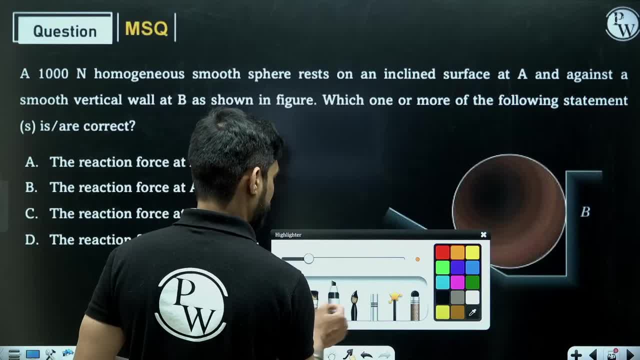 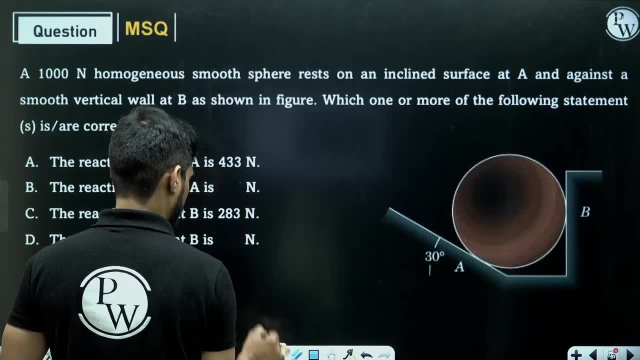 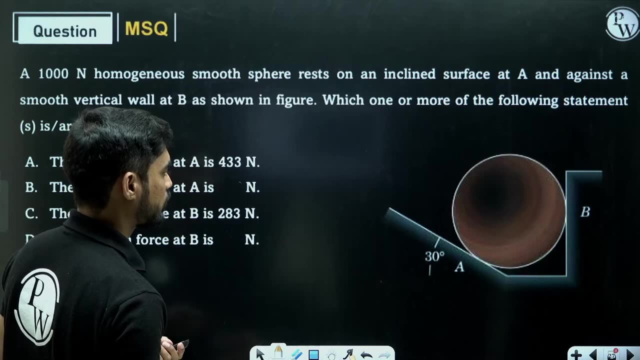 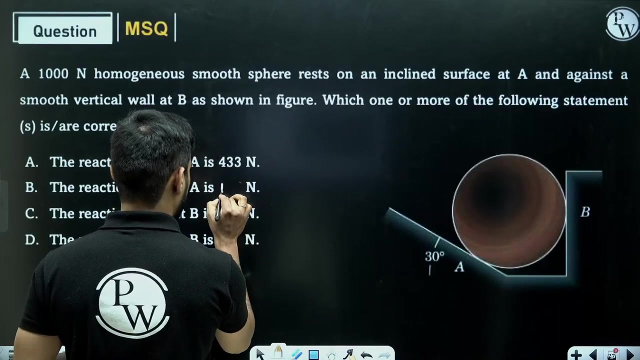 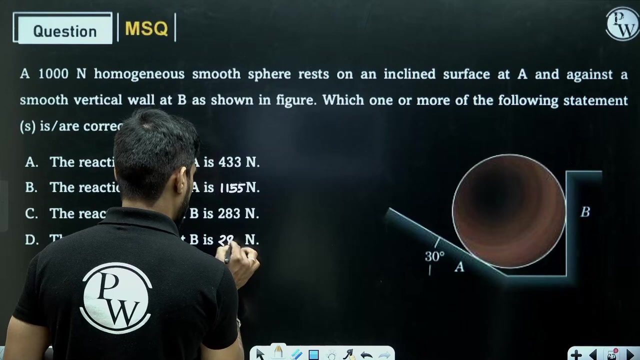 Let's change the options. Okay, Let's change the options. So Ra is 1154.7.. Let me make it 1155.. And Rb is 288.. So let me make it 289.. Okay, So now B and D are correct. 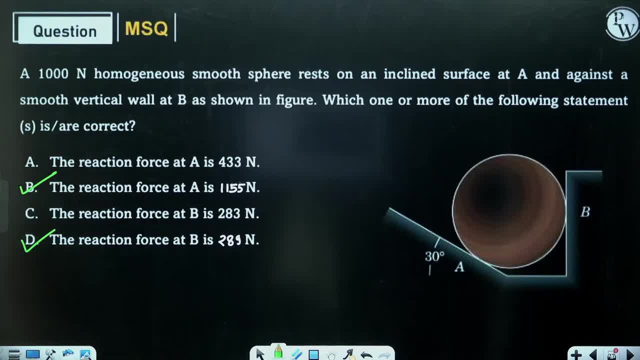 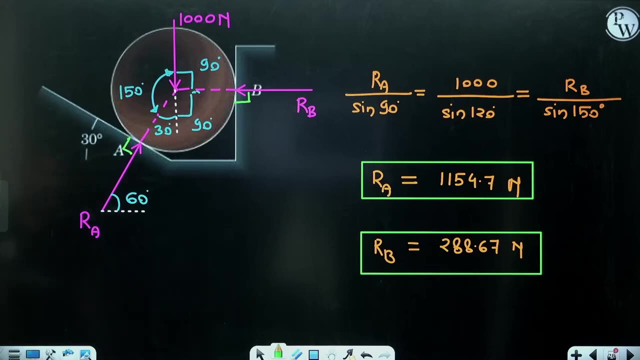 Okay, So there was some mistake with the question, but I have corrected the mistake 1155, 289.. So I hope this is clear. Let me check again if I am getting the correct thing. There must be some value, which was wrong. 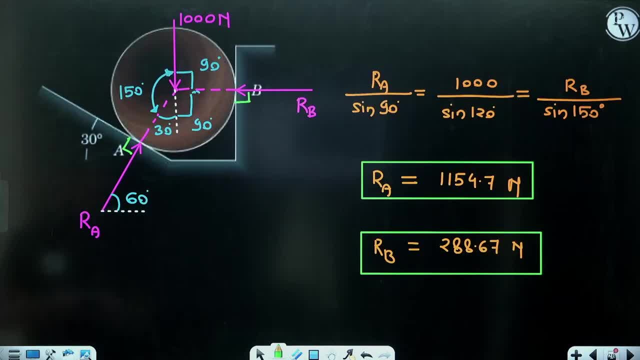 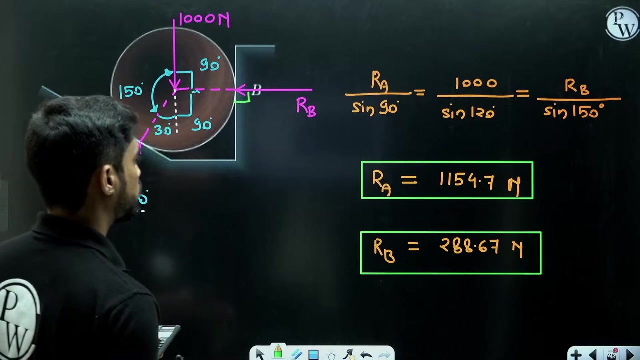 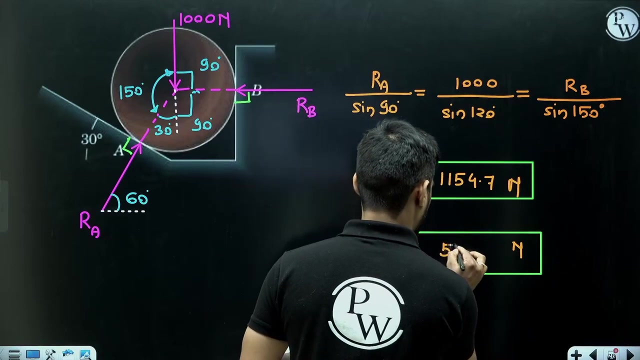 That's why we are not getting the correct answer. So I have changed the question itself. Let me check. Since we have the correct answer, I can populate at this time. This is the problem, Okay, Okay, So I was not getting it.